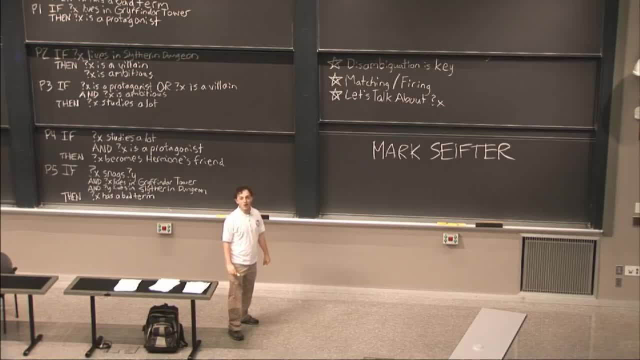 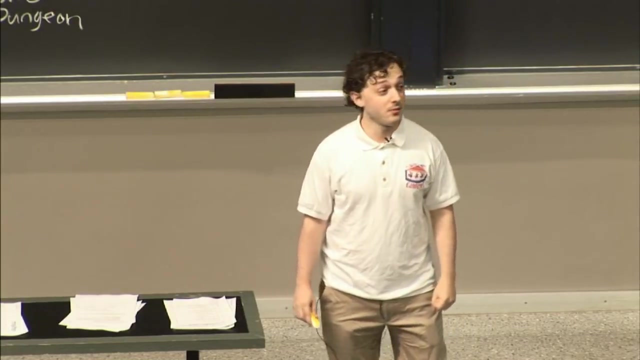 All right. so what is Mega Recitation? Mega Recitation is in this lecture stall room, but I hope to make it more like a recitation or a tutorial by- unfortunately for some of you- perhaps calling on you guys To participate during the Mega Recitation as we attempt to work with some of the material that Patrick has sort of given us the big picture for in the lectures. 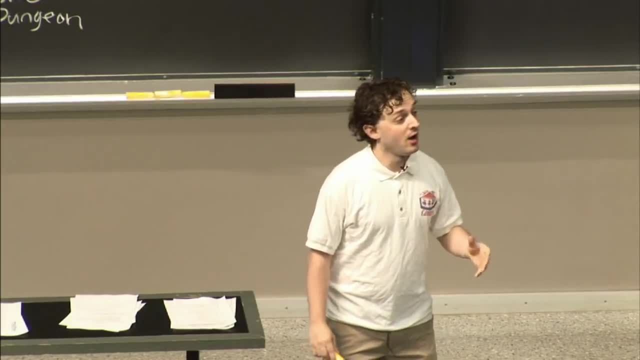 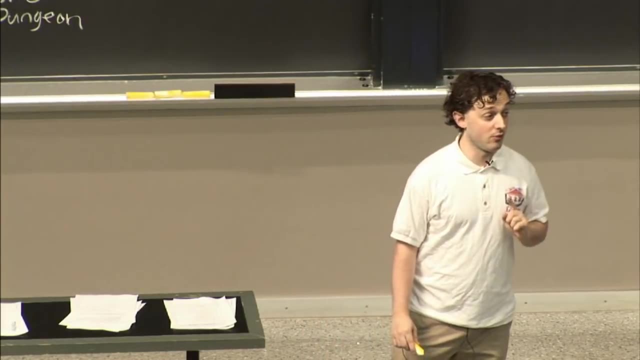 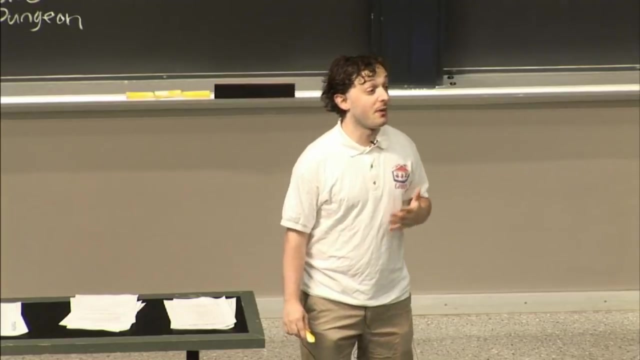 And if you've gone to recitation so far, you may have received a little bit of enrichment into how the algorithms work. Well, here in Mega Recitation we're going to figure out how you can work the algorithms, and that's very important because in this class- being able to work the algorithms by hand- 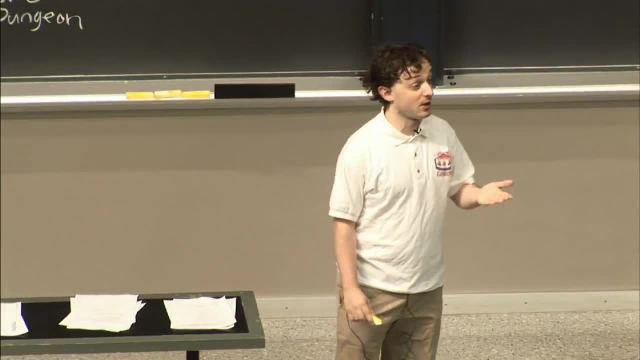 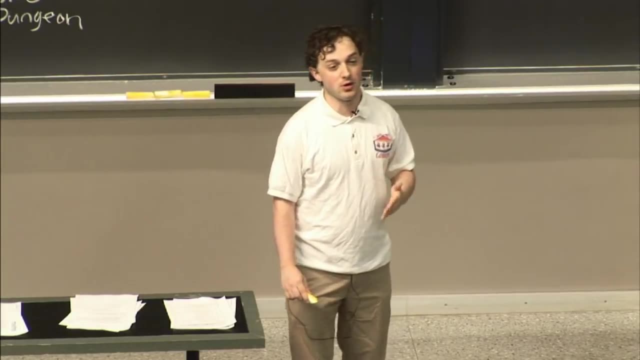 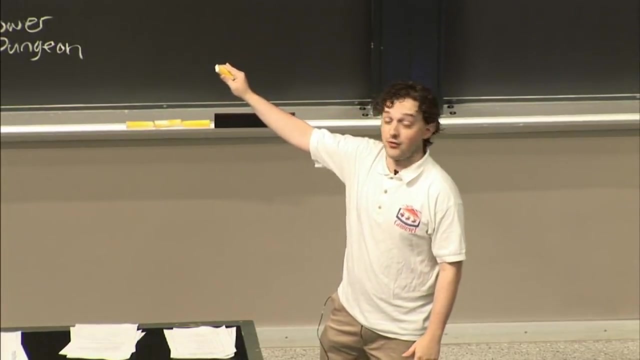 In some of these examples I put up here, or like Patrick sometimes does, in lectures, to teach you the algorithms is a crucial way of demonstrating that you understand how the algorithms work, and we use it on a quiz. The way we use it on the quiz is we? well, this is an old quiz problem. It's from last year. It tripped up a lot of people, so we're going to go over it today. 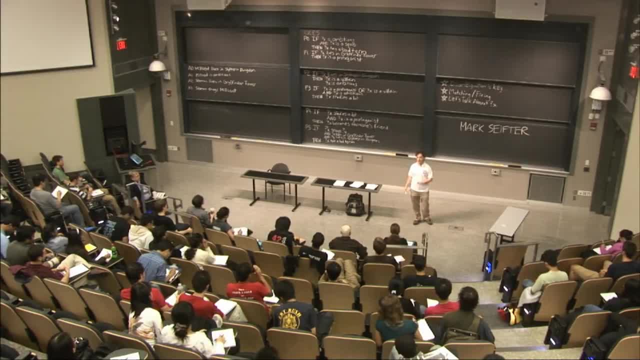 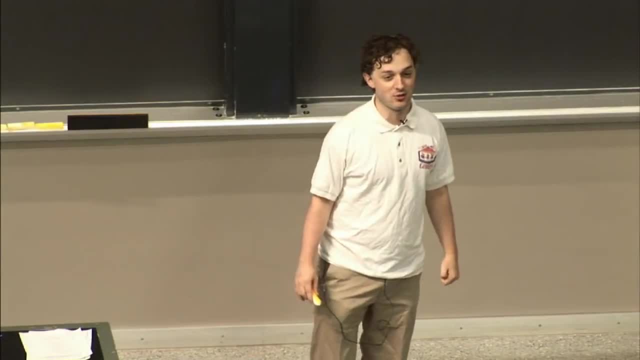 I'm going to tell you all the tricks that tripped up a lot of people, In addition to emphasizing tricks that I've picked up over the Gosh- it hasn't been three years of teeing this course before- so that you will not fall prey to any of these tricks, hopefully. 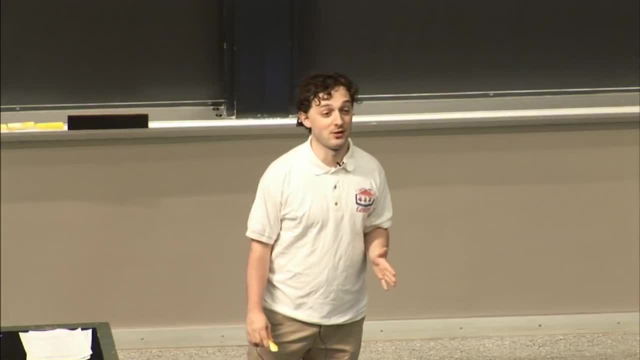 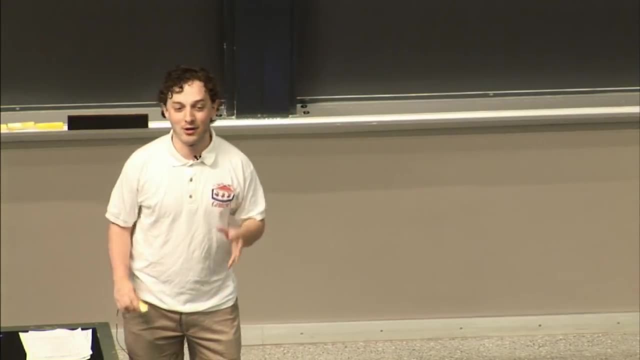 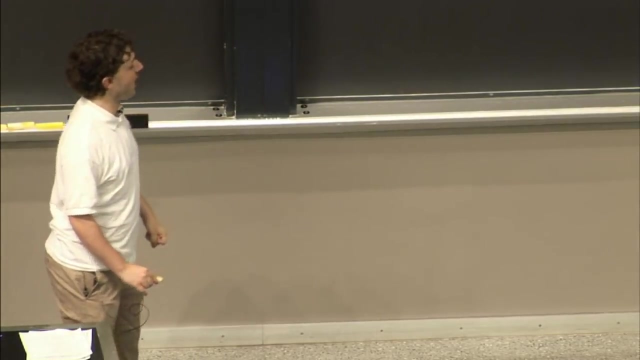 I say hopefully, because some of these tricks I talked about at Mega Recitation last year and people still got tricked by them. I guess maybe some people didn't come to Mega Recitation or they were just very tricky tricks. So be sure to come to Mega Recitation. Pay attention to the tricks, Pay attention to how these things are solved. 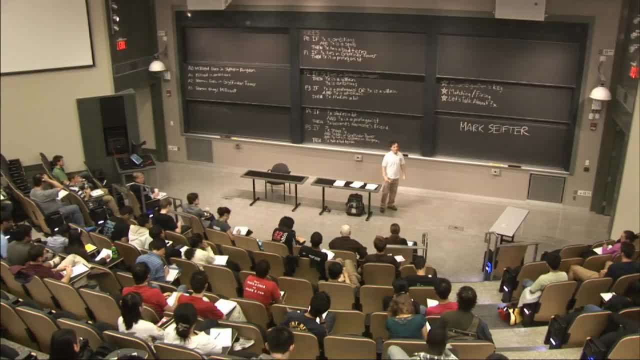 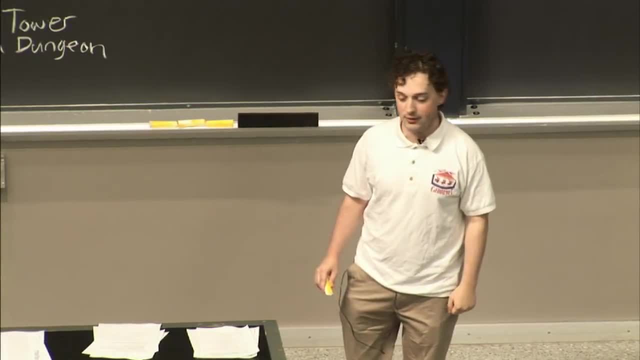 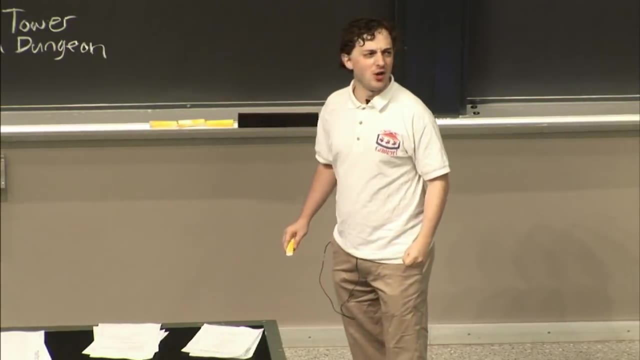 Ask questions if you're not not sure and when we get done with the hour together, I'm hoping that everyone's going to do really well on the rules part of the first quiz. So, without further ado, if there are no questions on that- which I don't think there probably will be- let's move on to the problem at hand. 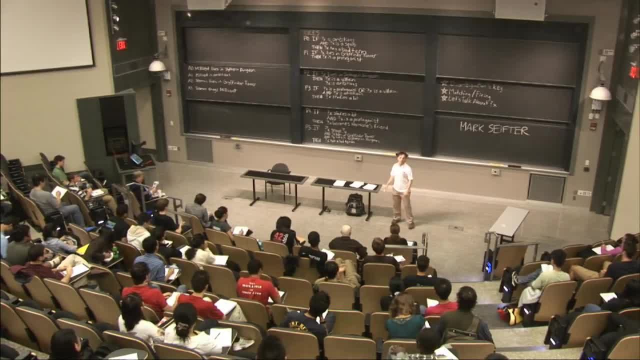 As some of you may have noticed, it is a Harry Potter-based problem. One of our TAs last year was a big Harry Potter fan, So what we have here are There are a series of rules and a series of assertions. 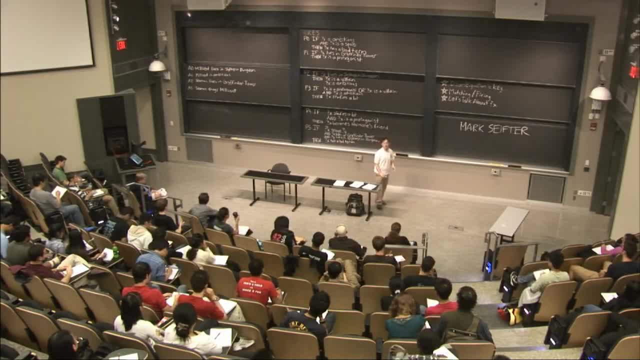 Now, if you happen to be a real go-getter and have already looked at all the past quizzes online- and you may have already seen this problem- and if you really really have attention to detail, you may notice something a little bit different in the way I wrote it as compared to the way it was written online. 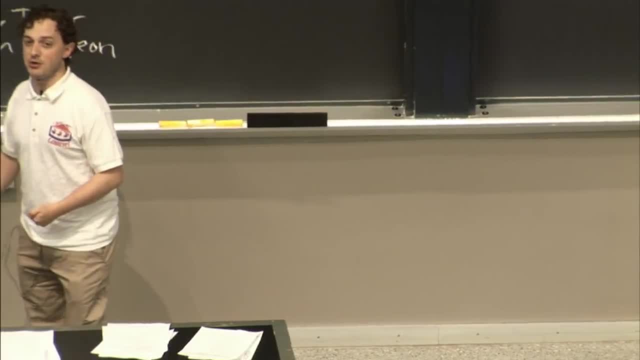 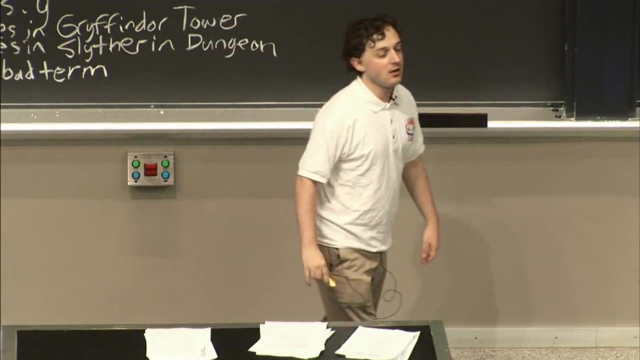 In fact you may if you have a lot of attention to detail, but you're not really in on Scheme or Lisp, you may think that the way I wrote it is much easier to understand. And in case you can't understand the other way, and in case one of the TAs decides to write it in a Lisp-like way again, let me explain. 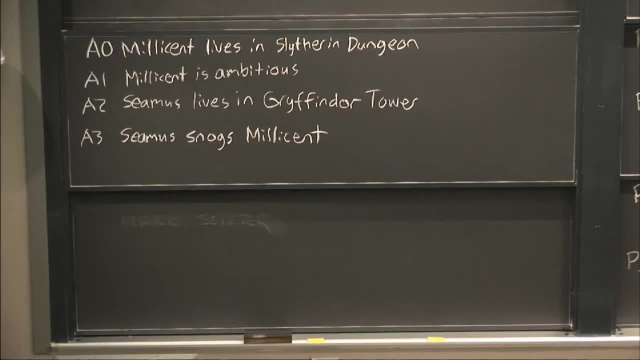 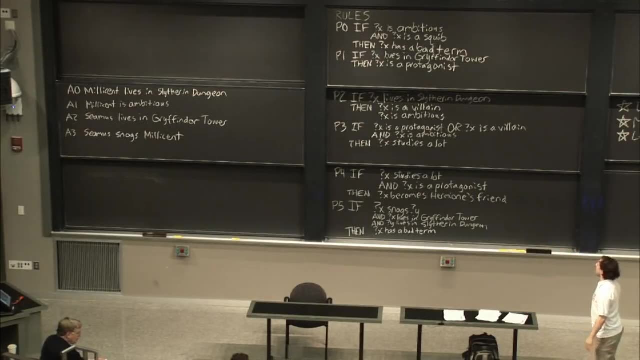 If you look at one of my rules, say, if x is ambitious and x is a squib, then x has a bad term. That's rule zero up at the top. That's written in sort of what we call in-fixed notation. It's easy, it's simple. all the operators are in the order you would expect. 2 plus 3 equals 5.. 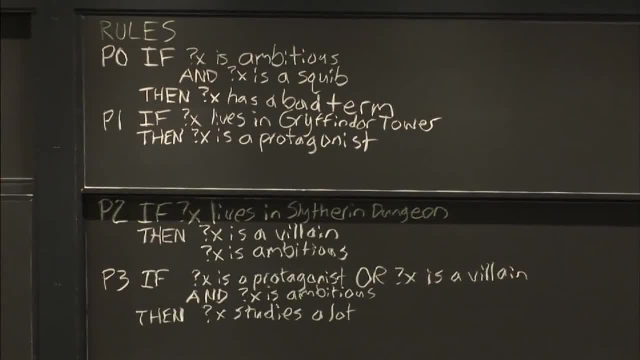 There's another kind of notation that is sometimes used on previous quizzes, and by sometimes a good number of times. actually, I'm not sure why we still use it that way, because of the fact that the classes moved on to Python, but we do sometimes. 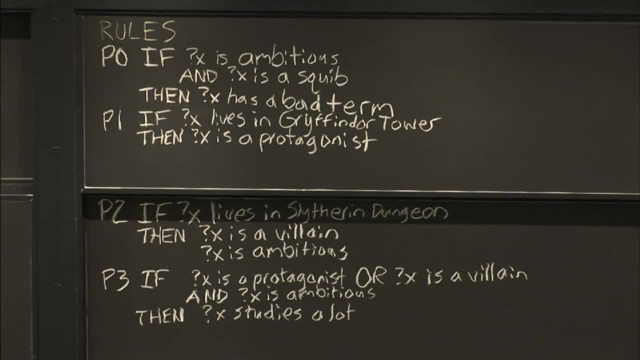 And that's called prefix notation. In prefix notation the operator comes first. So for instance: plus 2, 3 equals 5. The plus comes first. The function name comes first. In this case the function is plus. So if we were writing this in prefix notation: 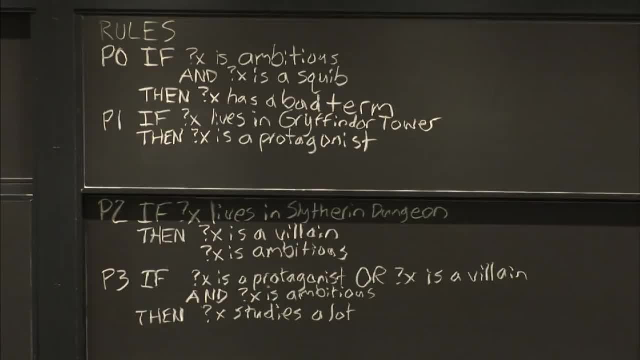 In fact, the way I received it, it said: if and x is ambitious, x is a squib, then x has a bad term. The and went first and there was a parenthesis which included everything that was scoped under the and. 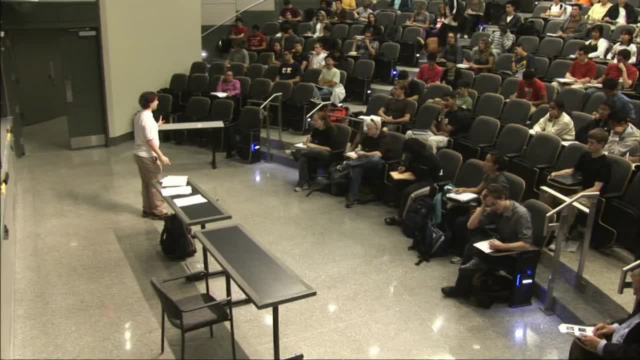 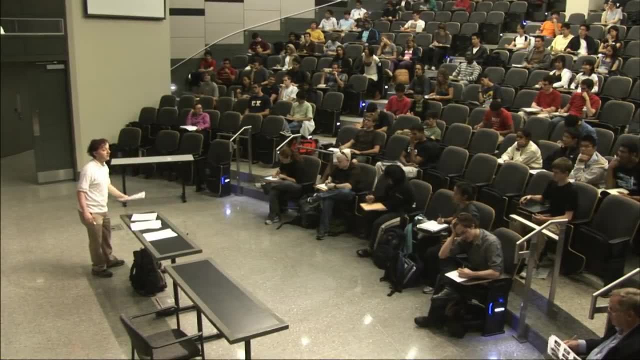 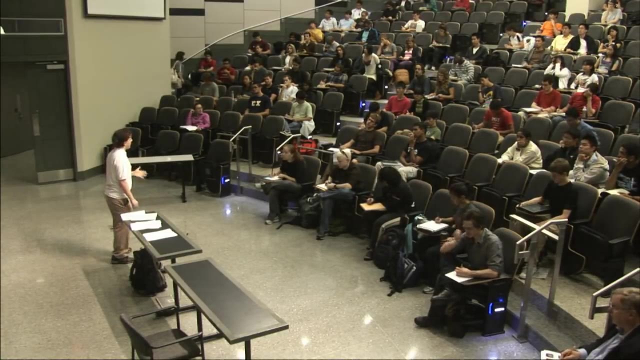 Does anyone have any questions about prefix notation, in case it comes up, Just remember, if things start being written in a really weird way, with lots and lots and lots of parenthesis, whatever is outside of the parenthesis, whether it be plus or and, or or is an operator that acts on the things that are inside. 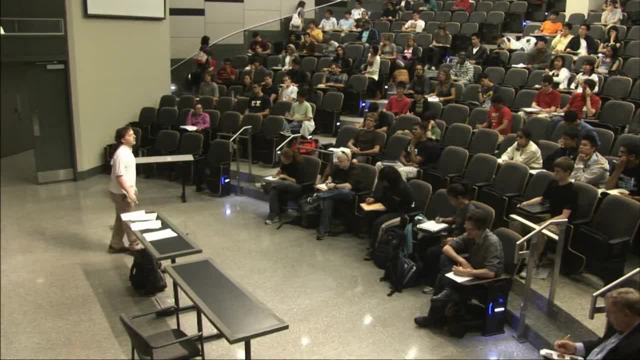 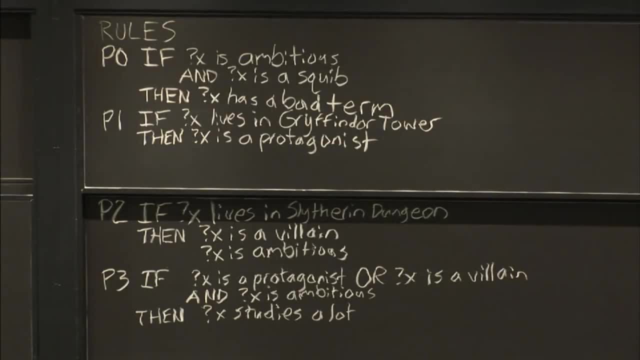 However, we're not going to deal with that now, because I think the most important thing is to understand the rules and the less important thing is to understand prefix notation, and you can do a problem at home that's written in prefix notation. to test yourself on that. 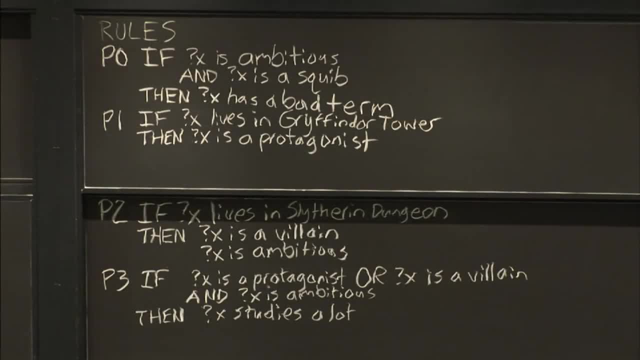 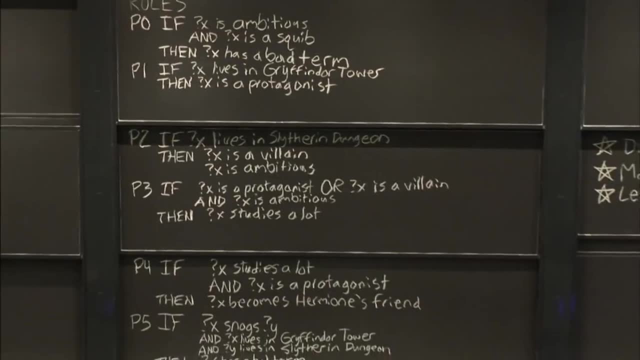 So what rules do we have here? We've got rules 0 through 5.. For some reason they are labeled with p's. They are often labeled with either p's or r's. The sort of secret on why they're labeled with p's is that one year somebody labeled 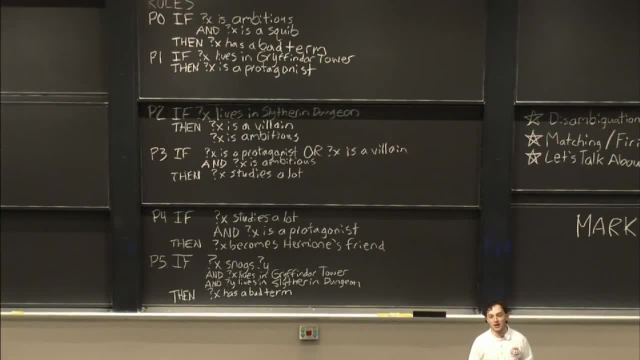 them with p's for like proposition or something like that. and then other TAs looked at that test and sometimes also labeled it with p's and it sort of down the line continued to be labeled with p's and sometimes with r's. So these p's are the six rules. 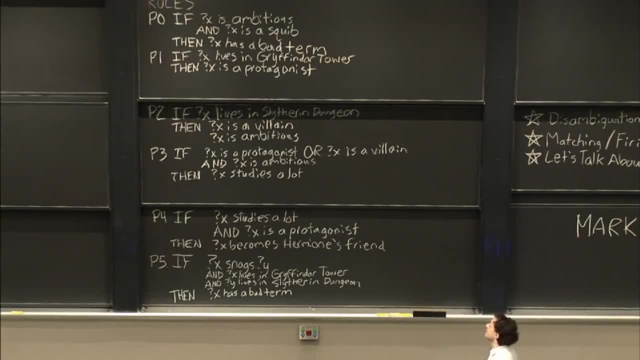 The first rule is: if x is ambitious And x is a squib, then x has a bad term. So what's the deal with these question mark x's? The question marks before an x or perhaps a y down here indicate that there's a variable. 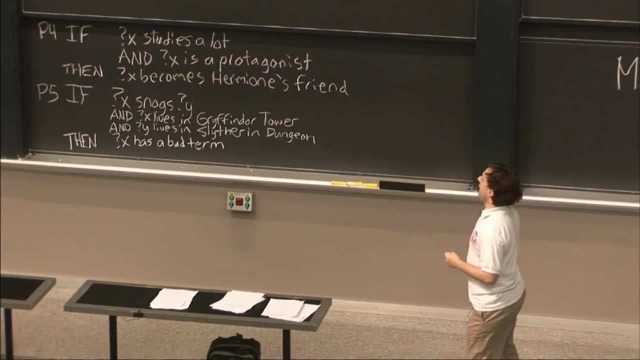 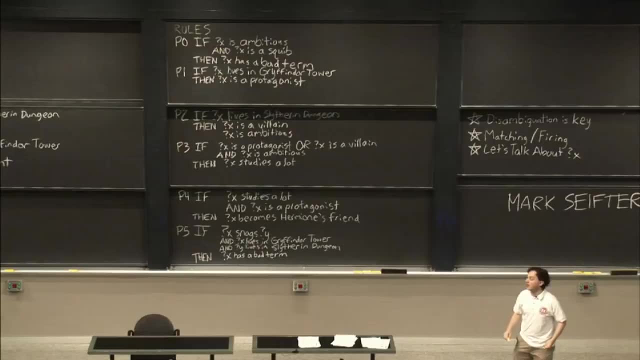 waiting to be bound. We're not assuming there's a Harry Potter character named x, and only if that question mark x the mystery character, only if mystery x character is ambitious can that person possibly have a bad term. What we're seeing is any character in the Harry Potter universe or not in the Harry 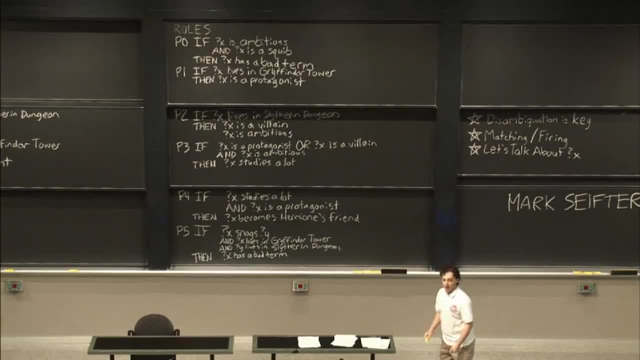 Potter universe. maybe a rhinoceros can fit into that x. So, for instance, if a rhinoceros is ambitious and a rhinoceros is a squib, then a rhinoceros has a bad term. That rule is saying for any x. this is true. 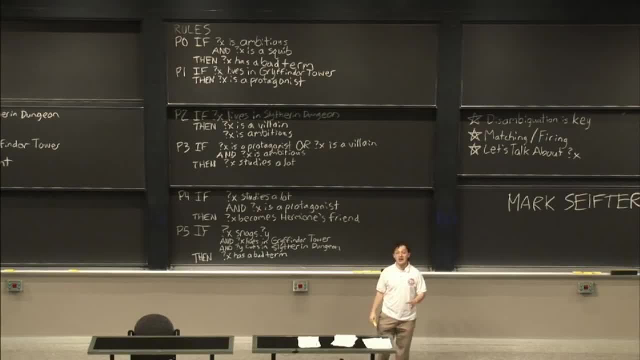 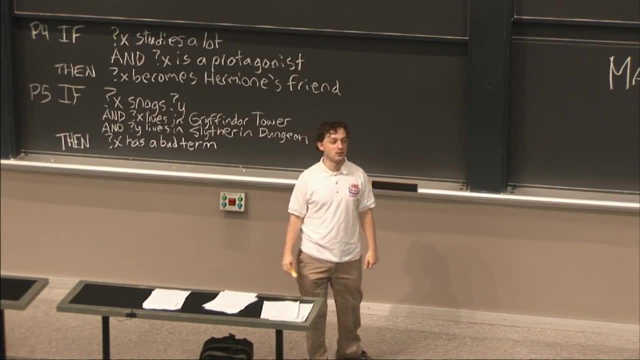 And it's very important how we treat the question mark x, how we bind the question mark x when we do both back chaining and forward chaining. I'll get back to that because some people made some very, very small mistakes that really messed up a lot of their forward and backward. 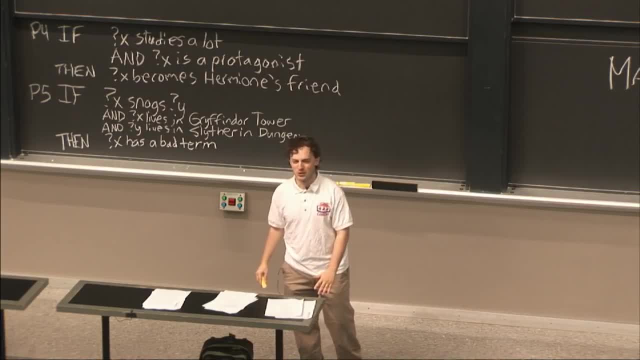 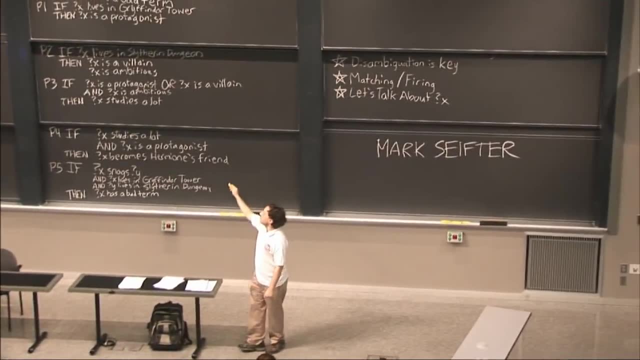 chaining last year. It was actually very tricky. Jeremy, the TA who wrote this was very clever and it makes it a really great case study for you guys. All right, So rule one: if x lives in Gryffindor Tower, then x is a protagonist. 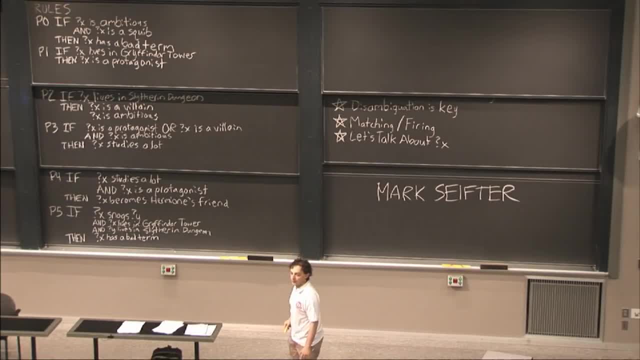 By the way, for conciseness, I'm going to be using gt for Gryffindor Tower when I write these later on, and I'll use sd for Slytherin Dungeon. So rule one: if x lives in Gryffindor Tower, then x is a protagonist. By the way, for conciseness, I'm going to be using gt for Gryffindor Tower when I write these later on, and I'll use sd for Slytherin Dungeon. By the way, for conciseness, I'm going to be using gt for Gryffindor Tower when I write these later on, and I'll use sd for Slytherin Dungeon. 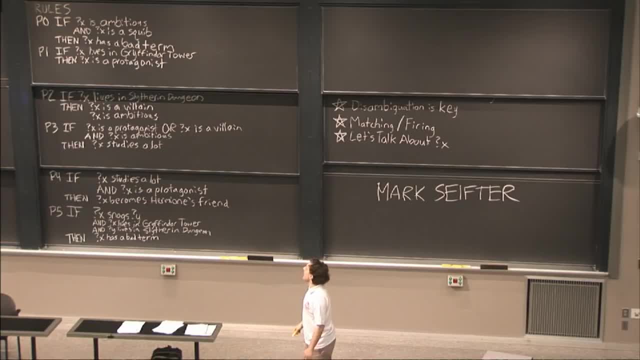 Speaking of which? rule two, if x lives in Slytherin Dungeon, then x is a villain, x is ambitious. Why are there two things here? Well, after the, if we have what we call the antecedent. That's something that needs to be true in order for this rule to match. 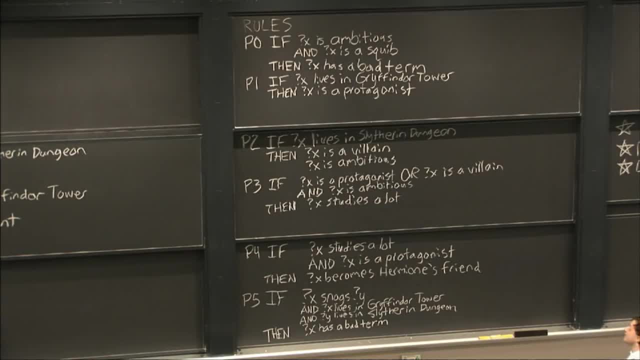 After the, then we have what is called the consequent, and in this case there are two consequences. Anyone who lives in Slytherin Dungeon is automatically a villain, and also ambitious, So you can sort of Think of there being sort of an and there for the purposes of both of those assertions. 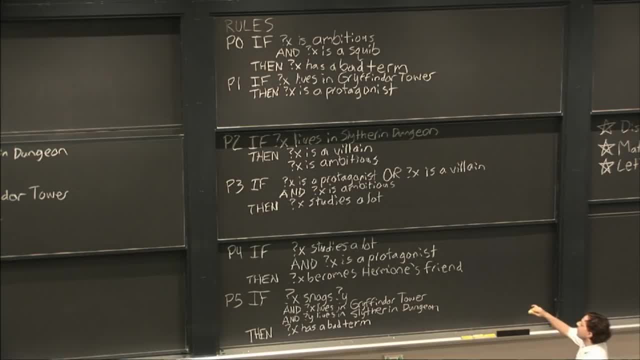 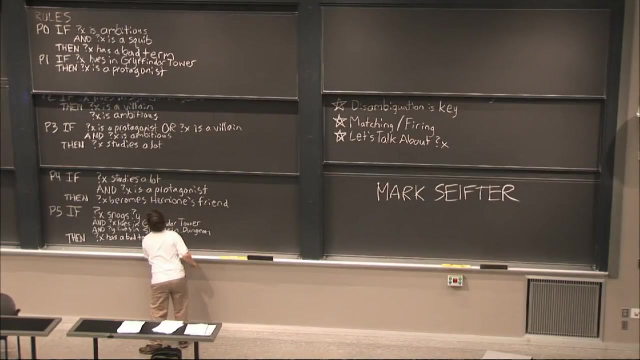 would be added to the knowledge base. Rule three: if x is a protagonist or x is a villain and x is ambitious, then x studies a lot. By the way, the scope for this- just to be sure that we're clear- is this: 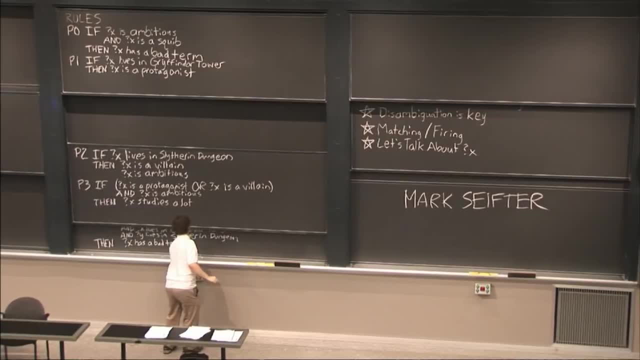 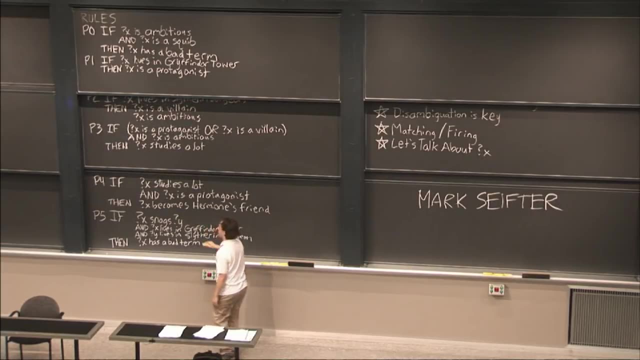 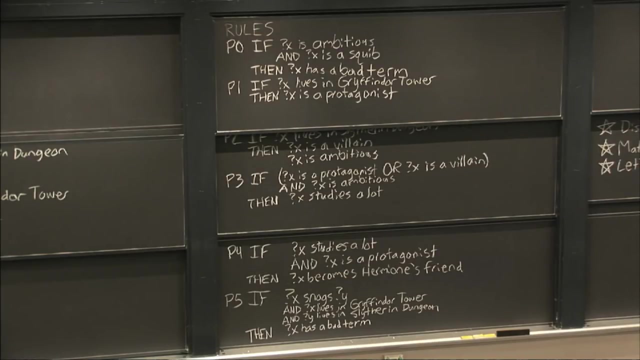 So we need them to be a protagonist or a villain and, no matter what, they have to be ambitious. Rule four: if x studies a lot and x is a protagonist, x becomes Hermione's friend. And rule five: if x snogs y and x lives in Gryffindor Tower and y lives in Slytherin. 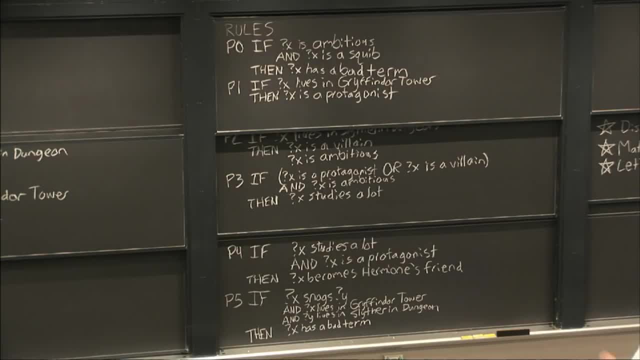 Dungeon, then x has a bad term. So those are our six rules that we can use to understand Jeremy's world of the Harry Potter series. I hope you enjoyed this video. I hope you enjoyed it. I hope you enjoyed it, Thank you. 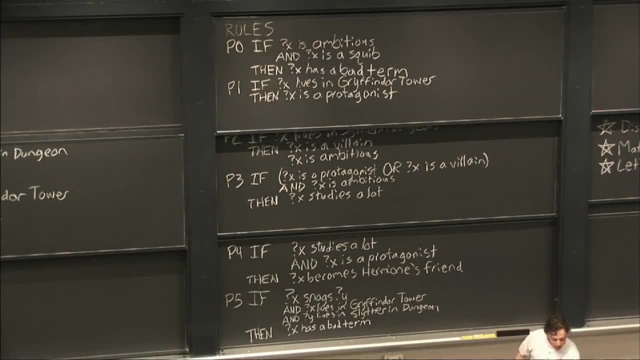 I hope you enjoyed it And start your quickly. Number four: think about ourselves. Then thank you for all the good facts in our universe. And we also start off with four assertions. Let me not underestimate the value of always looking to the assertions. 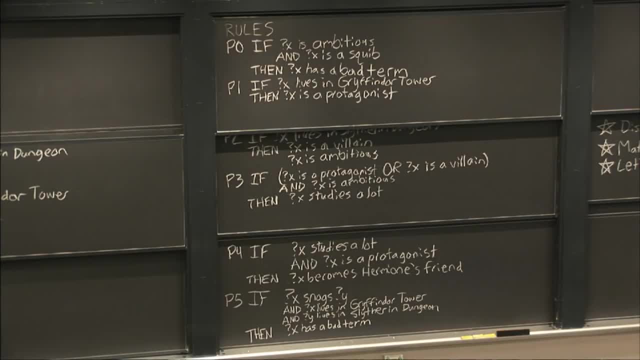 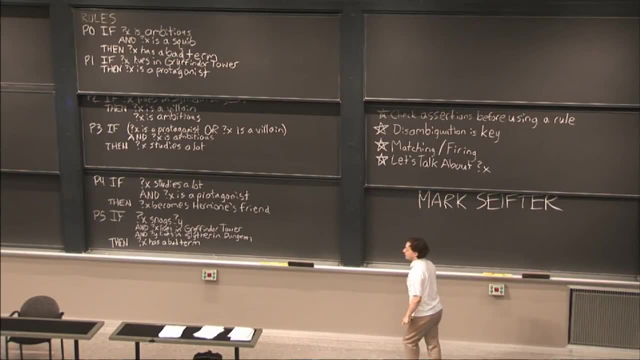 It's one of my white star ideas that are up here on the board. let me see. No, not that one. That's uh, perfect. Um, always check the assertions before using a rule. This really tripped people up last year. 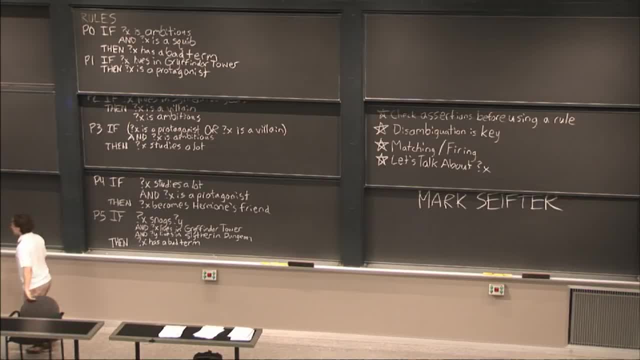 You'll see why, cause we're doing last year's problem Um Our four assertions that we start with. Assertion zero: lives in Slytherin Dungeon. Assertion one: Millicent is ambitious. Assertion one is what tripped people up, so remember that Millicent is ambitious. Assertion two: Seamus lives. 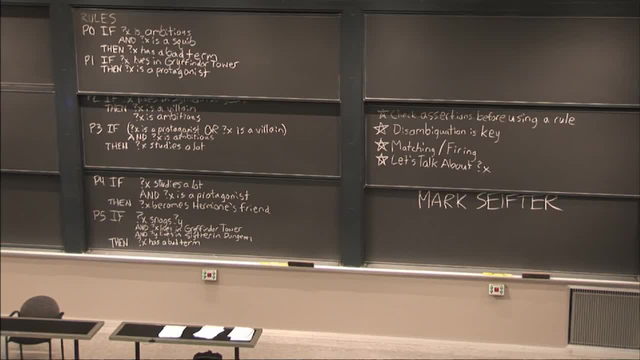 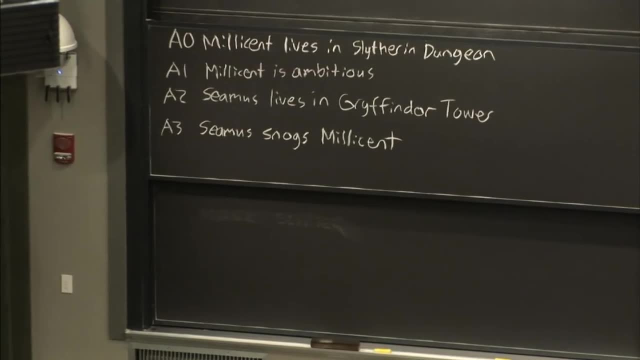 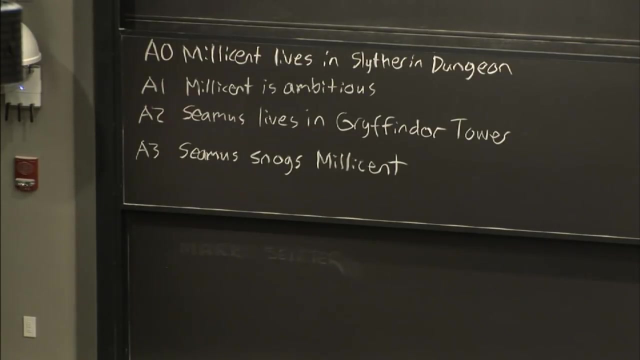 in Gryffindor Tower. And assertion three: Seamus snogs, Millicent. So those are our four assertions that we've already started with. Now the two things we're going to have to do are backward chaining and forward chaining. Now, when you guys learn these two backward? 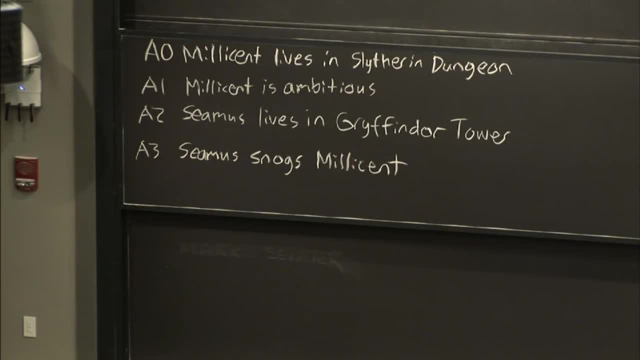 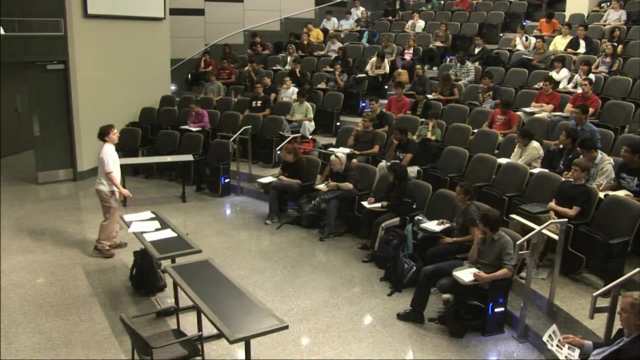 chaining and forward chaining. raise your hand. if you thought forward chaining was harder than backward chaining, Aha, I knew it. I can prove whatever point I want, because no one wants to raise their hand, Because I also think backward chaining is harder than forward. 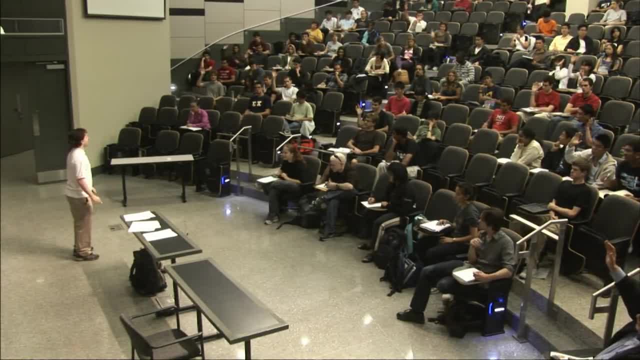 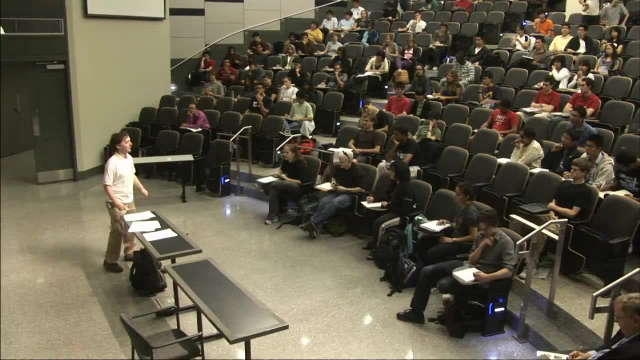 chaining. Raise your hand if you think backward chaining is harder than forward chaining. First of all, we have a good number of people. Second of all, since no one wants to raise their hand, I could just ask it the other way. That's a pro tip if you're ever with 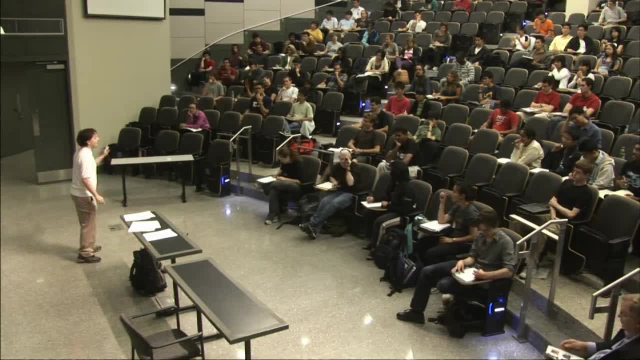 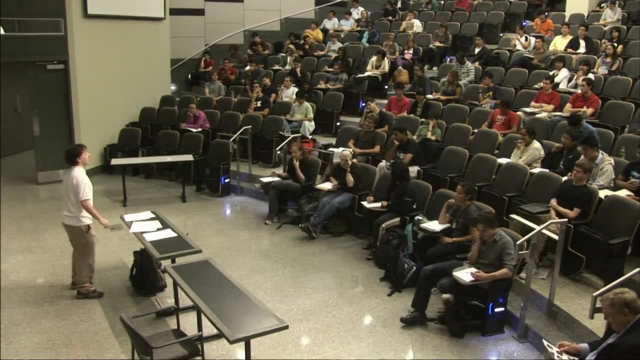 a large group of people. You can prove any point you want by Asking the other direction. no one will raise their hand. So I agree that backward chaining is harder than forward chaining And I disagree with Patrick that we're going to get out of. 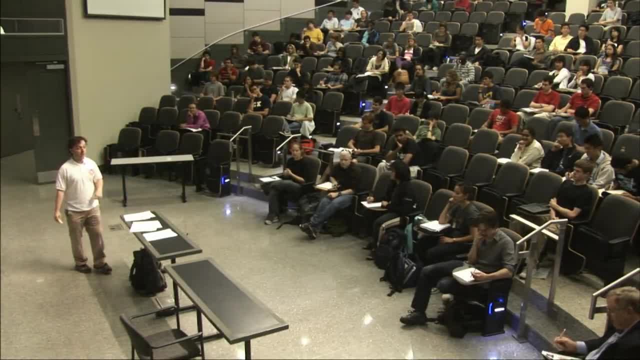 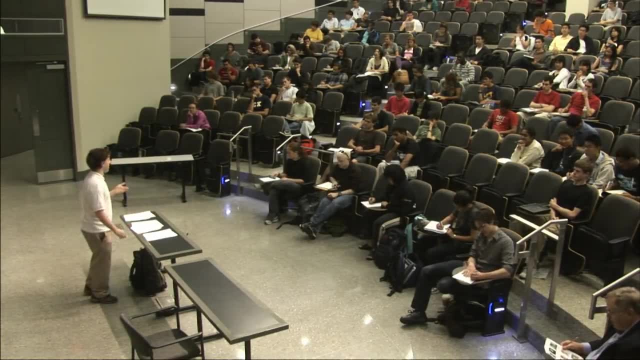 here early. So let's start with backward chaining first, so that we make sure that we spend the bulk of our time with it. Because forward chaining, well you know, you just go through, You go through pretty methodically and add new rules. Backward chaining, you have to. 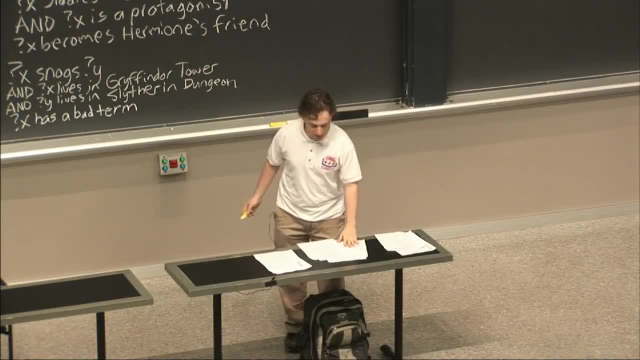 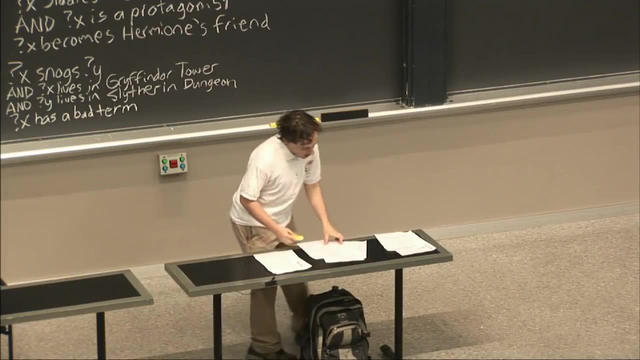 draw this crazy tree. There's a lot of places to get lost in the middle of the road, So let's do some backward chaining, And to do that I'll do it over here on the left side. So when we're doing backward chaining, we have to remember a few things that are written. 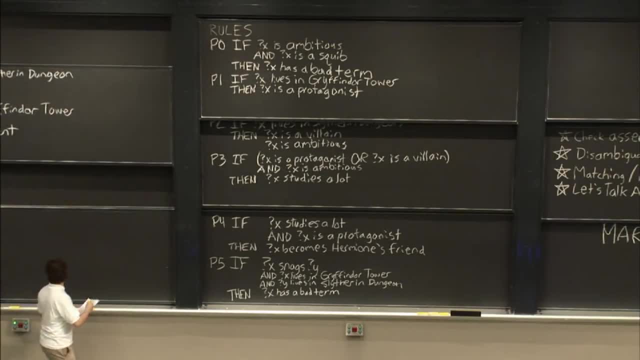 directly on the quiz, so you're not going to have to worry about that. But they're still pretty important, So actually I'll write it on here first. I'm going to read them off. So when working on a hypothesis, the backward chainer tries to find a matching assertion. 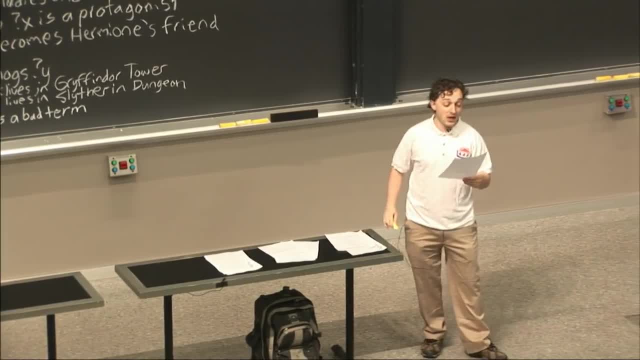 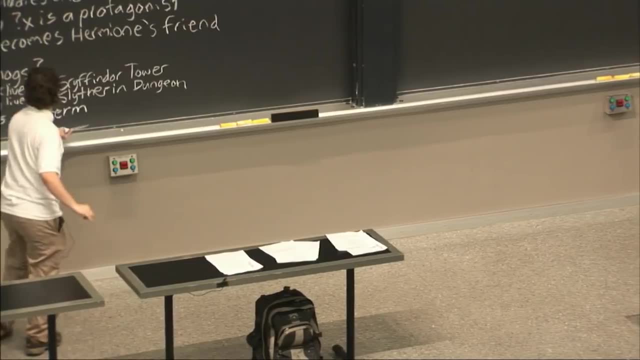 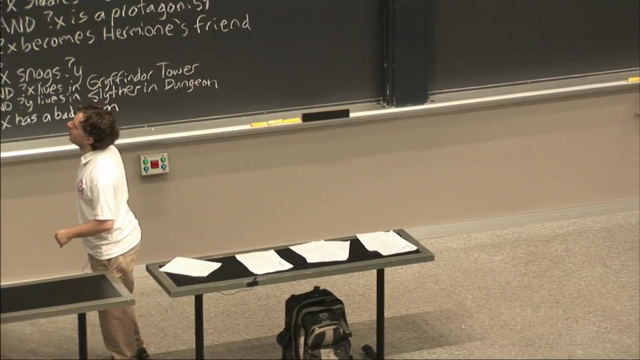 in the list of assertions first. If no matching assertion is found, the backward chainer will try to find a rule with a matching consequent, a rule that has something in the then that can prove the assertion it's trying to figure out. So, for instance, if I was doing backward chaining on Seamus-Snoggs-Millicent, what happens? I'm 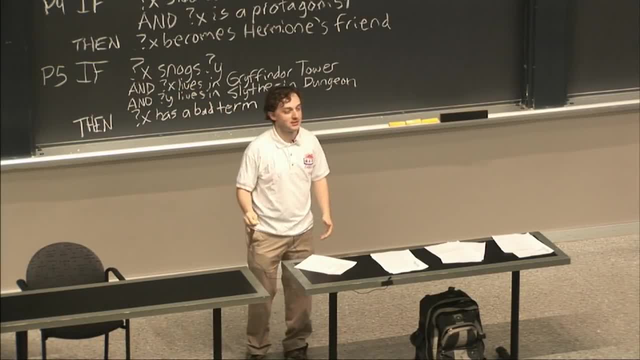 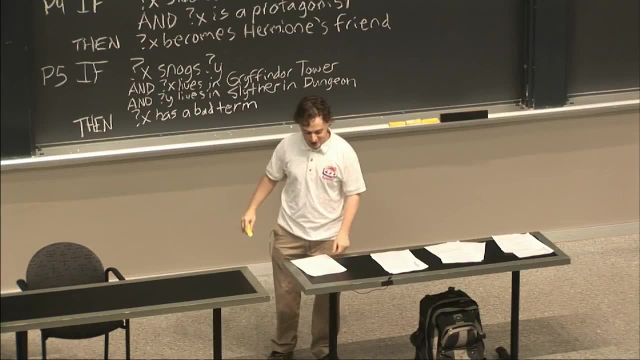 immediately done, because there's an assertion, assertion 3, that says Seamus-Snoggs-Millicent, I've proved it, I'm done, I'm happy, We can leave, We can go home. Unfortunately, that's not what the quiz asks us to do. Well, let's say that instead, we're. 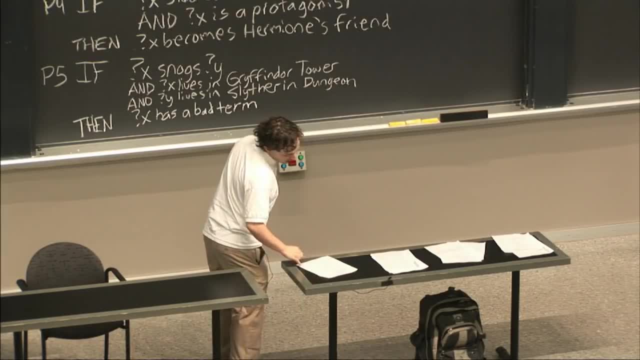 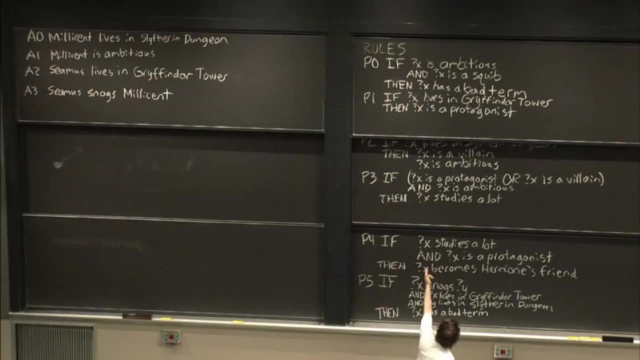 Instead we were supposed to say: I don't know, Seamus is a protagonist. Well then, we'd wind up looking through here and we would look at the fact that rule one can prove that someone is a protagonist, And we'd recurse and try to prove. 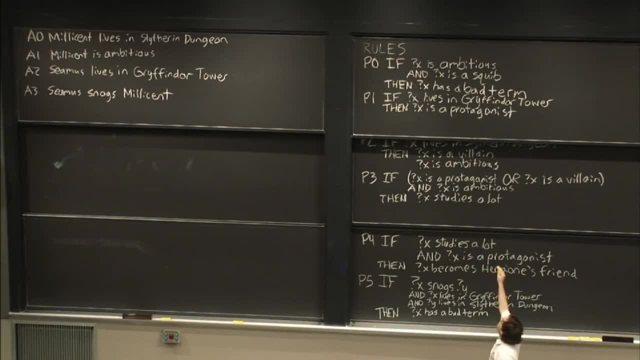 whatever is in the antecedent of rule one, which is OK. well, does he live in Gryffindor Dower? Assertion two: he does. So that's some really quick, and if that was too fast, don't worry. 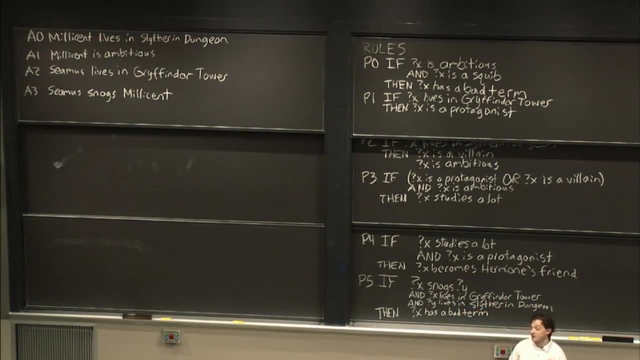 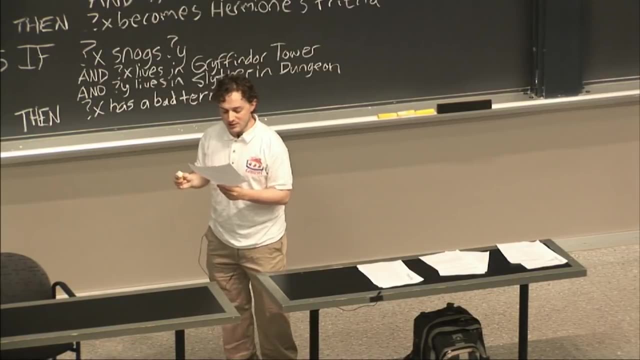 We're going to go step by step with the actual problem, But I just wanted to give two really easy problems really quickly. how it's going to do it. Let's go step by step with the real problem. Let's keep in mind the backward chainer never adds. 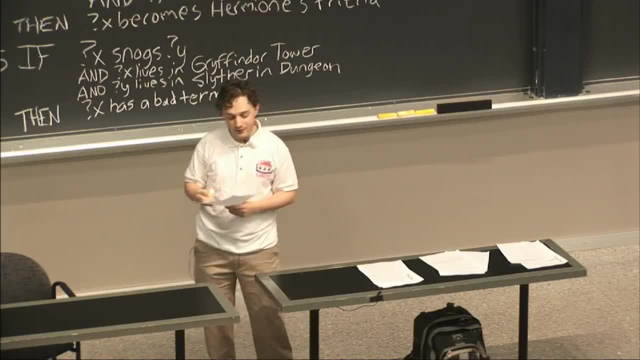 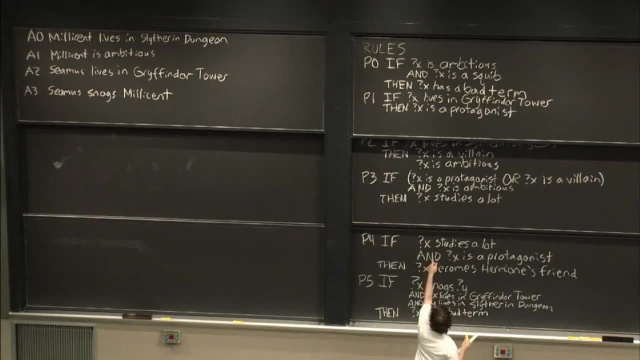 new assertions to the list of assertions And if you have a tie break, you always order based on rule order, first P0 through P5. And if the same rule matches with more than one thing in your list, Then you tie break based on the order of the assertions. 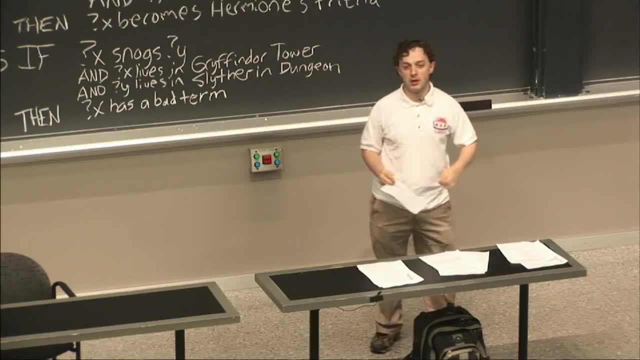 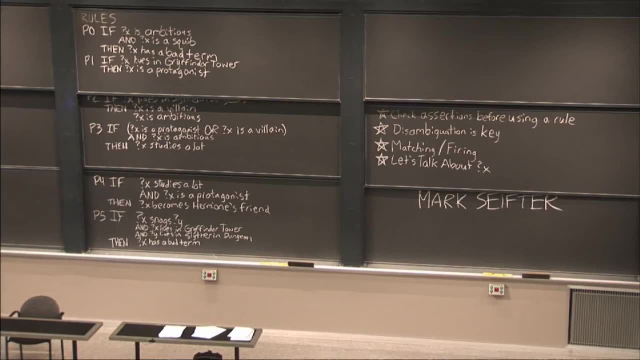 Very important. disambiguation and tie breaking are a big place to get messed up. So we're going to try to prove that Millicent becomes Hermione's friend, And so I'm going to abbreviate some of the things, but not for the very first line. 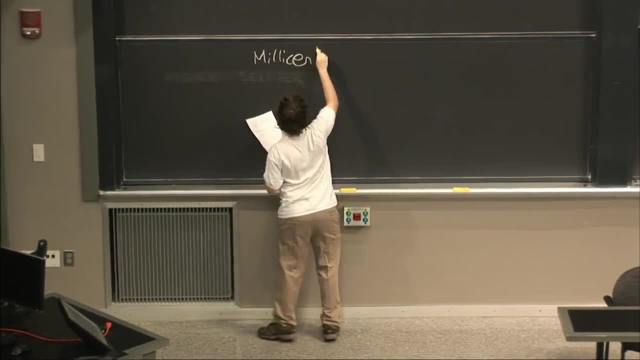 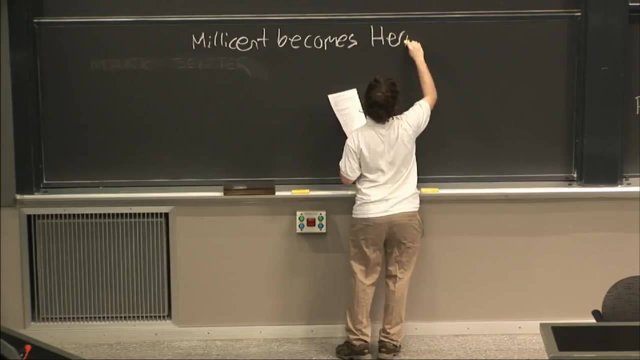 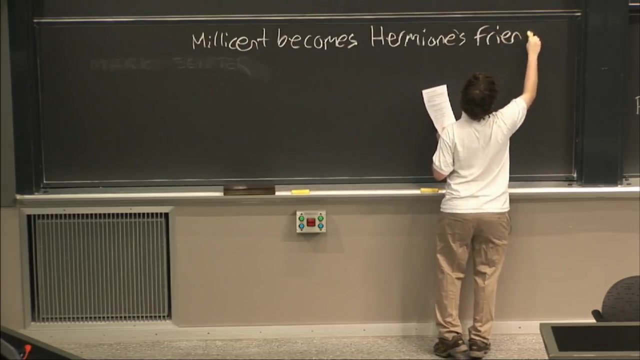 So Millicent- Millicent becomes Hermione's friend. We start drawing a gold tree. Now you guys are going to learn exactly what these mean. very soon in fact, next lecture. But for now, trust me when I say these gold trees are. 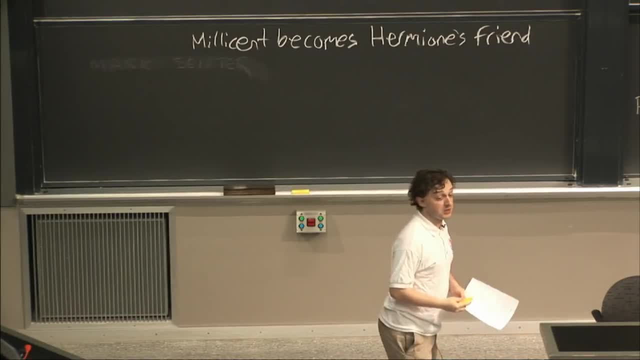 depth first, And I'll explain what that means, because some people have messed themselves up and spent more time than they needed to by treating the gold tree in a different way. Now Millicent becomes Hermione's friend. Let's pretend that we're the backward chainer. 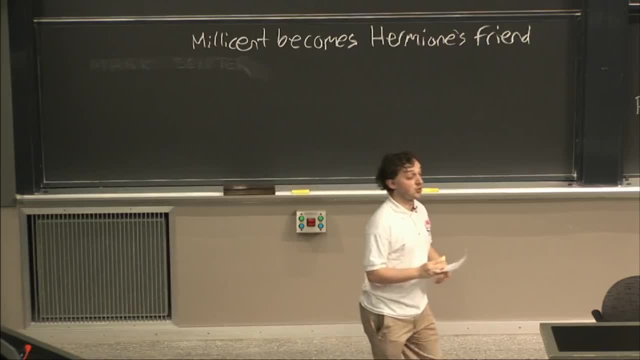 We're trying to prove that this is true or disprove and say, well, it's definitely not true with what we have. So let's see, I'm now going to make you guys help, And people in the back think they won't be called on. 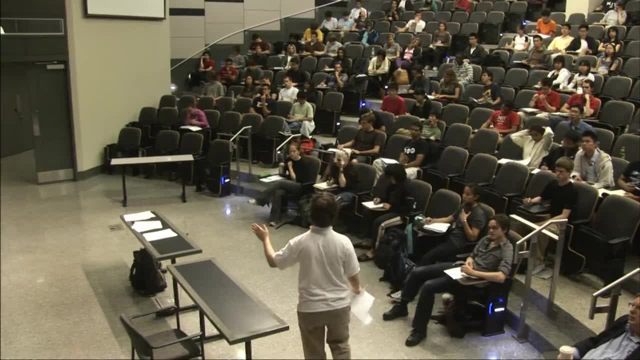 So I often like to call the people in the back. What do you think is the first thing we should do? Very first thing: Matching insertion. Yes, Look for matching insertion. Excellent. Do we have a matching insertion everyone? Yes, 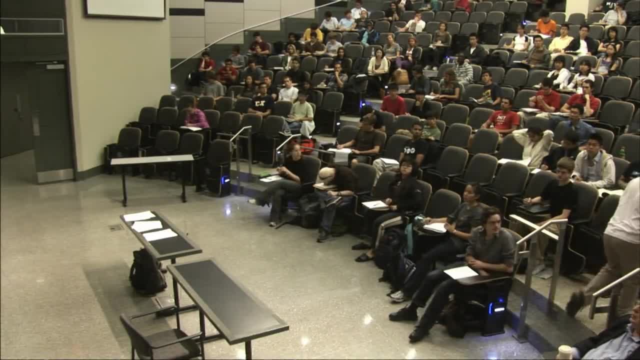 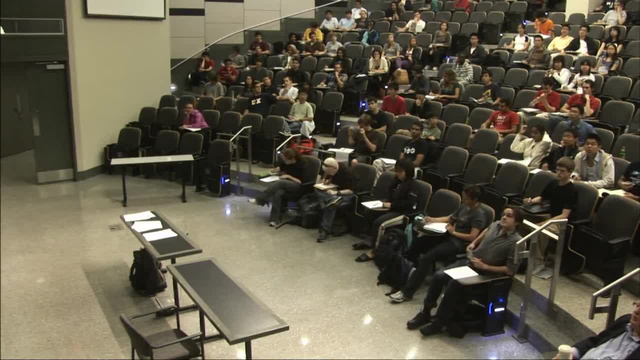 We do not have a matching insertion- Great. So since we don't have a matching insertion, what? now We start to look at the rule. That's right. And do you see any rule that could prove that Millicent becomes Hermione's friend? 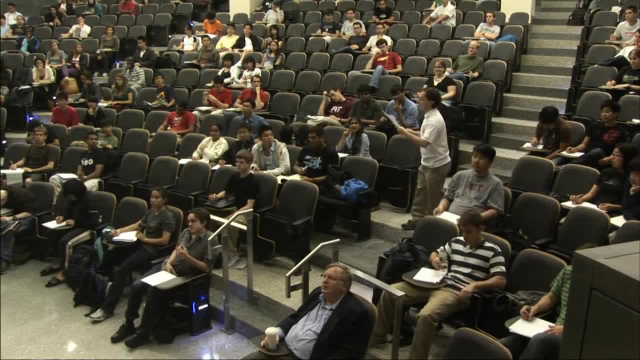 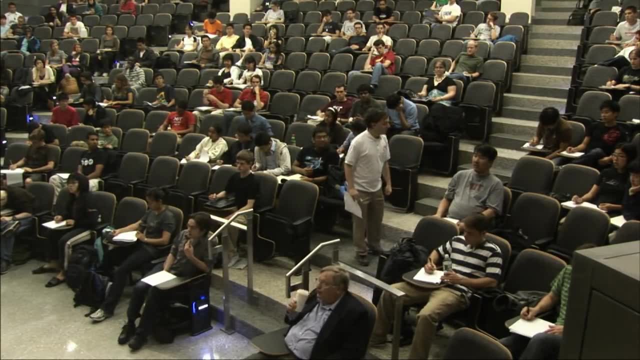 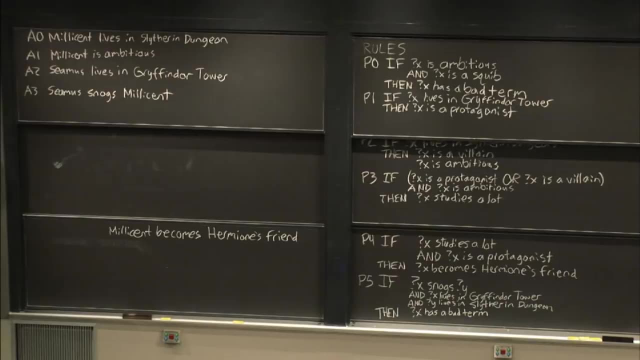 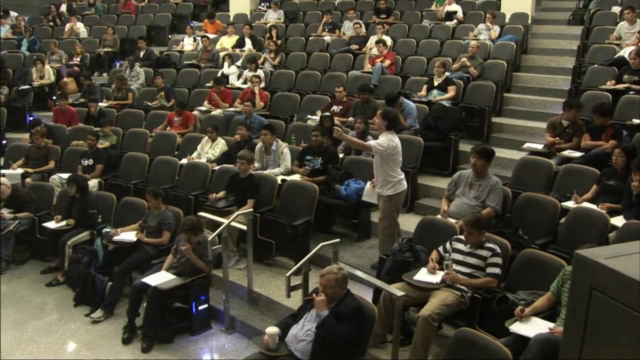 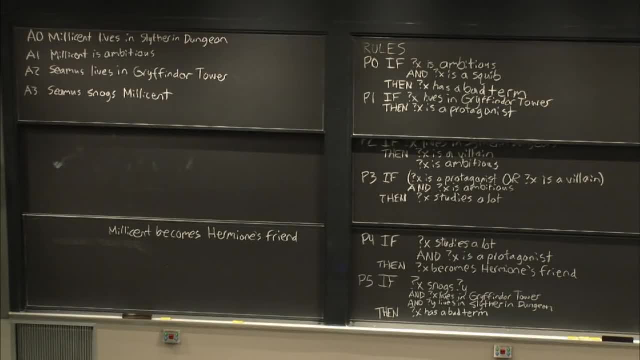 Anyone is capable of being Hermione's friend- Great. So P4 is our rule of the hour. So we're going to use P4. And when we use P4 to prove that Millicent becomes Hermione's friend, we're going to. 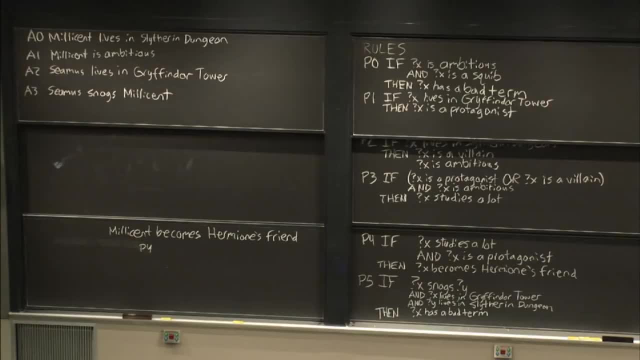 have to add something or another to the Goal Tree. So let's see, What do we have to add to the Goal Tree? This, That's right. Does everyone see that, In order for her to become Hermione's friend by rule four, 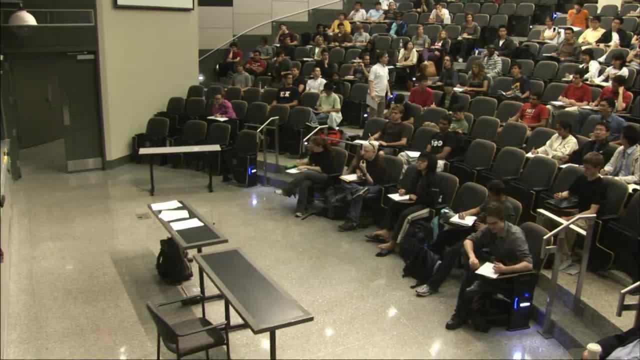 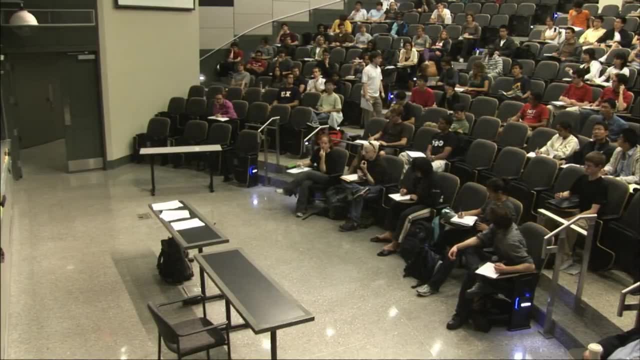 you have to see if she studies a lot and is a protagonist Question. Okay, that's a very good question. You're going to get screwed up if you look at the antecedent in backward chaining first. It's backwards partially for a reason. 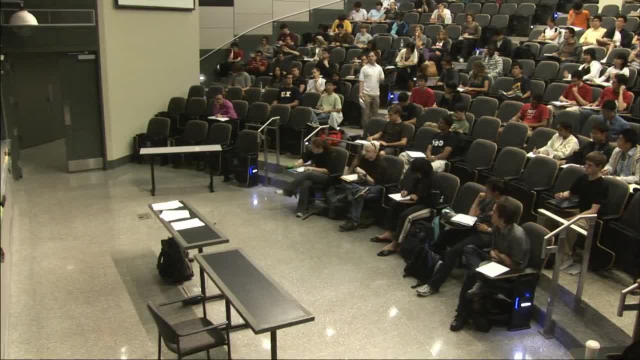 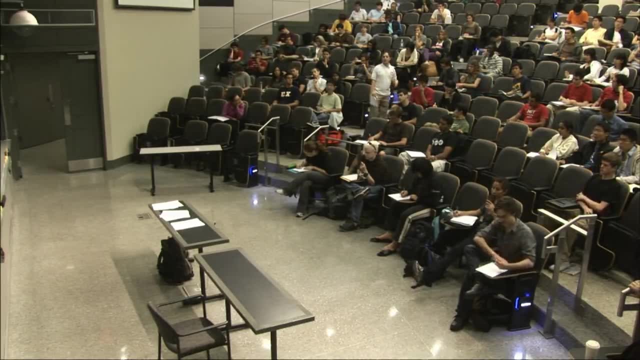 You need to look at the consequent. Now, why is that? Well, let's say there was a rule, rule six. It said: if X becomes Hermione's friend, then Hermione feeds X Polyjuice Potion, or something like that. 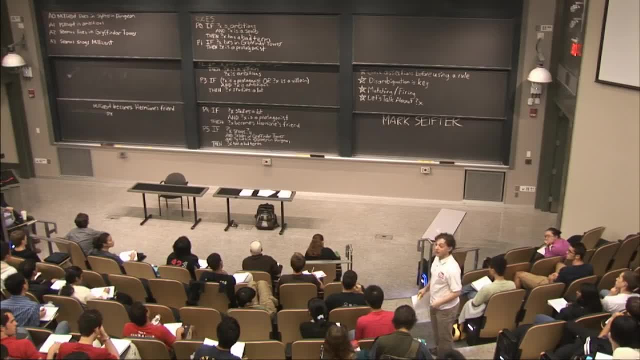 Will that rule help us in back chaining to figure out if Millicent becomes Hermione's friend? Some people are shaking their head, but think about it. Will that rule be able to prove it? No, Now, if they do become Hermione's friend. 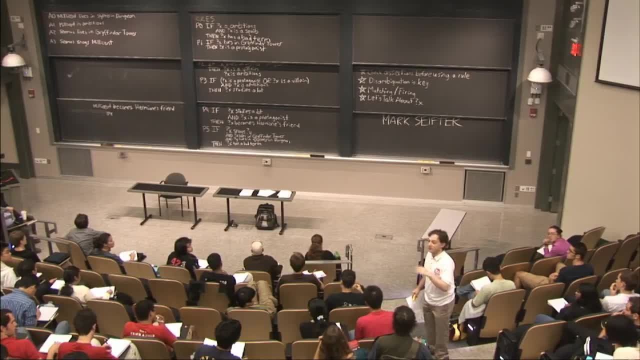 and we want to do some forward chaining, we'll figure out that they're going to transmute into some kind of other thing because of the Polyjuice Potion, but it's not going to help us do the one thing we want in back chaining. 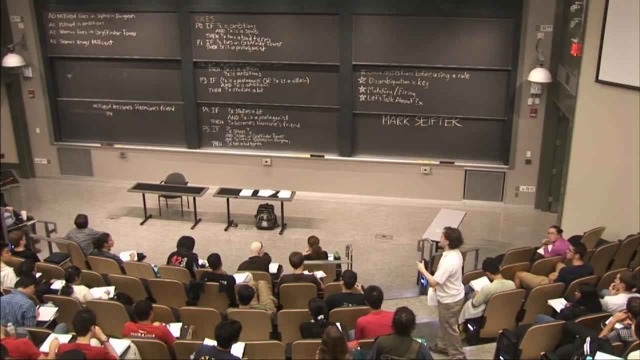 which is to prove that thing on the top. So we actually need to look for something that has our current goal and its consequent. Then we add on the antecedents As people I've asked so far. sorry, I don't know your names, like Patrick, 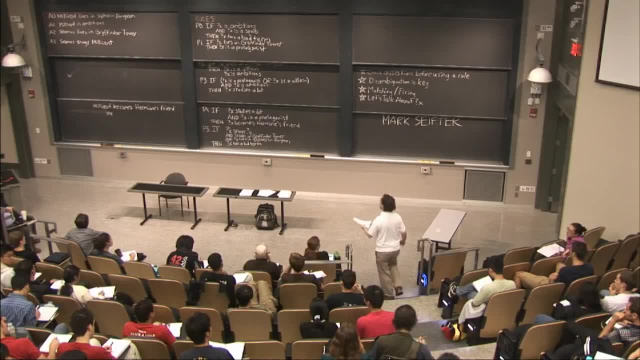 have correctly given me every time, which is excellent. So notice also that she didn't say X studies a lot needs to be added to the goal tree, She said: and Millicent studies a lot. Oh, another question. Great, It's obvious. 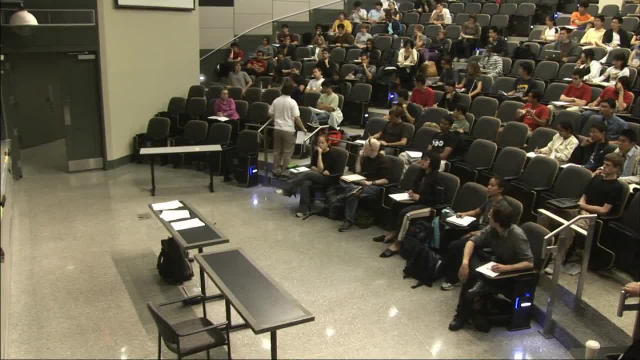 but after putting rule four in there, should we first check the assertions? Check on the assertions if our conditions are within rule four, because then we wouldn't have to search for other rules. The question is, once we put rule four in there, should we check to see? 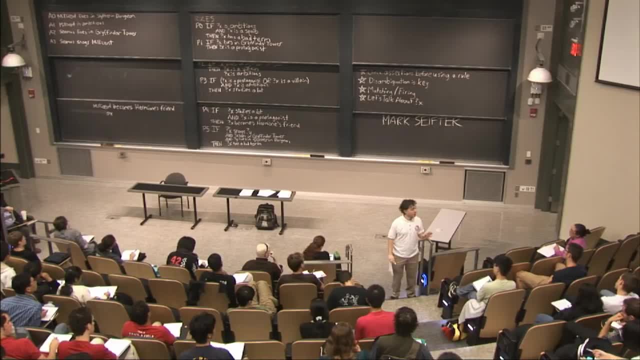 if those antecedents of rule four are already in the assertions, before checking other rules, The answer: you're not only correct, sir, you're exactly one step ahead. So I'm going to assume I called on you for the very next thing. 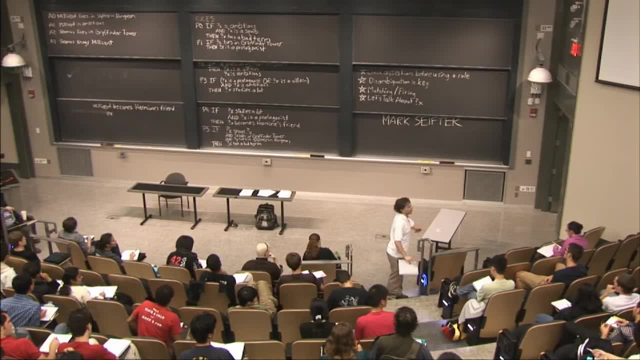 That's exactly what we do. once we draw it onto the tree, You're exactly on the way. Further question: Perfect, So All right, Great. So again we're putting up Millicent studies a lot. Millicent is a protagonist. 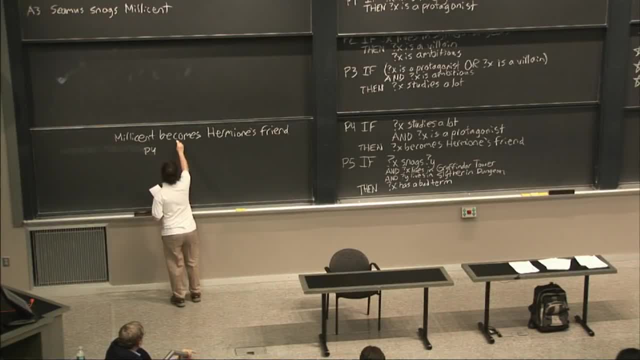 We're not putting up X. Some people did that And of course it's an AND node, as we heard. We need them both to be true, or we're not going to be able to continue onward. So we have, I'm going to use M for Millicent. 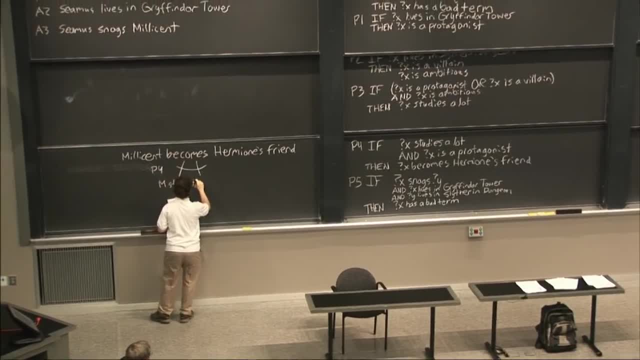 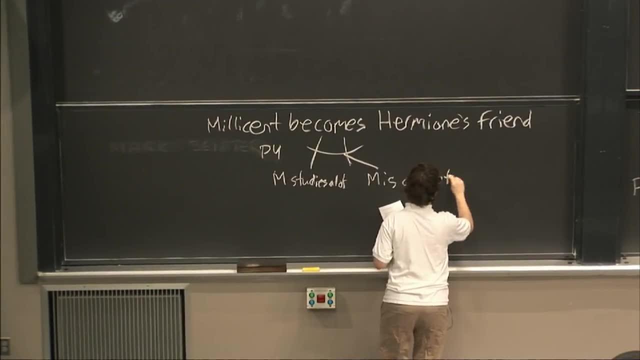 Millicent studies a lot Also over here. Millicent is a protagonist, Great- And we've already heard that we need to search in the assertions before we go into any rules for what we're looking for next. The question is: 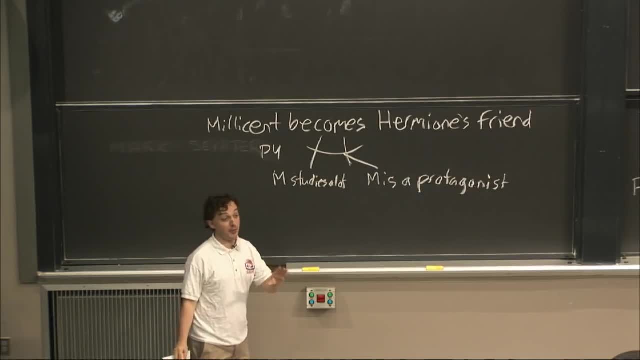 what are we looking for next and in what order? This is where that thing I told you about depth search is crucial. We're going to look here on the left node And if it has any children, if we have to keep going down. 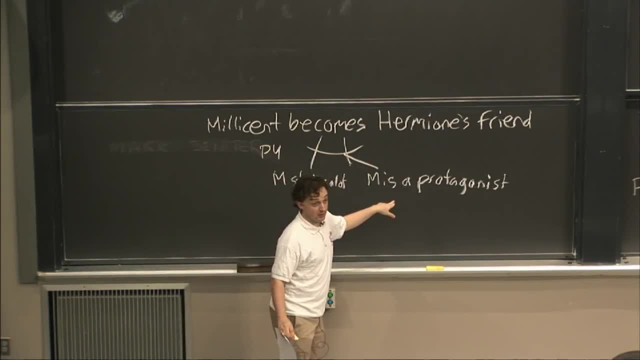 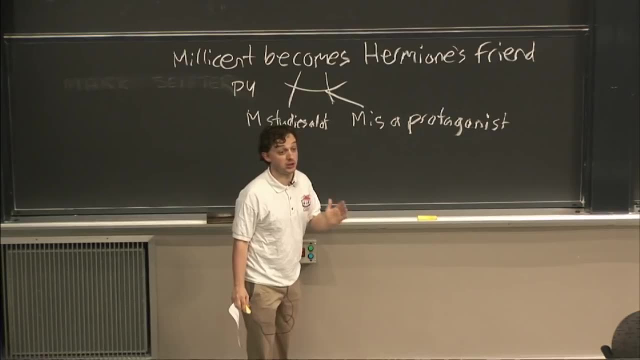 we are not going to look here yet, All right. There's a few reasons for that, one of which is that we're lazy. The evaluation, if you learned about it, is also if you learned about lazy, evaluation is also lazy. 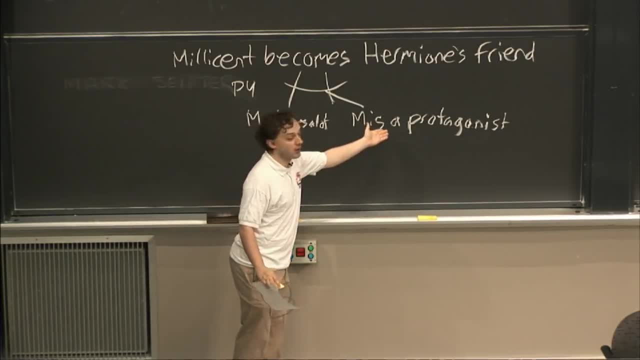 And if we can disprove this studies a lot branch. we don't have to do any work with the protagonist branch. We're done, We're out of here And it's, and it's a, it's a loss, All right. 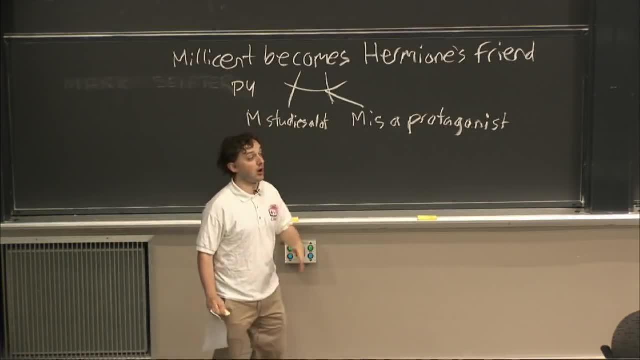 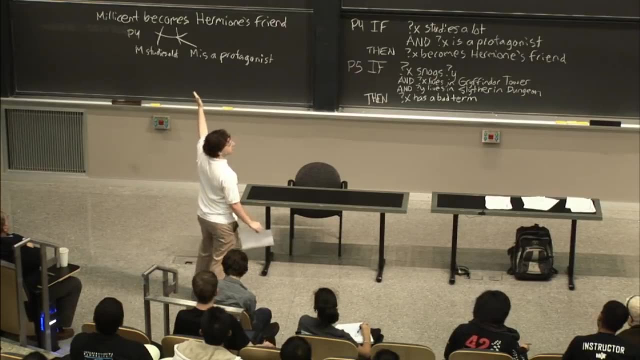 So we're going to move down the studies a lot branch And we already heard from the audience. we need to look to see if it's in the assertions. Everyone is studies a lot. Millicent studies a lot in the assertions. 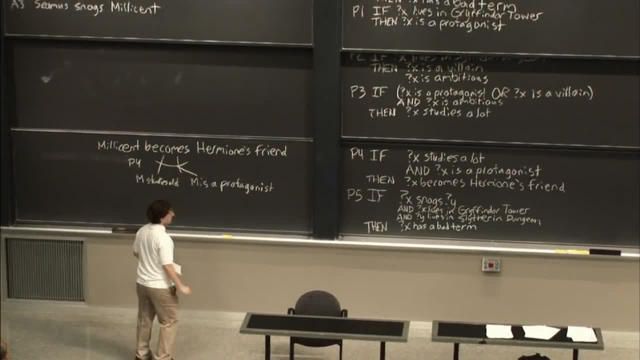 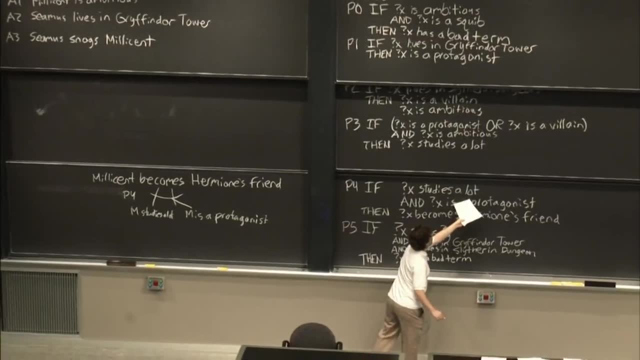 No, it's not All right. Well then, now we're going to get to that question that I had before about the antecedent or the consequent, because studies a lot is here in the antecedent of rule four, but we're not going to be able. 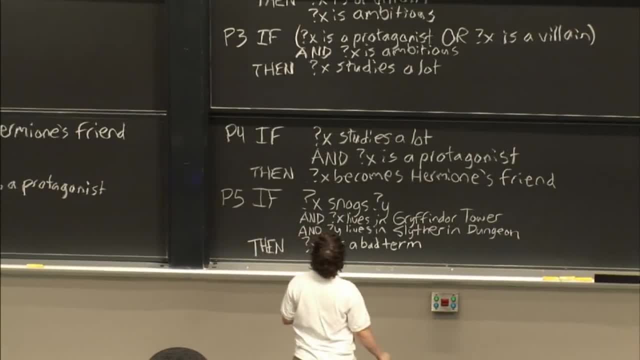 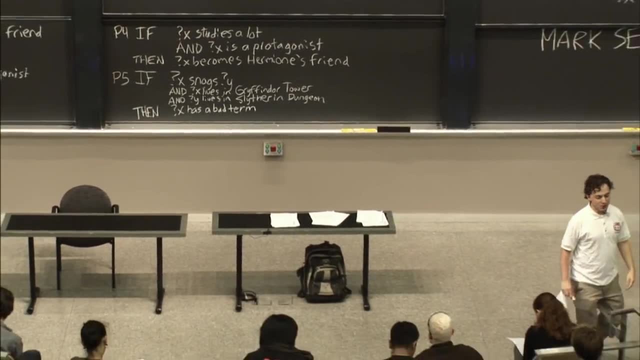 to use rule four here. In fact that's how we got here in the first place. So question is: let's see. the question is: do we have a rule that matches in the in the consequent? that matches Millicent studies a lot. 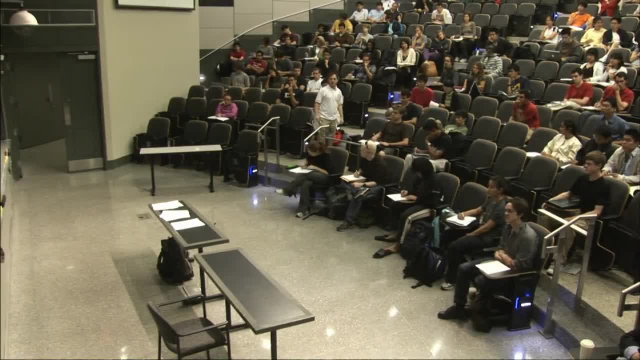 Yeah, P3.. Yep, that's right, P3. And P3 would be perverted, That's right. So P3 is would give us Millicent studies a lot. and so, therefore, what do we add to the goal tree? 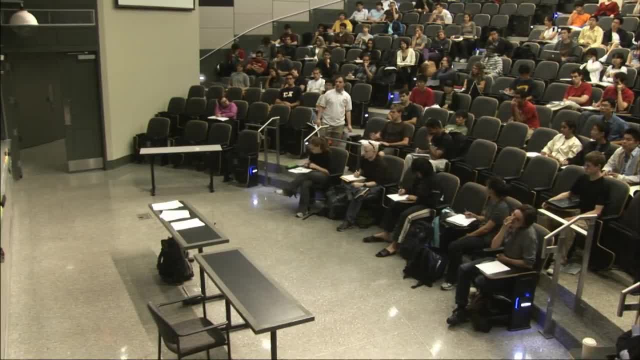 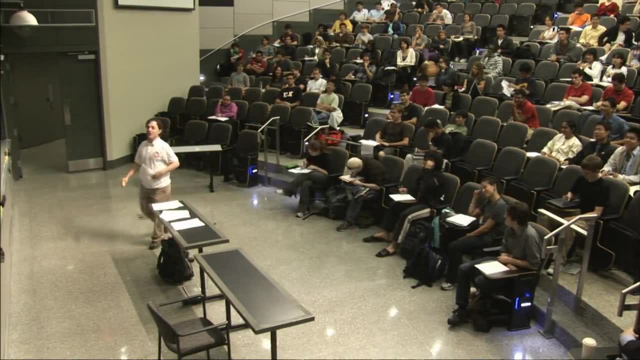 We add: we add both: that it is Millicent, either a protagonist or a villain, and that he's a bitch. Yep, she turns out to be a girl, All right. So that's exactly right. We heard that we need to add. 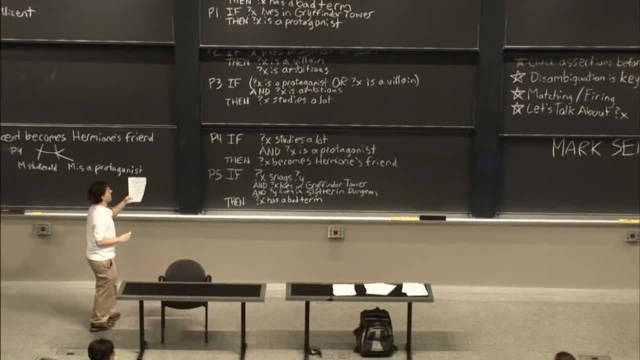 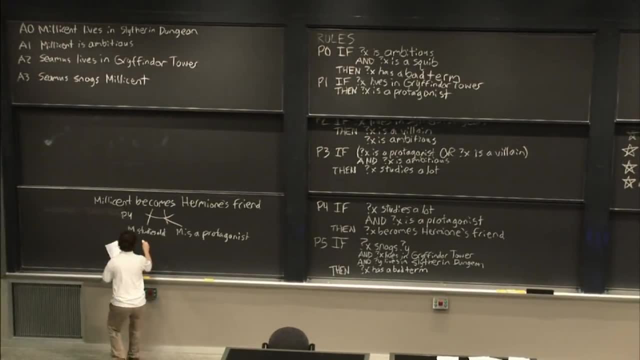 we need to add an and node, which also has an or node at the bottom of it, because this is a little bit of a complicated rule. So we have an and node, So we have an and node. and the first thing on the and node, 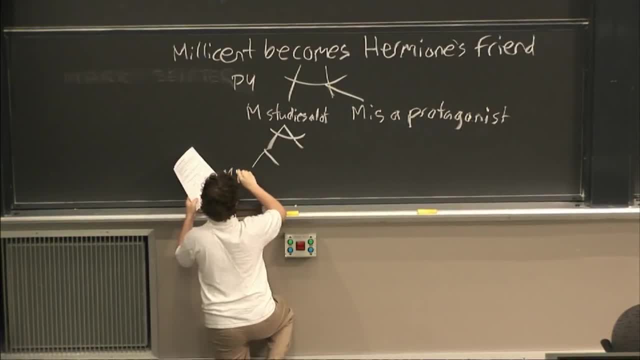 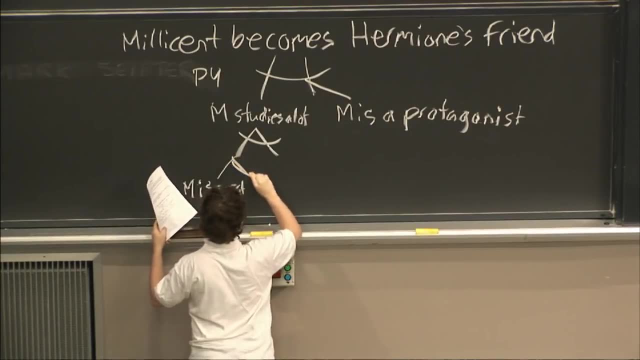 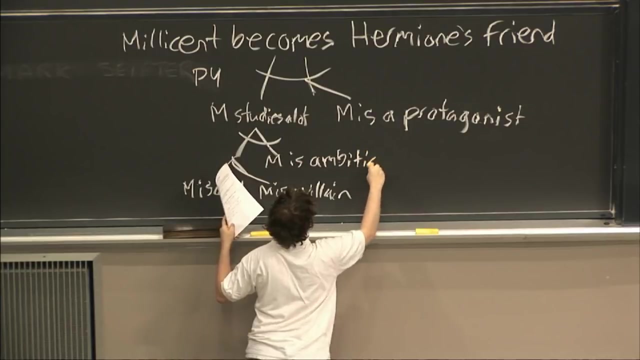 is: Millicent is a protagonist or Millicent is a villain. And the second thing on the and node is: Millicent is ambitious. Well, actually that is the second thing on the and node. I hope that's what I said. 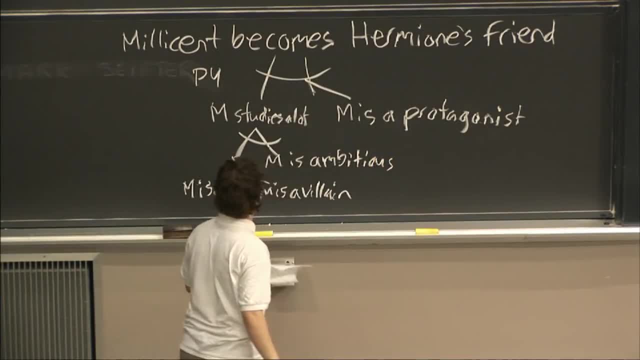 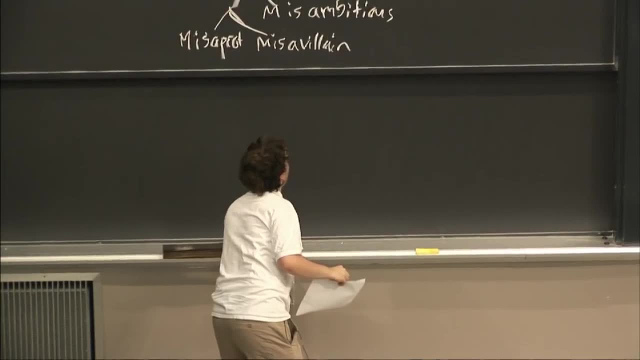 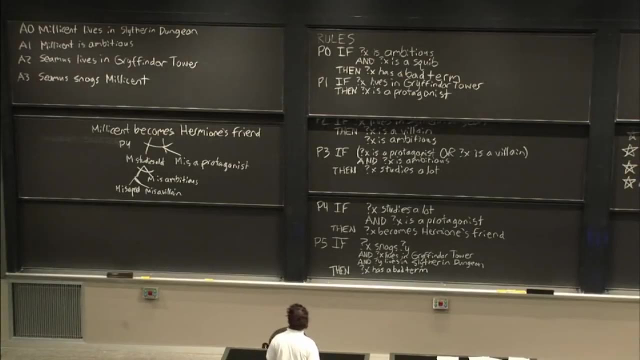 All right. The second thing on the and node is: Millicent is ambitious, Great, Okay. So here's our handy little tree. Now, this is where it's important. As I said, we're doing a depth-first search. 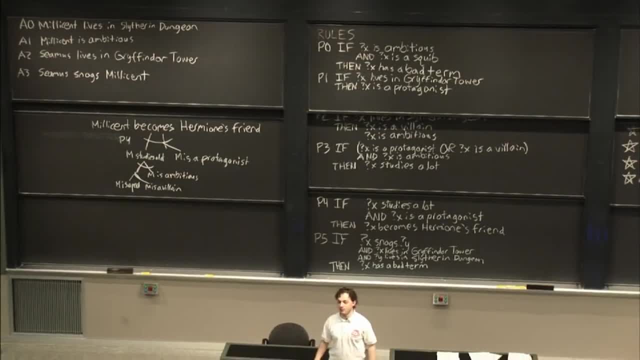 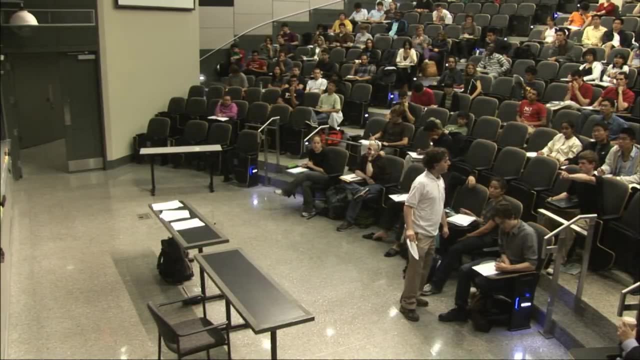 We're going down along the left branch, So where do you think we're going to go next? on this tree? Not quite. That's a good guess, You didn't. you didn't say we're trying to prove M is a protagonist. 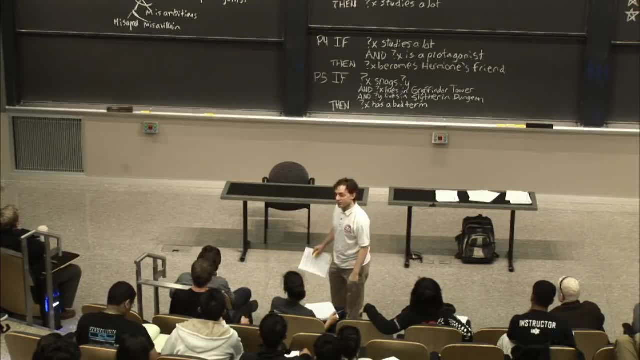 on the right branch, which is a very common mistake. Where do you think we're going to go next? We should go down to see if there's a consequence, for M is. oh, Millicent is a protagonist. Which one of the two? 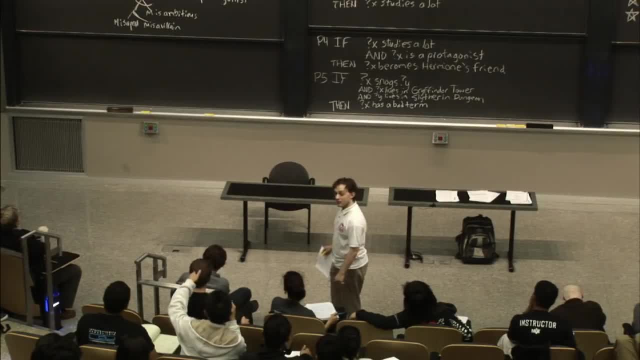 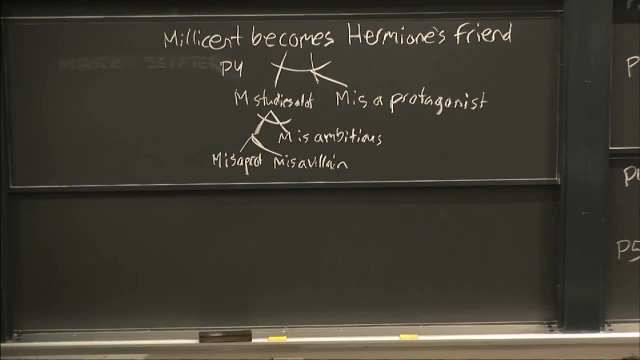 Millicent is a protagonist. do we want to look at? Yeah, the farthest down left, That's right. So you guys will learn depth-first search on Monday, at which point it'll become much clearer what I'm saying. 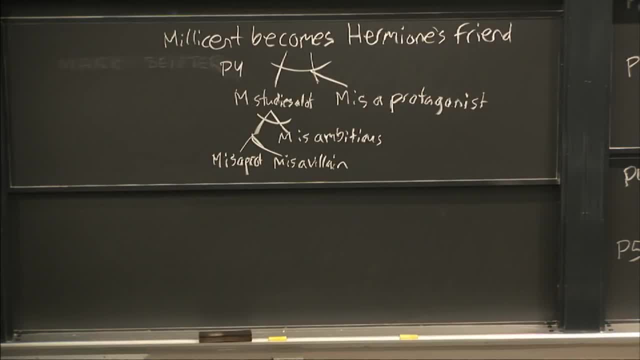 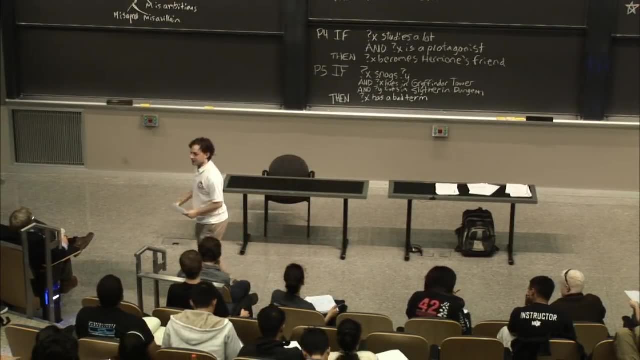 But yeah, you always follow the left branch as far down as you can. Then you take the right branch of that same branch that you followed. All right, Great. So we're going to try to find. Millicent is a protagonist. 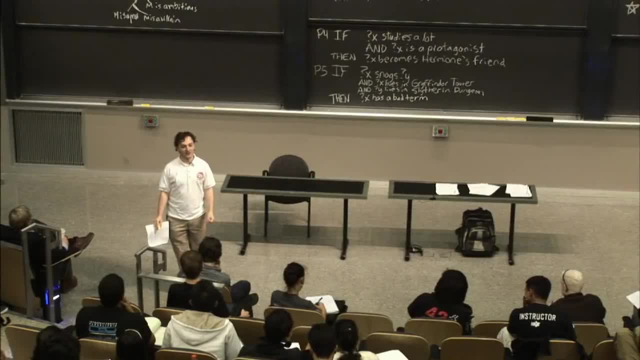 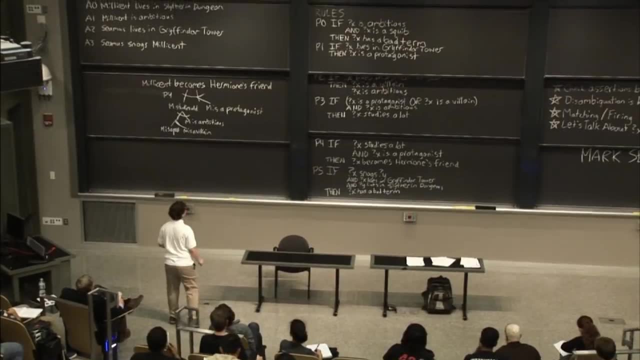 What do we do? first, Everyone Check the assertions. Check the assertions: yes, Is it in there. No, it's not Okay. So, therefore, we're going to try to find a rule, as we heard about whether Millicent 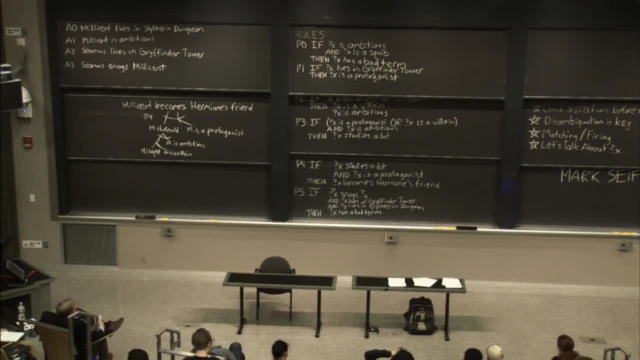 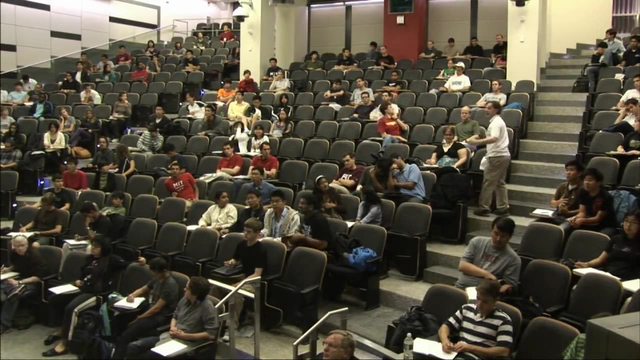 is a protagonist. So, all the way in the back, All the way in the back, Is there a rule that matches, It matches, the, the, the, the matches, and it's consequent that Millicent is a protagonist. Um, 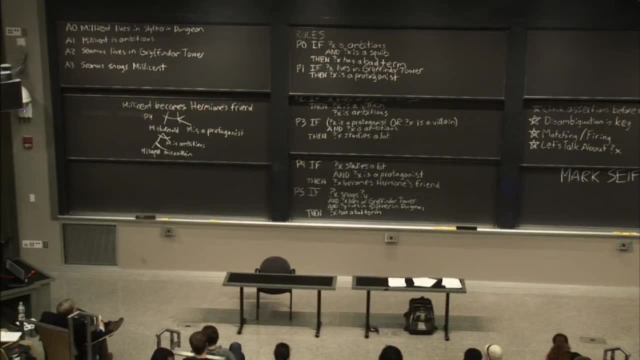 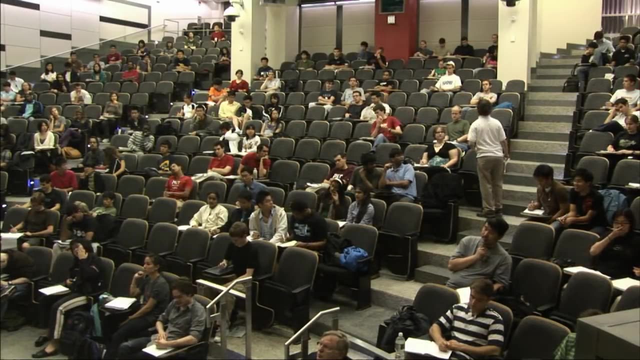 there is a rule that matches. Okay, Well, let's give it a try. Which one Rule? one? Rule one, That's right. So therefore, we have to add what to our goal tree? Um, another leaf, Right? 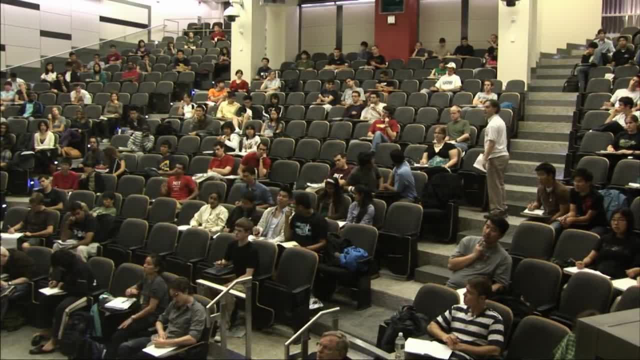 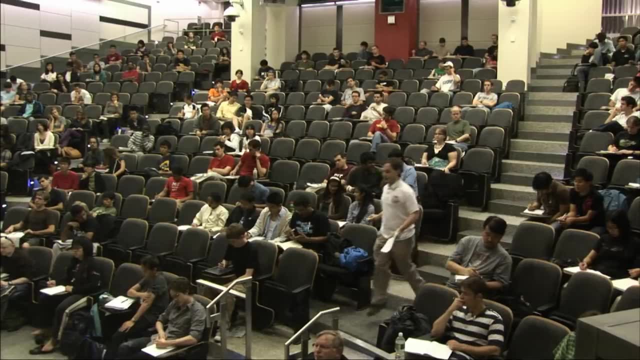 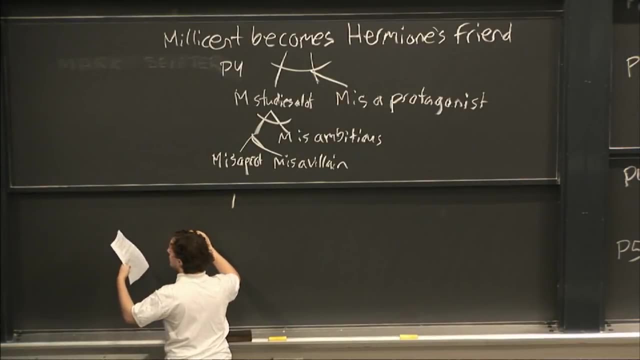 And what's on that leaf? Um, it's explicit original: Yeah, Millicent lives in Grimindor Tower, Perfect. So our new thing that we're searching for is pretend this connects. Actually, I guess it does connect. 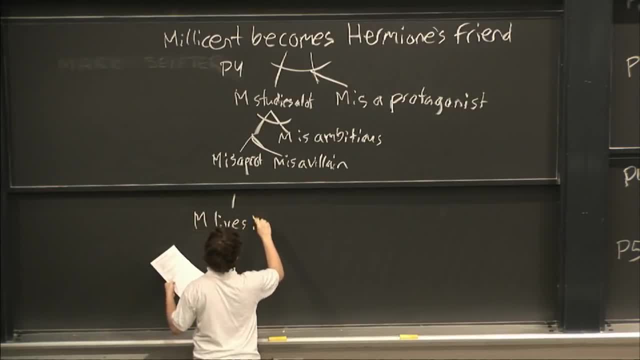 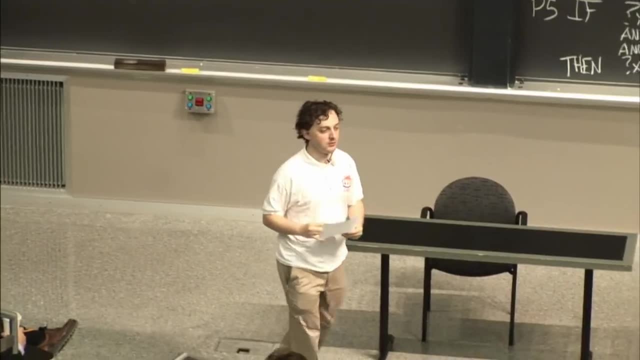 We're looking for. M lives in Gryffindor Tower. Great, All right. And since it's step first, that's where we're going next. Great, We're on a roll. So what do we do first? Do we have? 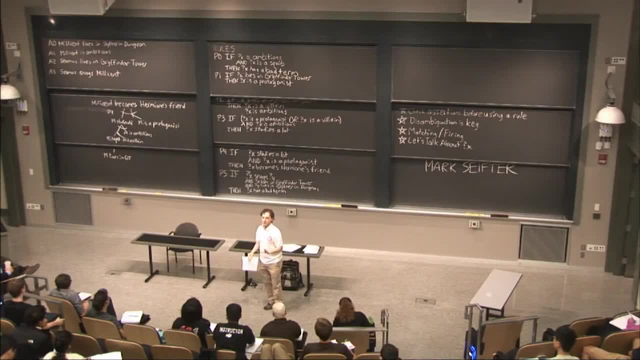 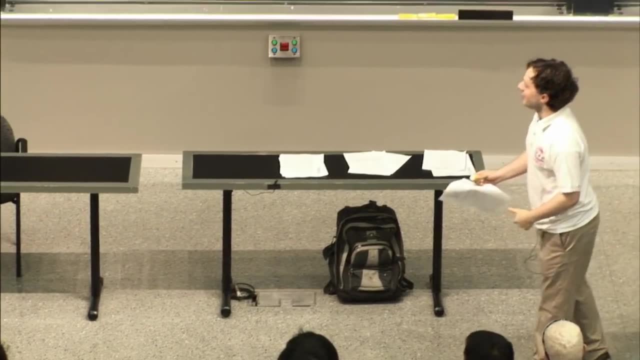 that in assertions Some people say yes, but the answer is no. We have, in fact, Seamus living in Grimindor Tower. Most of you said no, You're right, The majority rules. Uh, we don't have it in the. 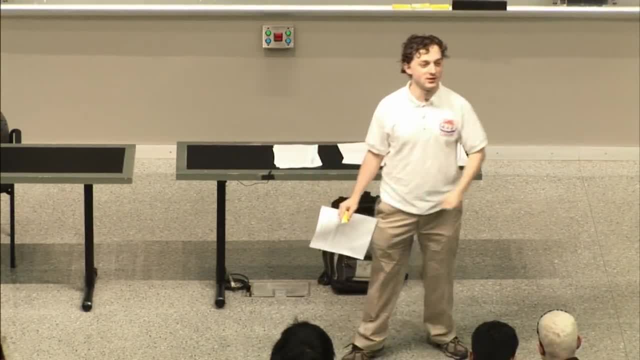 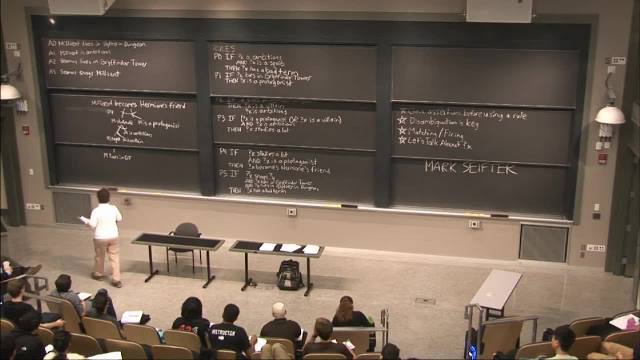 assertions. However, do we have a rule with that in the consequent No. So what do we do? People are saying different things that are all correct. Backtrack. you say: Go to the next. We can't prove it. 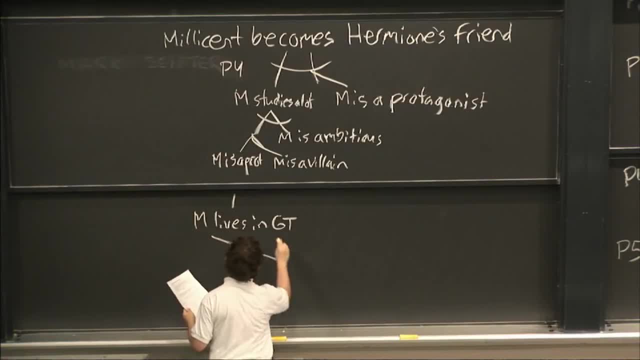 All correct, Put a big X. This isn't true. Now we look up, We're on an or node so, but we're not done yet, because either of those can be true Great. So now we go back. 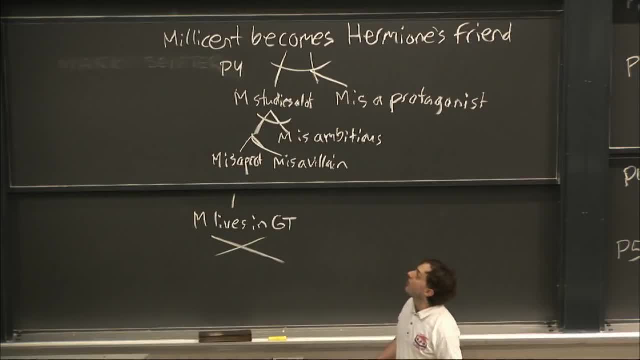 up backtrack. Millicent is a villain- Great. What do we do? first Check the assertions. Is it in there? No, it's not. Don't worry, We're getting to one where it will be. We're about. 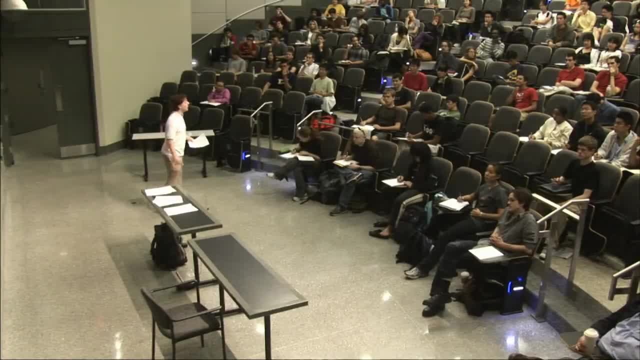 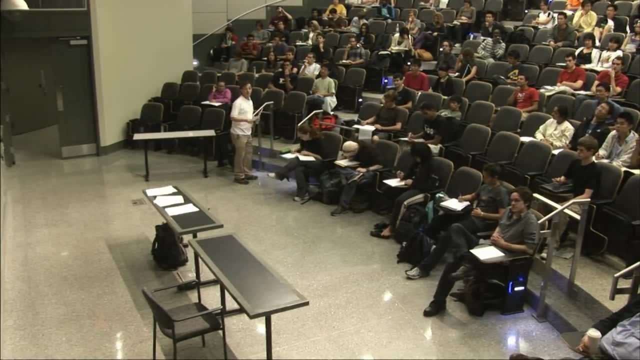 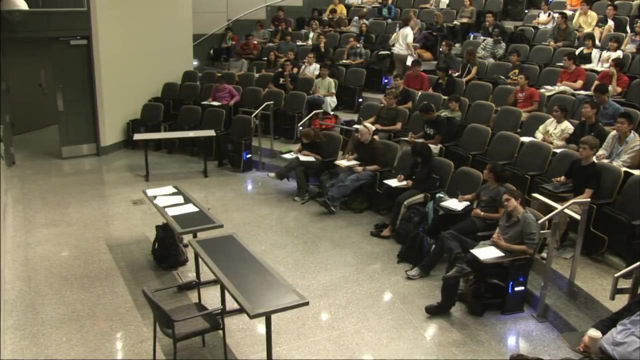 30 to 40% of the class. last points: Very, very soon. So we see that Millicent is a villain and it's not in the assertions. So therefore, is there any rule that has that in its consequence? 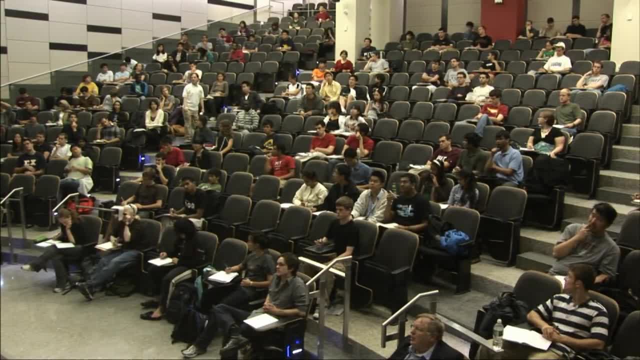 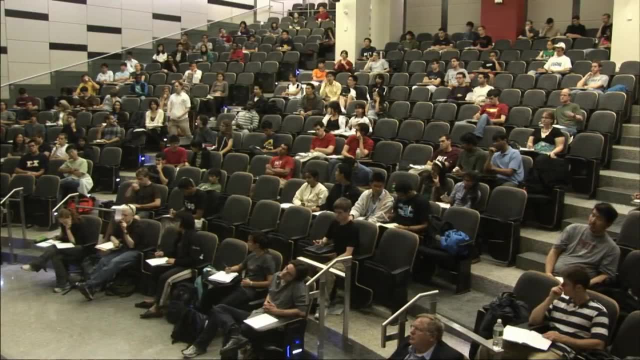 We're looking for. Millicent is a villain, Right? Well, we have. I can't see it All. right, I will move it down slightly because I have a little bit off kilter when I put in the parentheses around the end. 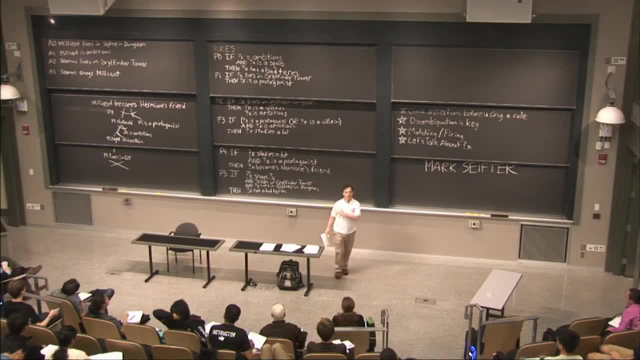 Hold on, There you go. Okay, Is it a protagonist or is it a villain and vicious? Then they study a lot. All right, We're trying to prove that she's a villain, though. So do we have any with that in the? 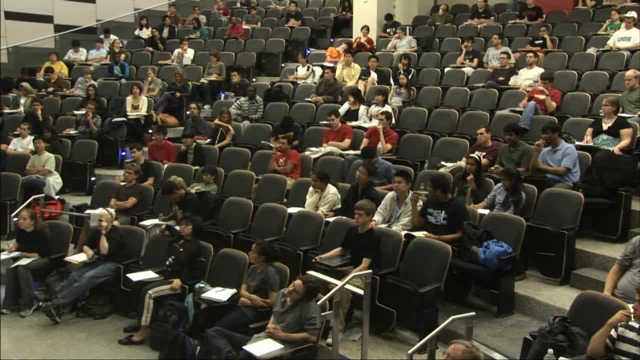 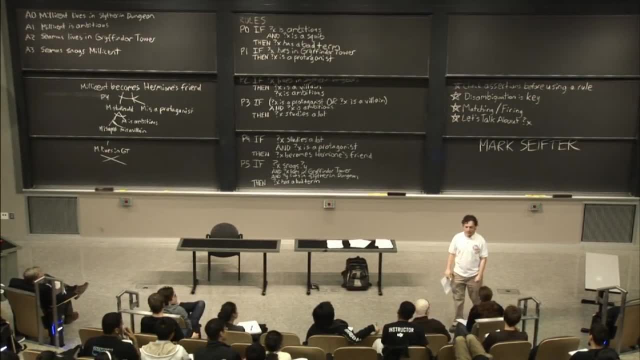 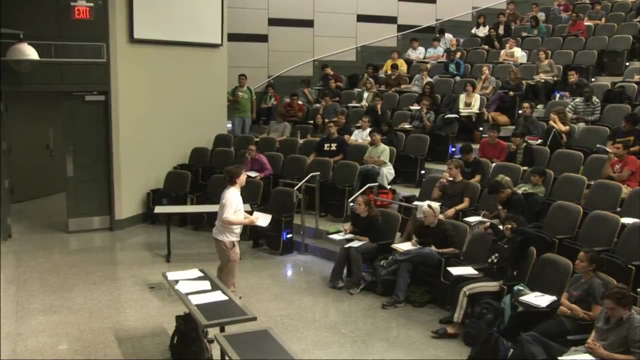 consequence: Anything that will prove that she's a villain if we fire off that rule. All right, Want to give her a little bit of help. Ah, see that It had two, so it was a little bit harder. Now, some people. 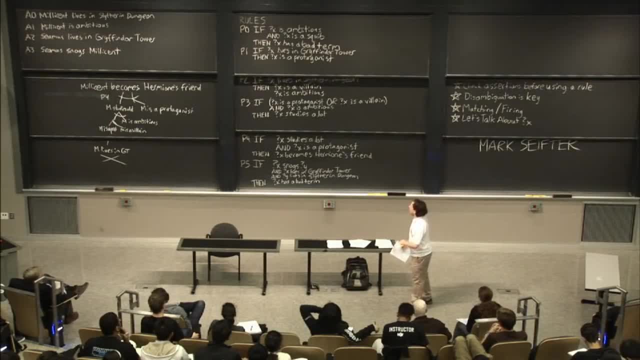 ask: what about that ambitious thing? Can we like add that to the tree or something? No, The backward chainer is single minded, focused and stupid. Even though it's later going to need to prove that she's ambitious, it doesn't. 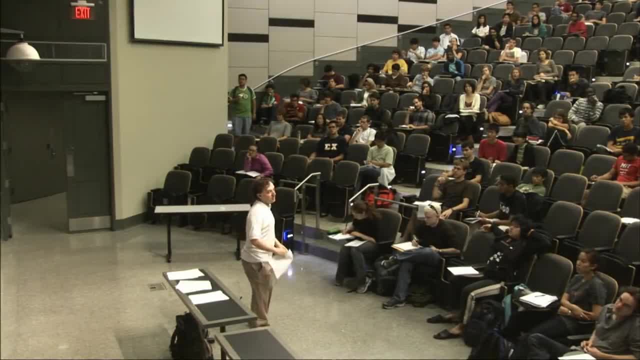 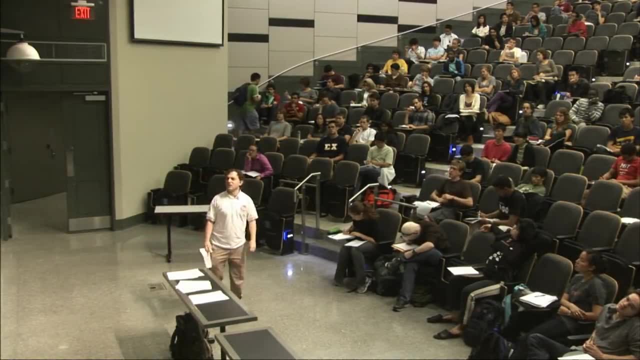 care, It just sees the villain there. Villain, oh, that's great, As long as we've got the antecedent we are going to. This is actually an important point, not in this particular problem, but in some other problems. 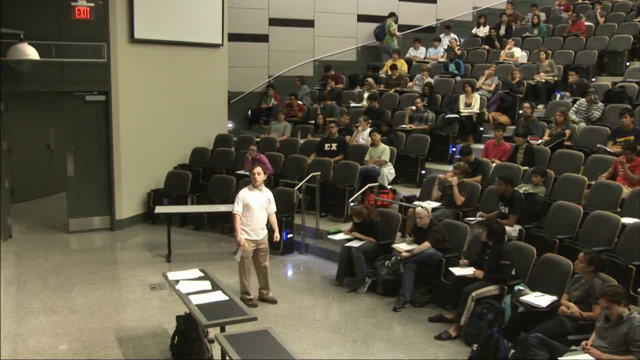 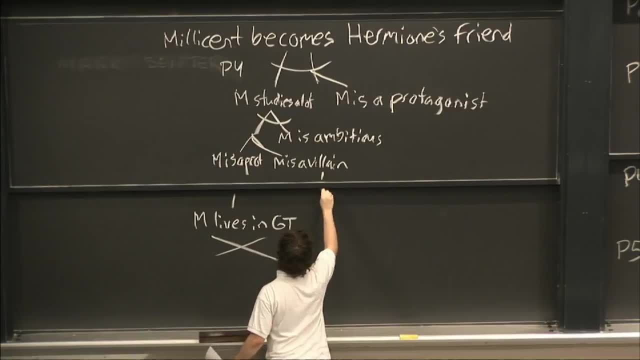 So by using P2, we're obviously going to have the antecedent X lives in Slytherin dungeon when X here is Millicent. So Millicent lives in Slytherin dungeon, All right. So 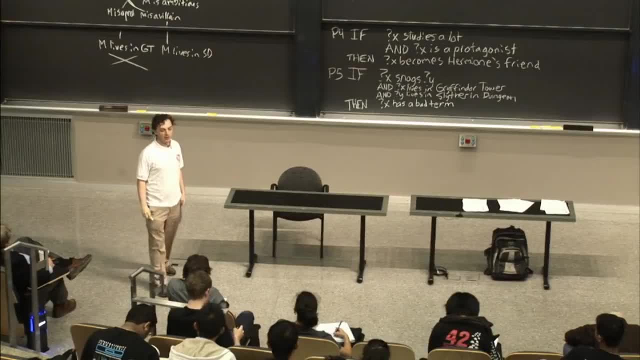 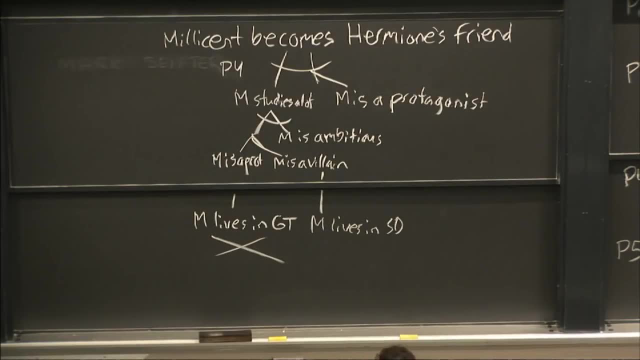 what's the first thing we do when we see this new assertion? We check the assertions. Is it in there? Yes, That's not where everyone lost points, but yes, it is in there. Check This order. node is happy Now. 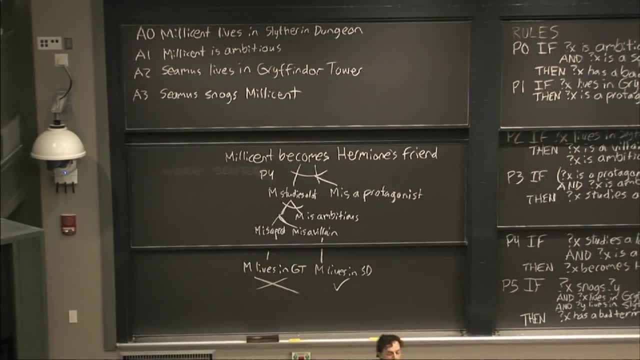 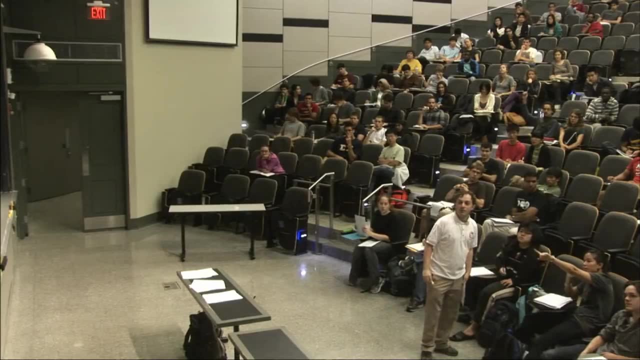 we move up to the and node with: Millicent is ambitious. So Millicent is ambitious. What do we do now? I have a second question. Oh sure, Ask a question. So, in the consequence of P2,, 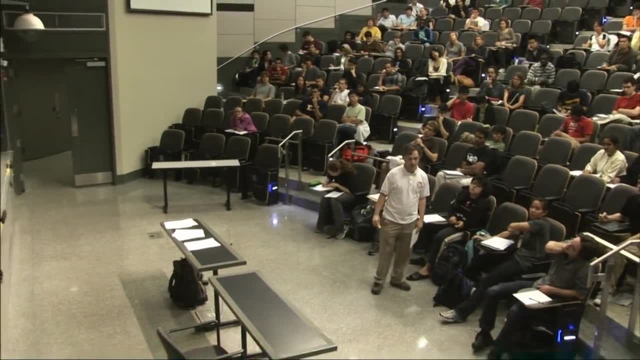 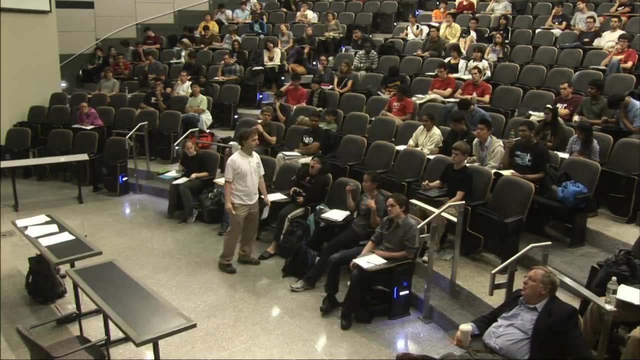 we know that X is a villain and X is ambitious Like I don't know if it's like luck or whatever, but in our assertion do we have that Millicent is ambitious. Is that necessary to let us use rule 2?? 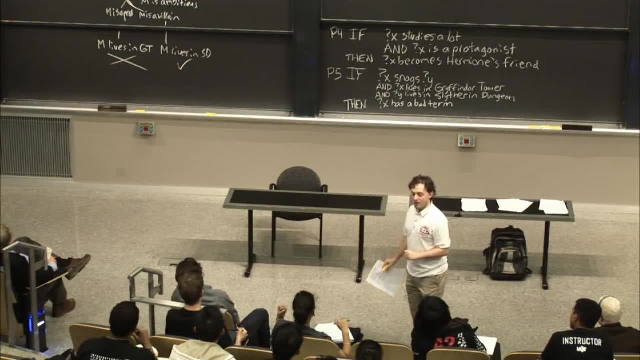 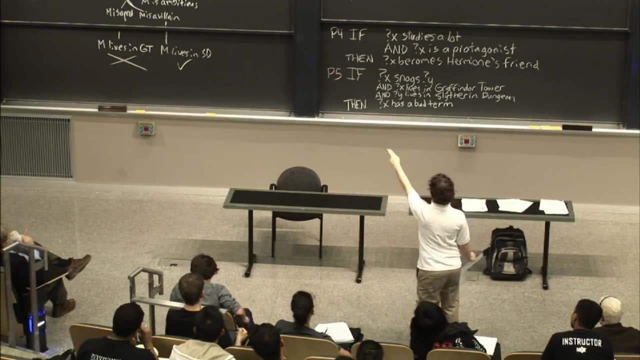 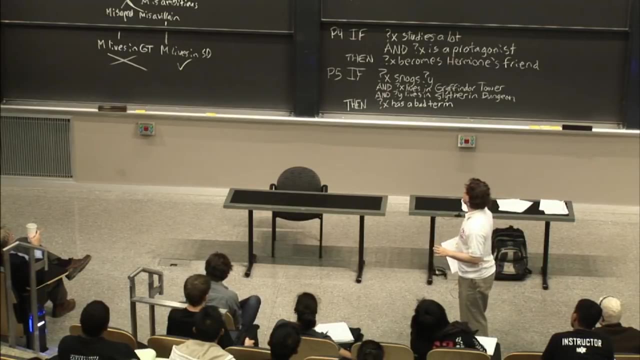 Actually no. The question is: do we need the X is ambitious to be in our list of assertions in order to use P2?? For instance, if we didn't have the assertion that Millicent is ambitious, would P2 have a? 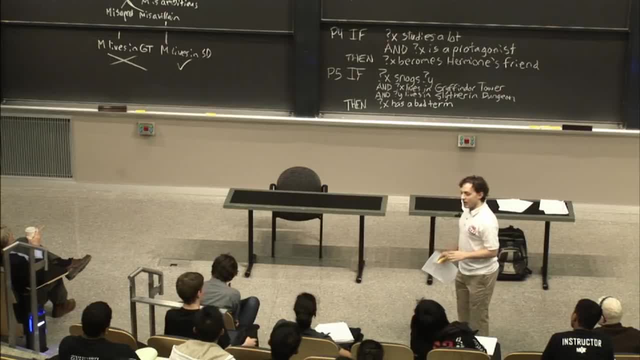 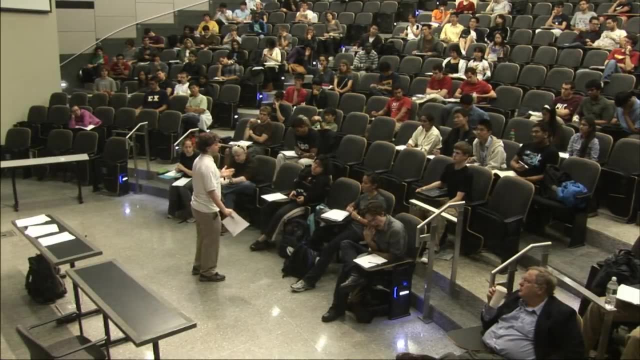 problem firing. So it's a very interesting question. It's sort of what actually I was trying to mention earlier when I said it's single-minded, it's focused, it doesn't care about the other one, Because you might say well, 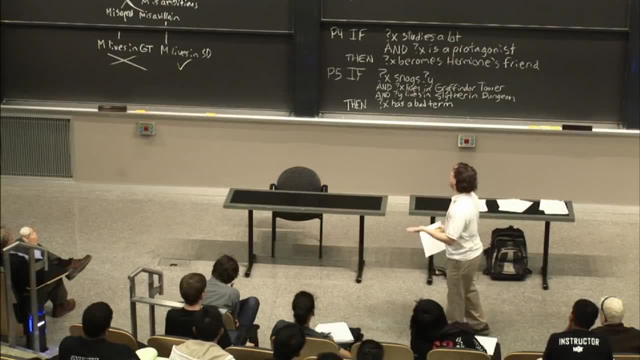 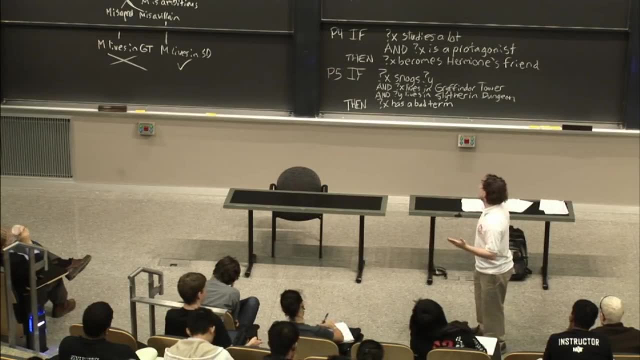 wait a minute. P2 could never have actually fired if it didn't have both of its consequences. But in fact the backward trainer doesn't care. All that the backward trainer is looking to do is to prove whether or not there's a 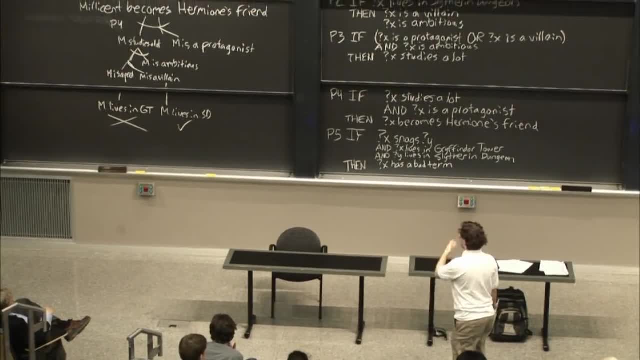 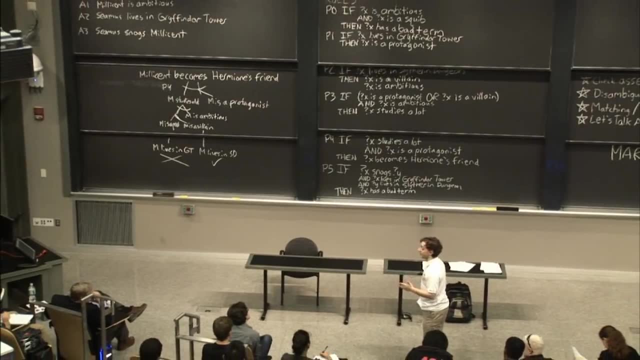 possibility that Millicent might be a villain. It's not trying to of some. certain rules are making Millicent a villain and all the other things that are there, like ambitious, are in the database. It's not the forward trainer It. 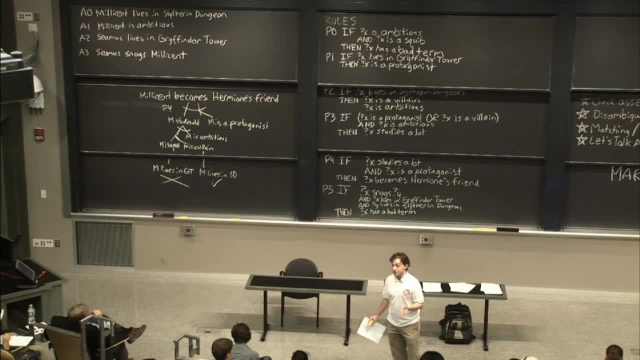 actually doesn't care. This sometimes leads to unnecessary computation, but it's very simple and it's very simple to code, So it often will probably speed you up in the long run, Like if there's, for instance, 100 things in the. 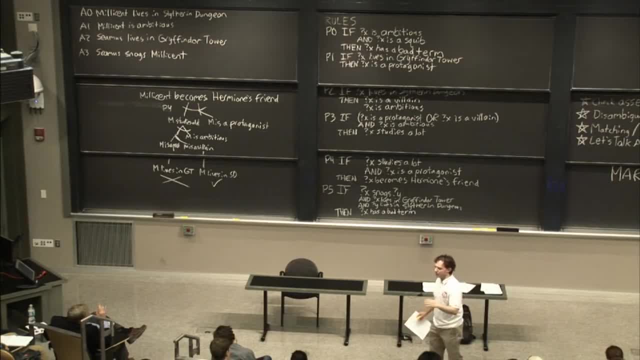 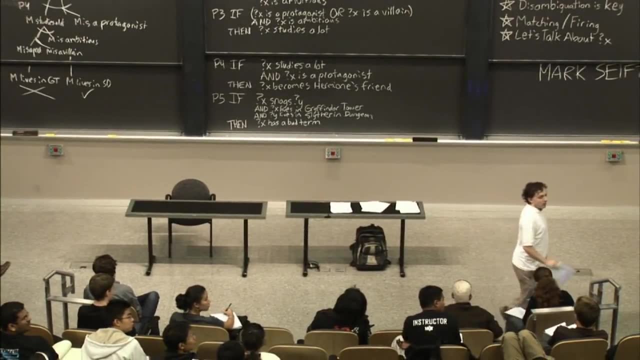 then, and you only care about one of them. it would be a waste almost to add those 99. There was a follow-up over here somewhere. You still have to walk the whole line as well. You have to walk order n of the 99,. 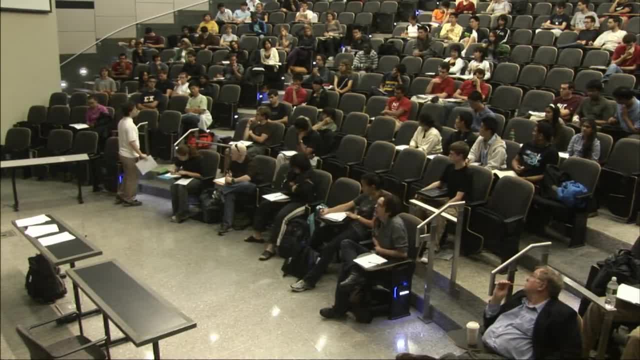 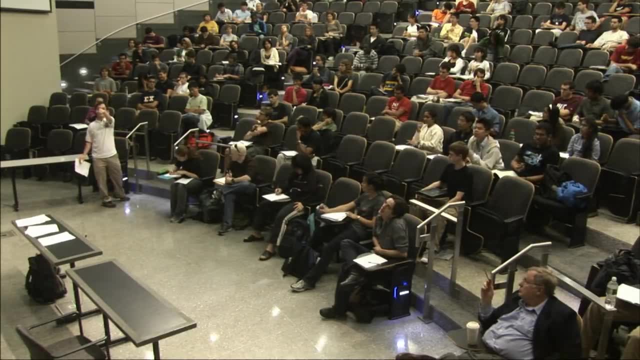 and so then you're doing an order n computation and you add all n of them to some hash table. You can try. However, then at that point, every time you check the assertions, you'd be attempting to check those 99. Also. 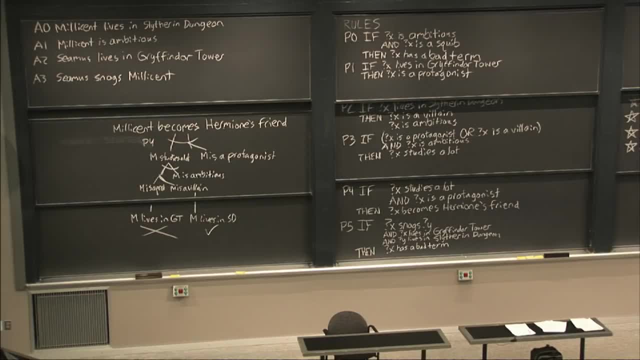 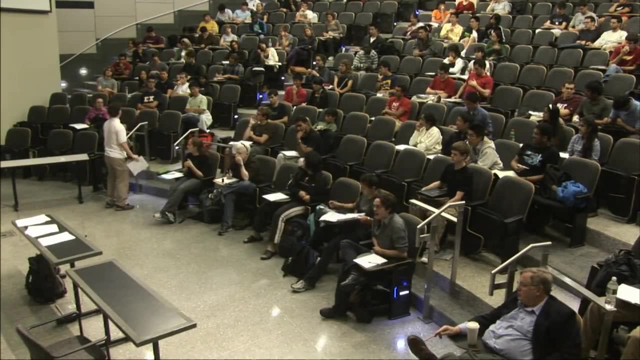 you might not have used those rules. The question is: could you make a hash table with all of the 100 things that were in the consequent And then, after having made that hash table, since you were already walking through those anyway- when you? 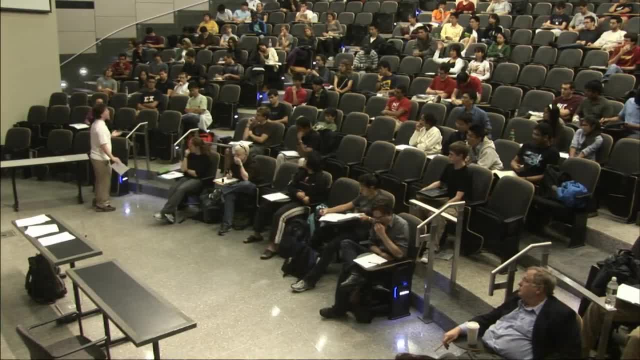 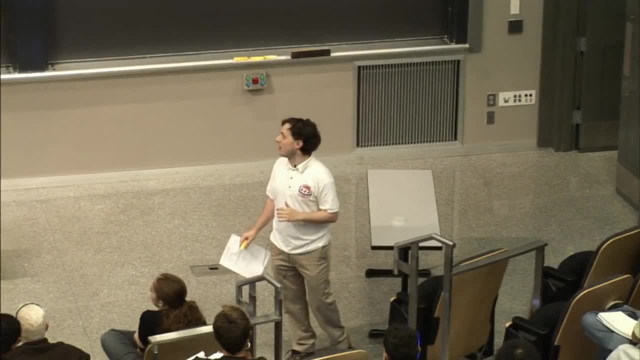 were checking it, you could add those to the assertions. The problem is that you might not necessarily want all those with the backward chain, or you might not necessarily want to think that all those things in the consequent are necessarily true. However, 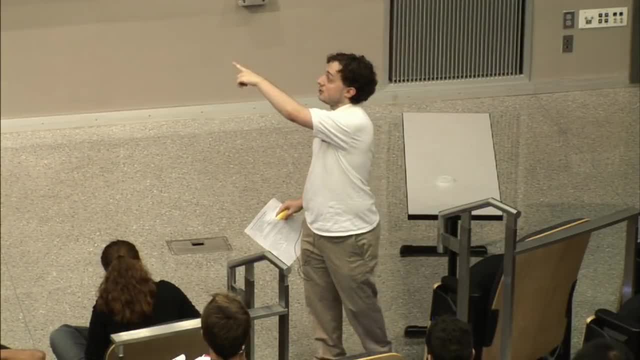 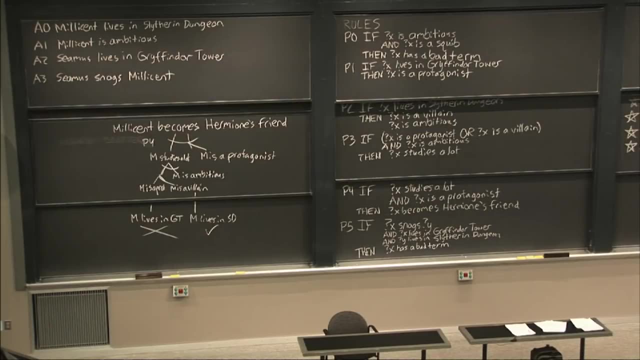 you might not care about them. And then you have to make in order n computation. every time you check that list of assertions in the upper left, That's true. However, you don't know what assertions there are. You have to check. 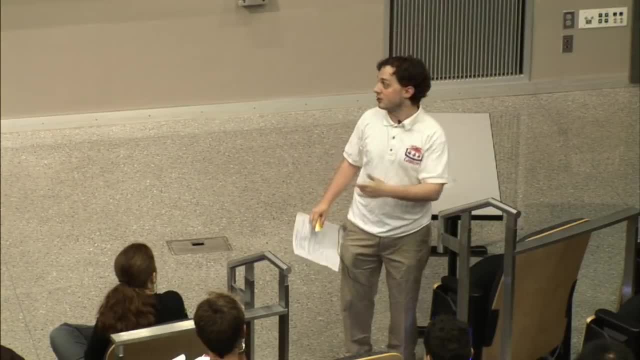 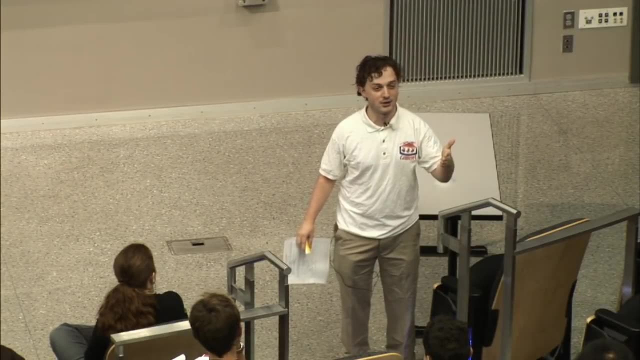 the entire list of assertions in the upper left every time you get to a new node in the goal tree. So each one is order one. but I'm not saying to find a specific assertion is order n, I'm saying every time you make a. 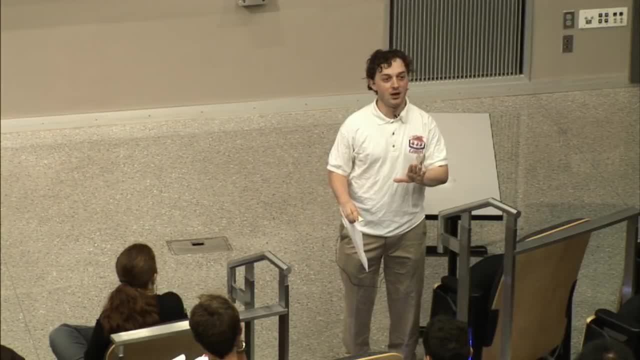 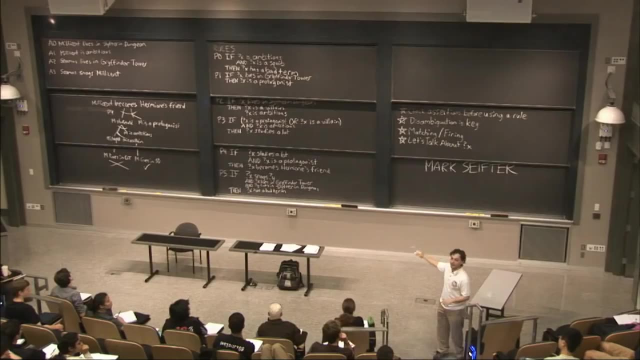 new node in the goal tree. you have to check all of the assertions you've added. Yeah, let's check the four, but let's say that there were 10,000 consequences of P2. You would have to check 10,000. 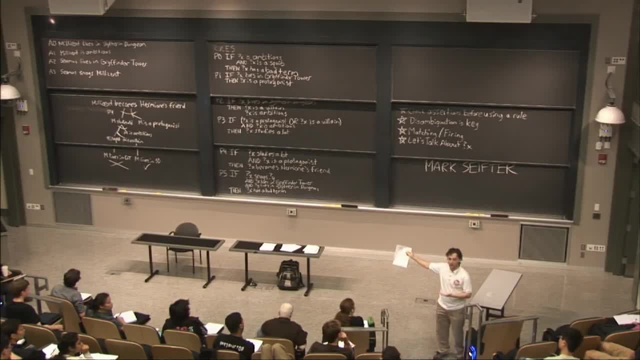 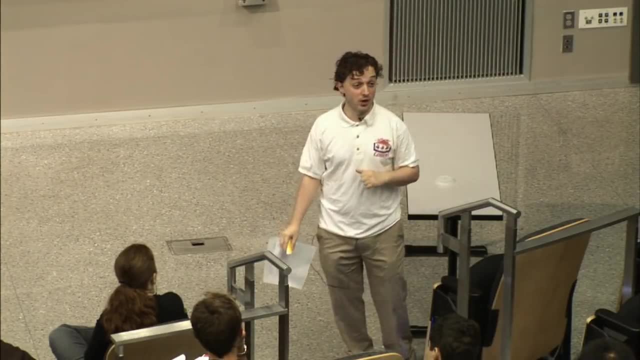 instead of four if you added them all after proving P2 was true on the goal tree. Also, another important note is that you might not use every branch of the goal tree if there's an or that's up higher and you wind up using a. different branch, in which case you probably have to make a separate hash table for every sub-branch that you have and then remember which hash tables were updated based on which sub-branch, and then the sub-branches die. It's probably more effort. 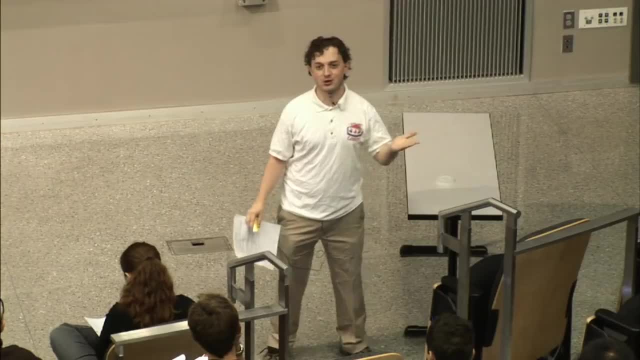 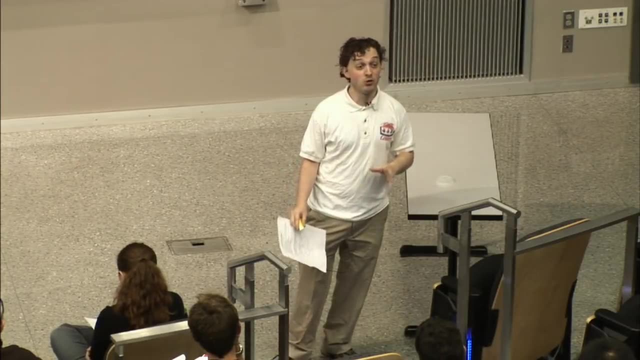 than it's worth. It's certainly an interesting question. It's a great question for debate and recitation and also I'm happy to talk about it later. I think that someone who very intelligently made hash tables and thought the problem through. 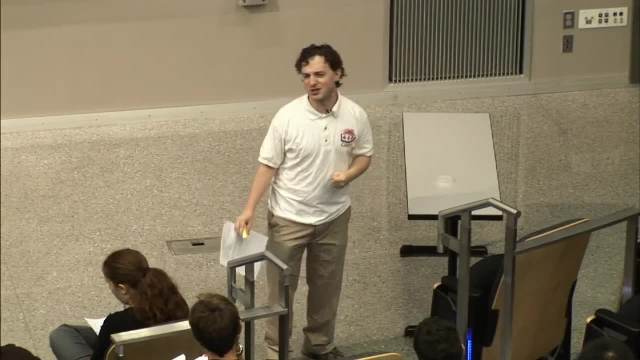 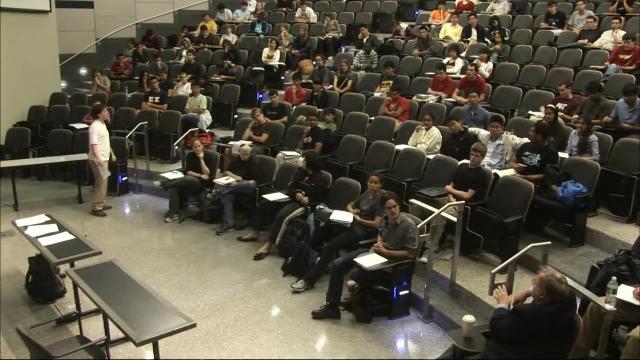 as Patrick said, more knowledge can mean a better search, because we haven't done that lecture yet. You're talking about implementation decision, and using hash table might well be a good way to do this. The problem is that we're presuming some things about. 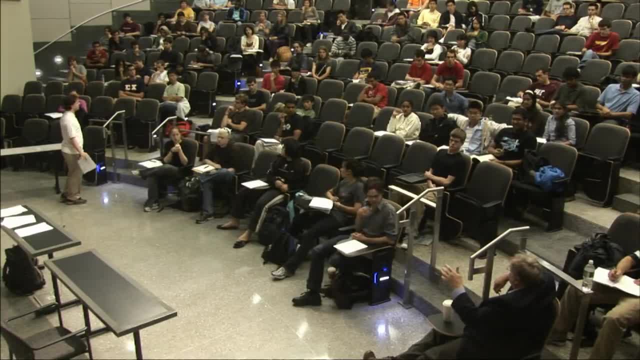 how the rules are firing and what bindings they're firing. that depend on the order of the assertions in the table. So if we use the hash table, we'd lose the order and we wouldn't be able to create a homework. That's true. 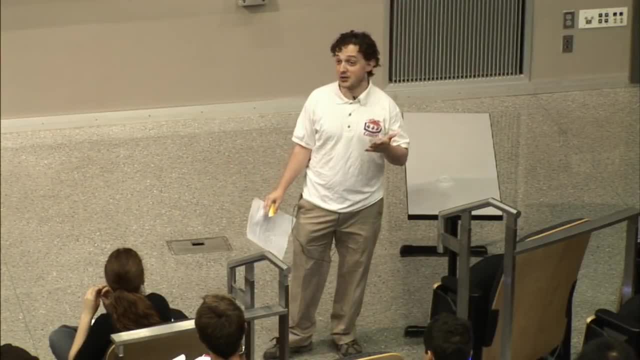 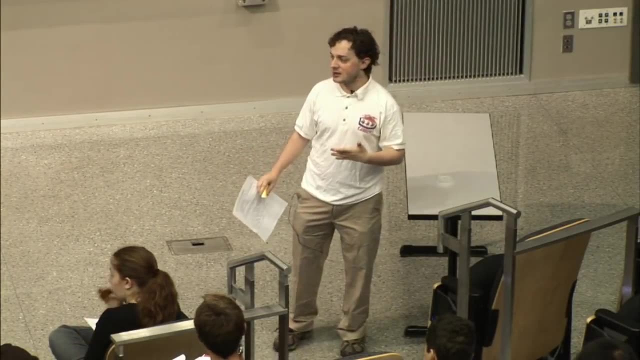 That's true, but I'm thinking, if someone wanted to make that implementation, as do some research in rules-based systems. it's possible you can increase the running speed In this class. we are not completely as focused on the fastest algorithms, but I 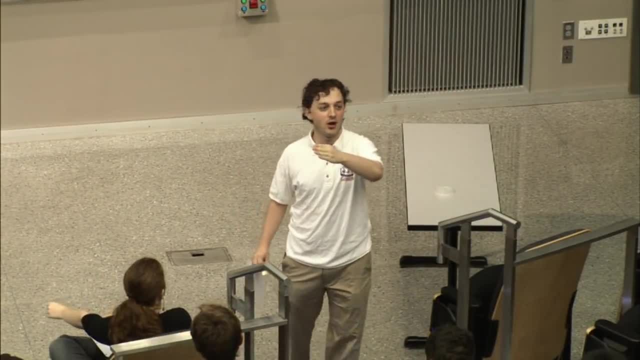 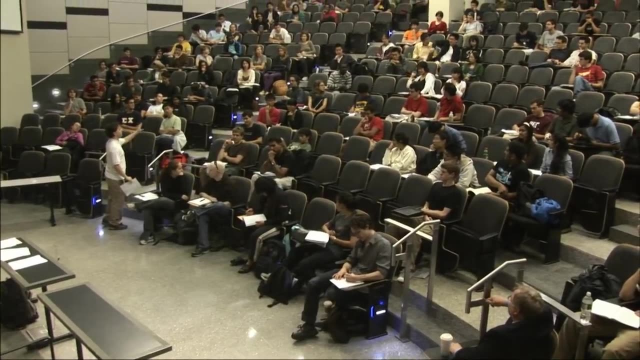 still think that's a cool thing to try Questions from people in the crowd. I'll start here. So ignoring the hash table thing. Ignore the hash table thing. That's a good idea because it's a little extra enrichment thing It's. 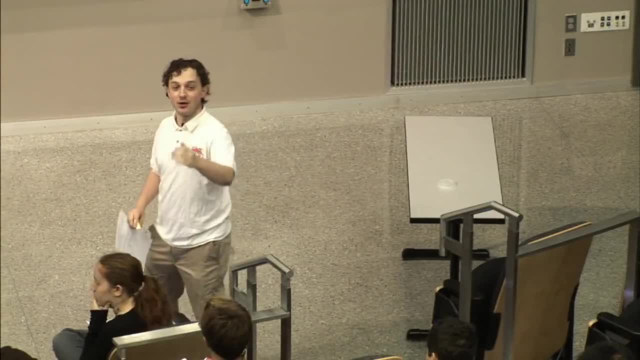 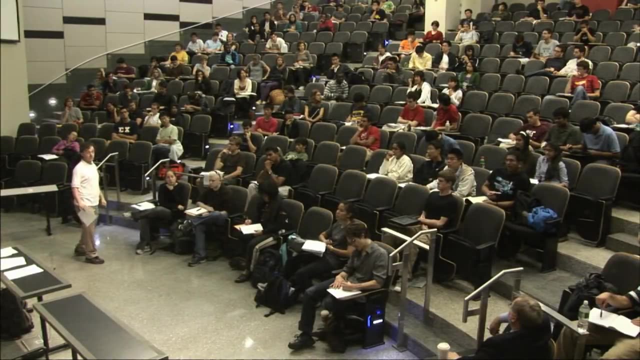 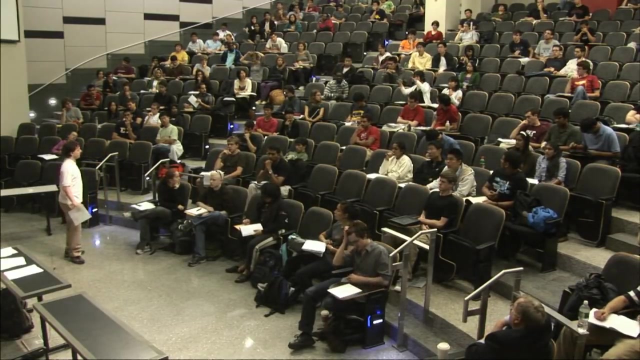 not anything you would possibly need to know for the quiz. So if it became like an event and you're using this, then statement because you want the villain. So along with using this, you get X is ambitious. What happens if you use after that? 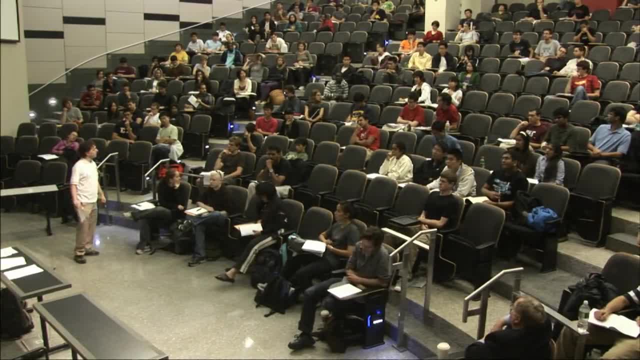 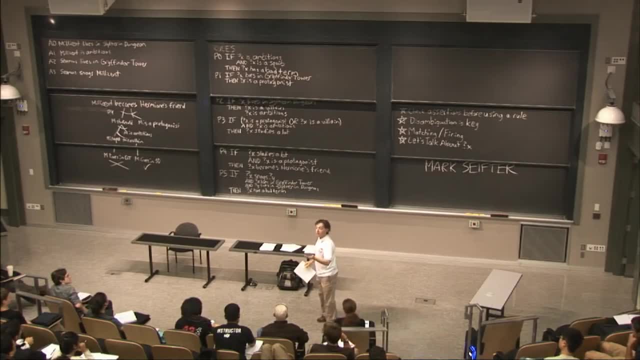 another. then statement that you also need that says X is not ambitious. So how would you resolve that? So the question is: let's say you used rule two somewhere in the tree to get that X is a villain. Then later you have X is. 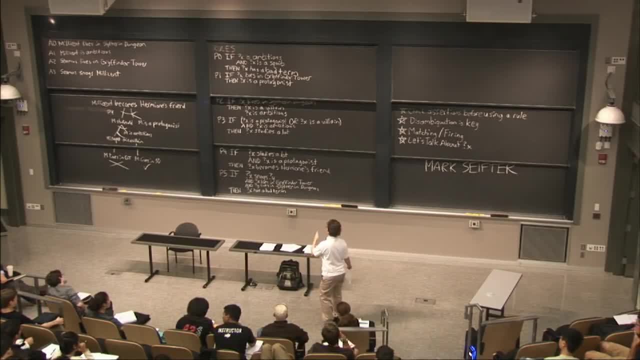 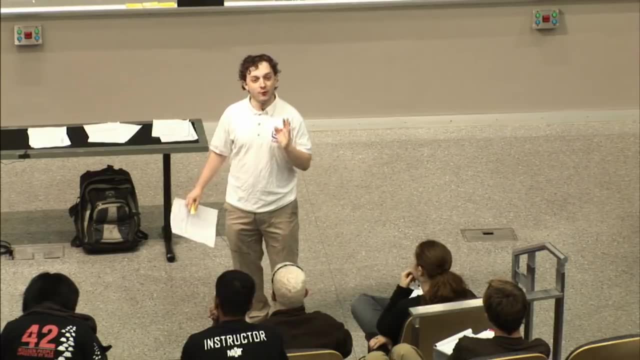 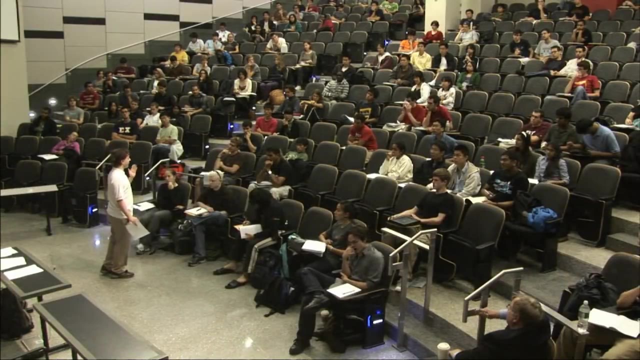 not ambitious somewhere in one of the other rules that you then later need? The question is: how do you resolve that? What does it do? First of all, interestingly, if it says X is not ambitious, literally like that, and I'm. 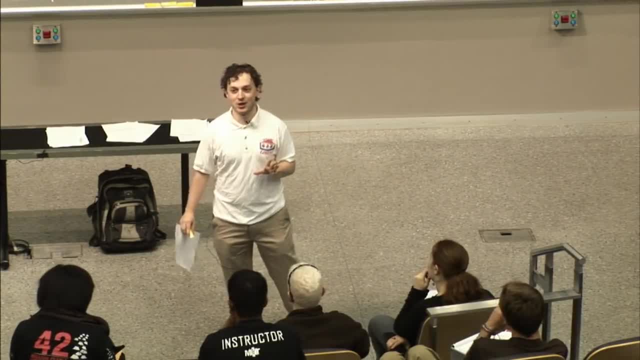 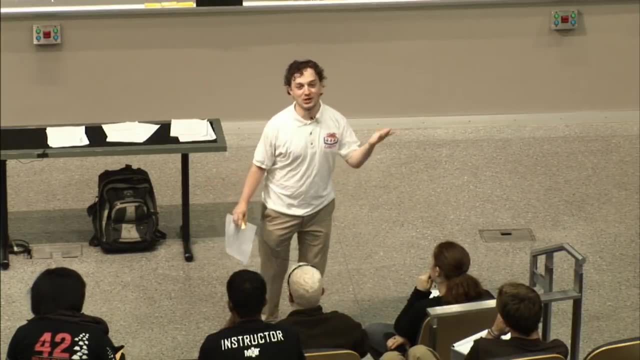 not being pedantic here. this is one of the tricks someone played in a previous quiz. you can have that, and X is ambitious both in the list, because it's a dumb rules based system that doesn't know that you can't have both of those. 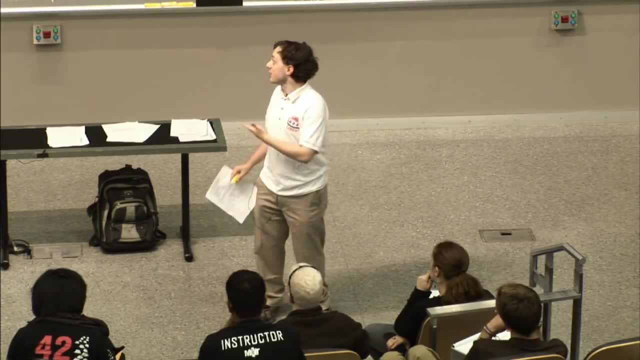 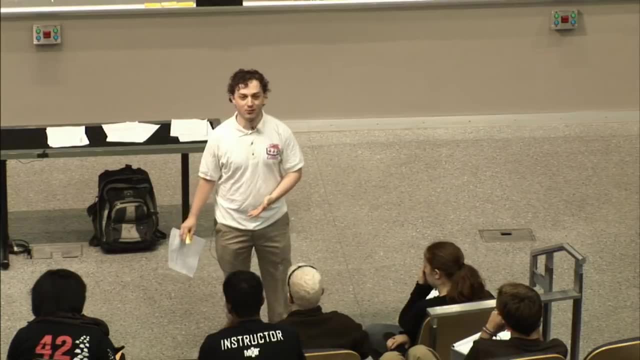 on the list. So if you have a positive assertion in a consequence, X is not ambitious, it'll be happy to add: Millicent is not ambitious. and while Millicent is already there, because it's stupid, Now if it had, delete Millicent. 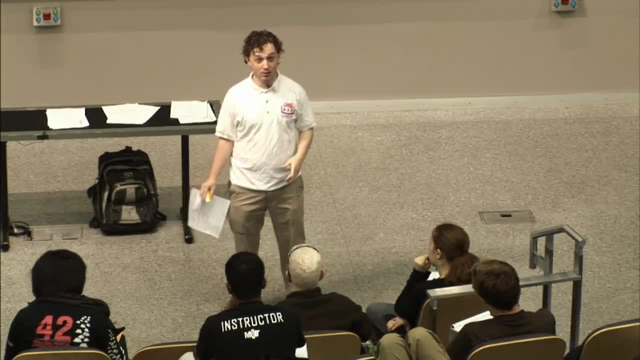 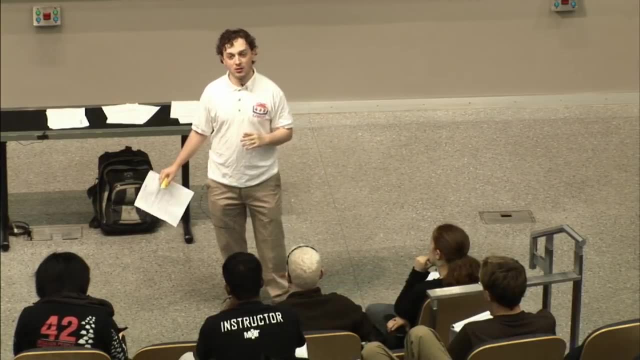 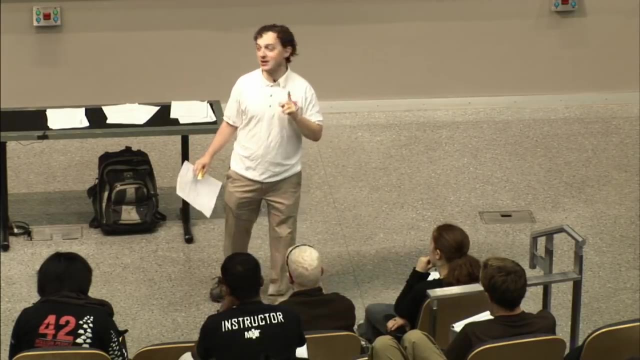 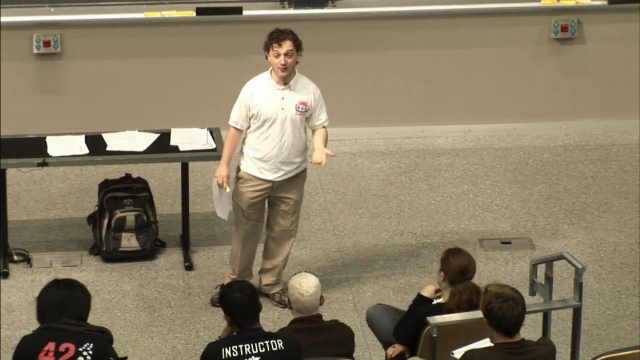 as ambitious in the consequent and deleted something that was previously there. that would probably make the mistake of allowing this. However, this is exactly why we do not have delete statements on the quizzes. At least previous quizzes did not have them, except for in. 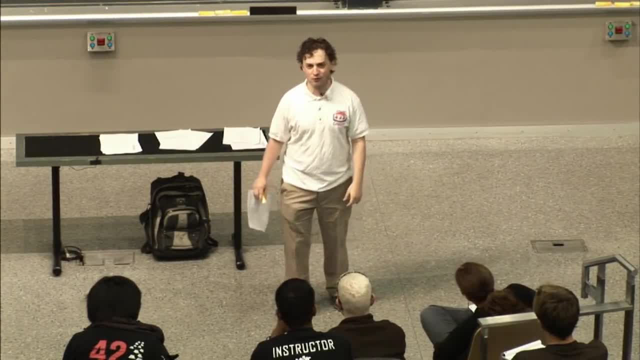 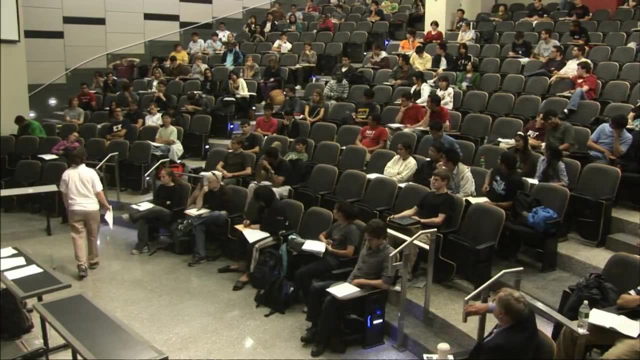 a hypothetical of what happens if we had a delete statement here. I don't think we've ever made people work things through with the delete. Delete would possibly cause some issues Question in the back. So just to check this we're doing backward. 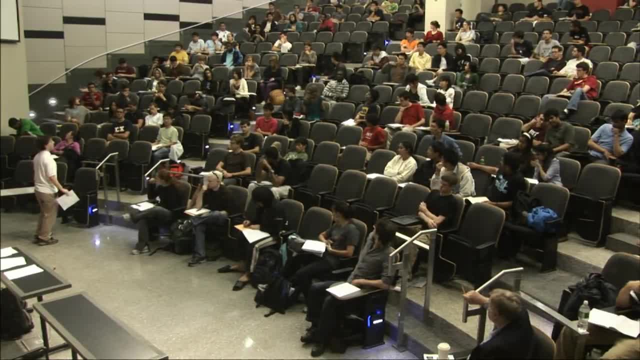 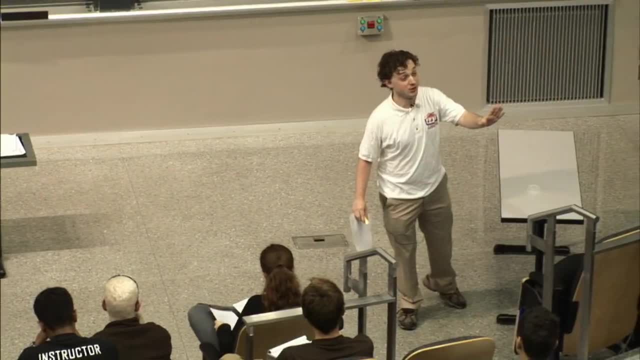 chaining and we don't actually add assertions to your assertions. Never add assertions and backward chaining to the assertion table. It's dumb, The system is dumb. I'm not saying it's a dumb idea to do this. It's actually pretty fast to. 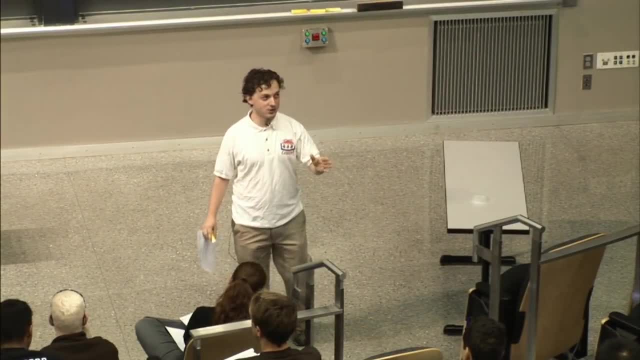 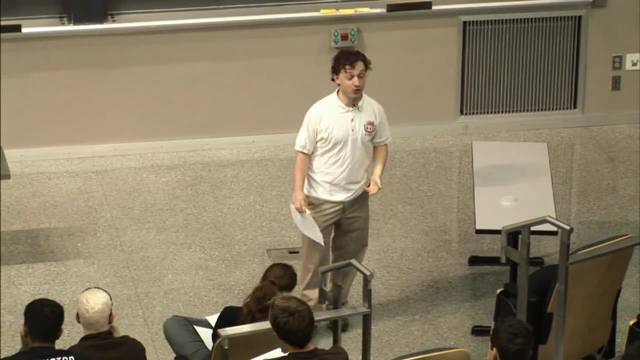 do it this way, But the system is dumb. So the question is: do you add assertions or you don't add assertions or you do not. You simply go through checking all the things in your goal tree until the goal tree is either proven or disproven. 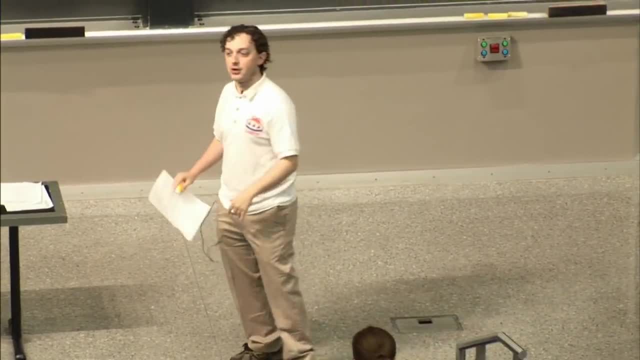 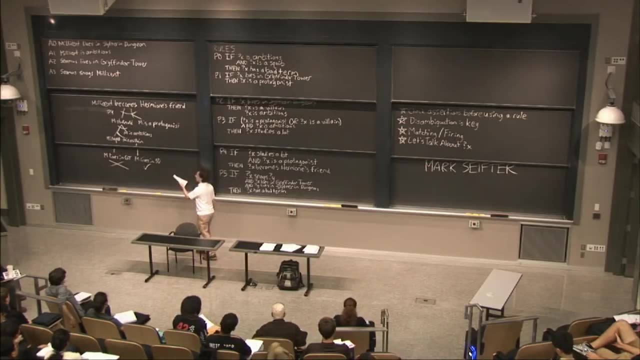 then you are out of here. All right. So cool so far. everyone, Good questions from everyone. These are all questions that are things that often trip people up. So our next thing is ambitious. We sort of the cat is out of the bag. 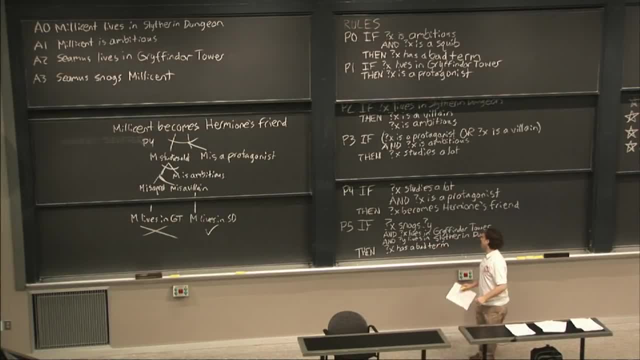 because there was a question mentioning that there was an assertion that says that. But I direct you guys to our favorite rule, rule two. Shouldn't we use rule two to prove that Millicent is ambitious? The answer is: if you want to. 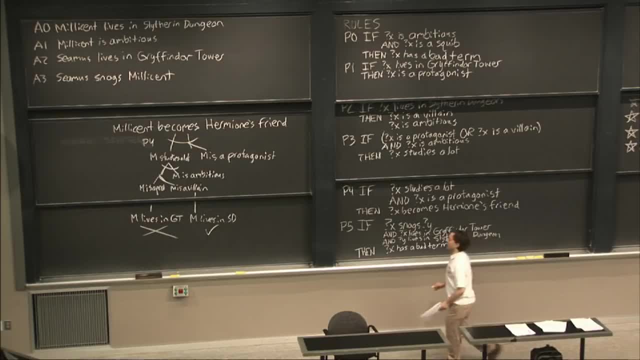 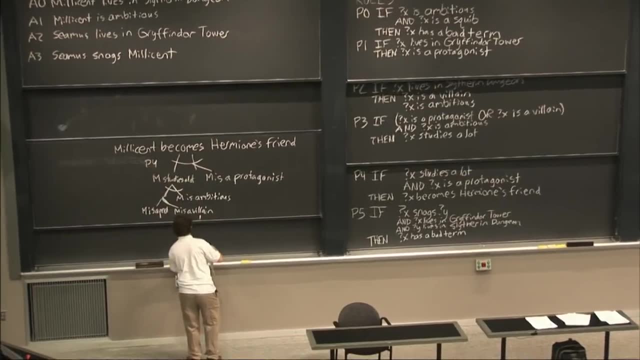 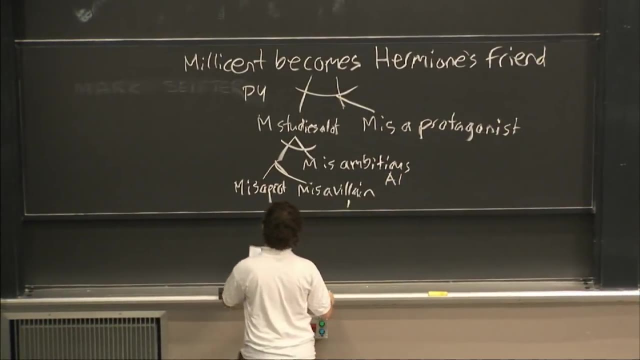 lose four points, or however many points, then yes, But if you don't want to lose points, then this is already correct by virtue of assertion one. So I guess I should write also that this over here, Millicent studies a lot. rule is this rule. 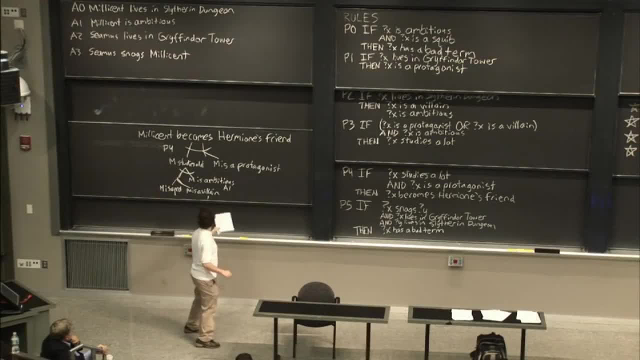 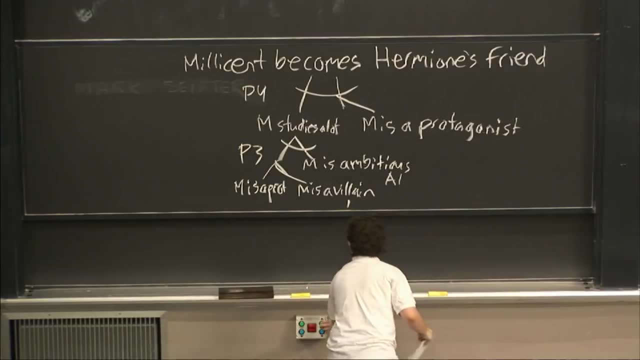 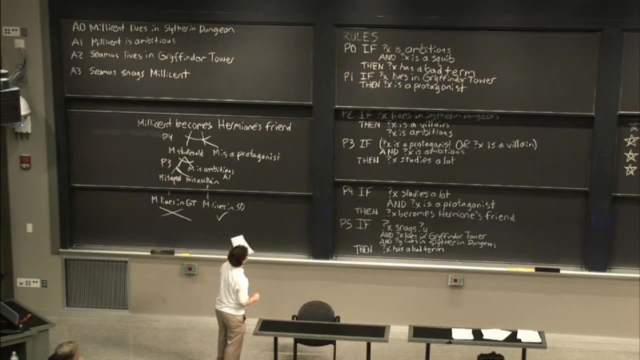 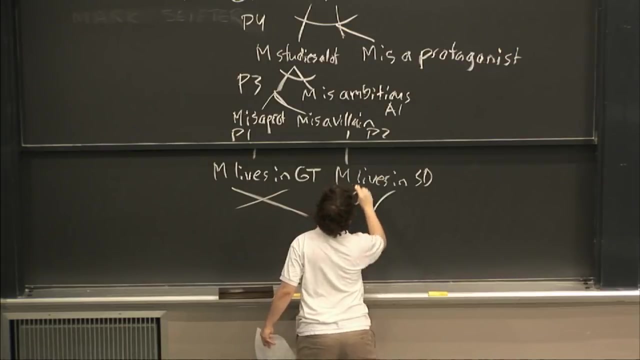 is rule four, down here, to prove that she studies a lot, is rule three. and then, at the bottom, here we have, what rules? here we have the protagonist rule, which is one, and the villain rule, which is two. This is correct virtue of a zero. Okay. 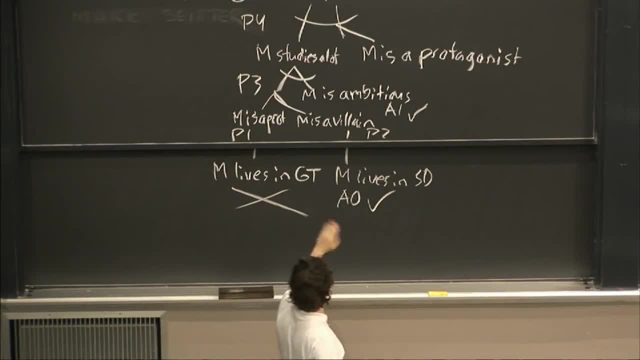 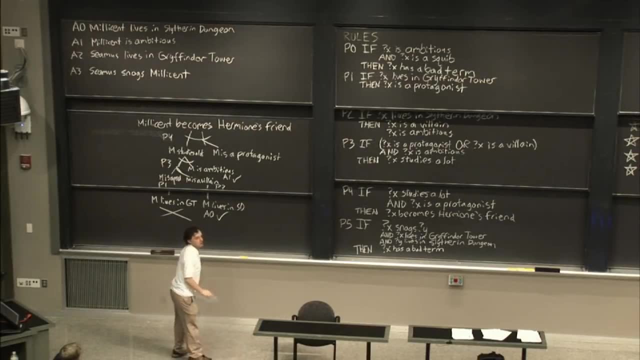 Great, So we've proved this whole end node. We know that Millicent studies a lot, But now we're going to have to go a little bit more quickly based on time, and so I will do the remaining things. anyone who has not been 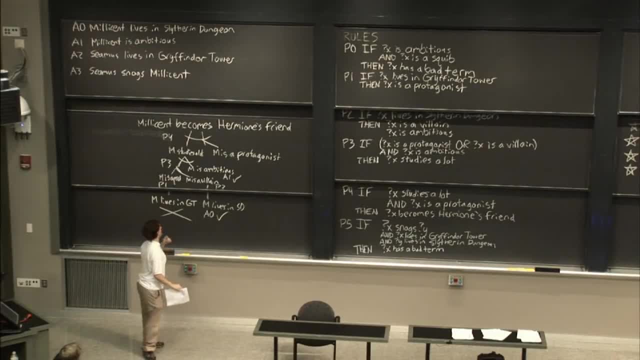 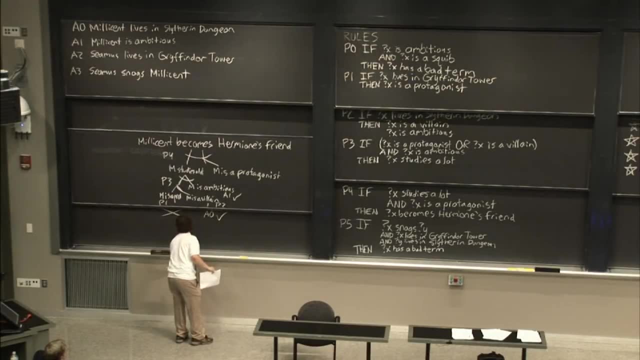 called on is off the hook, but that there's some interesting stuff still to come. So Millicent is a protagonist. Well, good news everyone. There's one other reason that I can do this, and that's that you've already told me what I 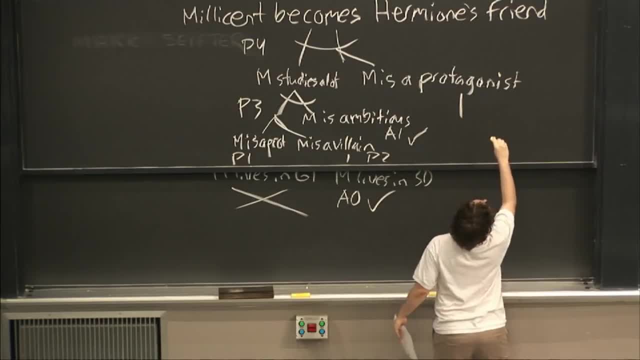 need to do. Millicent is a protagonist. you use rule one and check if she lives in Gryffindor Tower. Now will it do it again? Yes, it will. It hasn't cached that. it's already tried that. Now a hash. 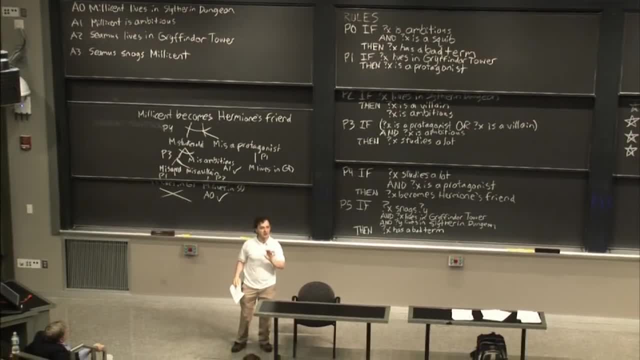 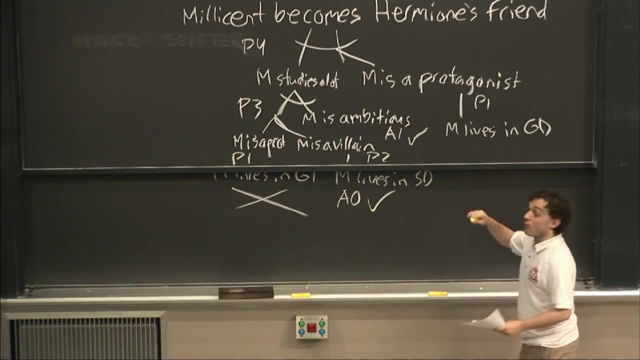 table. not withstanding, caching something you've already tried may be a good idea with backward chaining, but we do not do that in this class. That's an implementation detail. it's another idea of something you can do. We don't cache things that we've 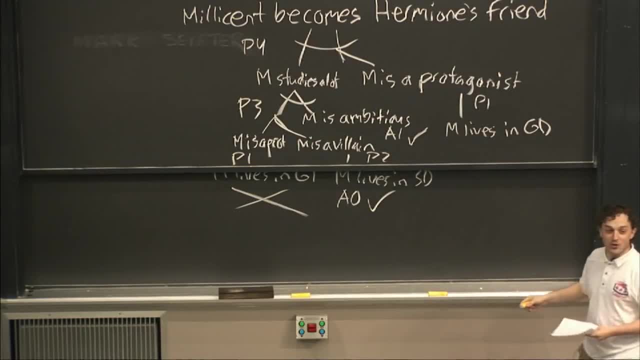 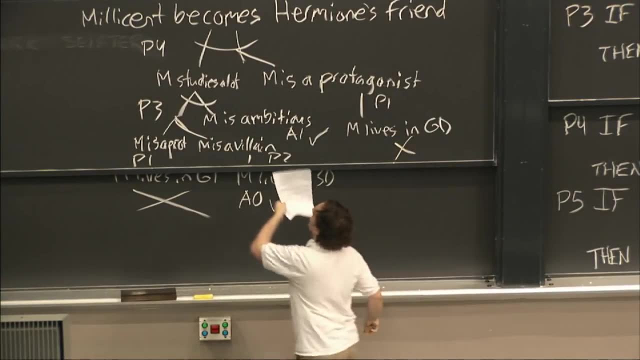 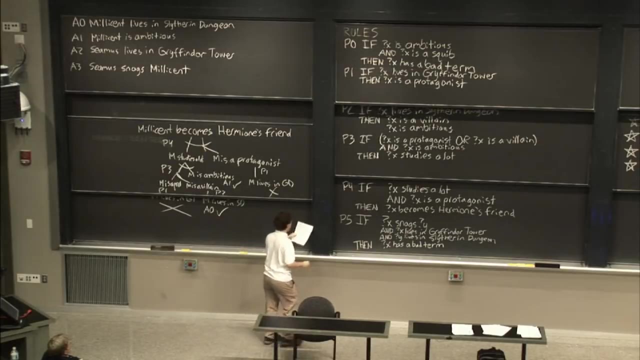 already tried. we try them again, damn it. and when we try it again, maybe it'll work this time. no, it never works. they're bitter enemies. Millicent does not become Hermione's friend, so now they ask us a few questions, which are pretty easy to answer. 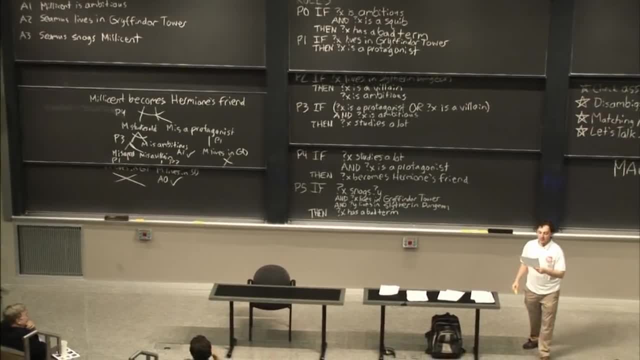 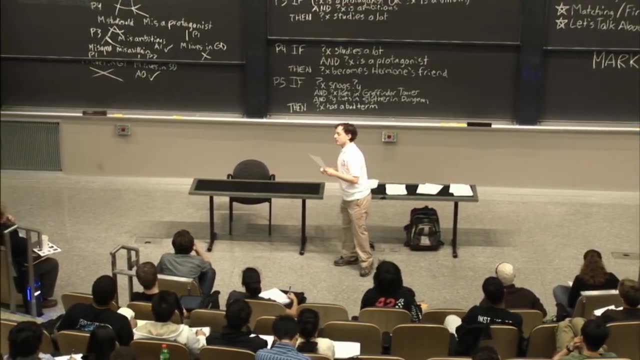 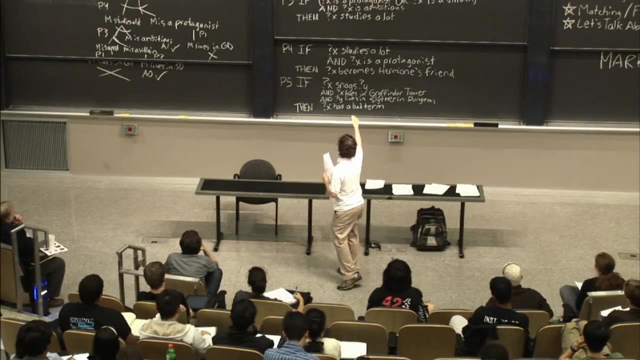 based on the ordeal we've just been through. so determine the minimum number of additional assertions that we would need to add for Millicent to become Hermione's friend, but you're not allowed to add an assertion that matches a consequence of a rule. you can only 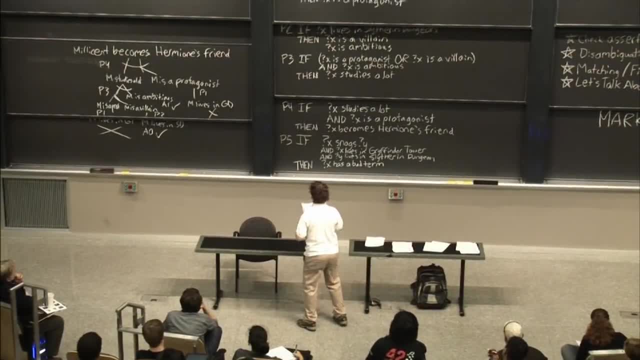 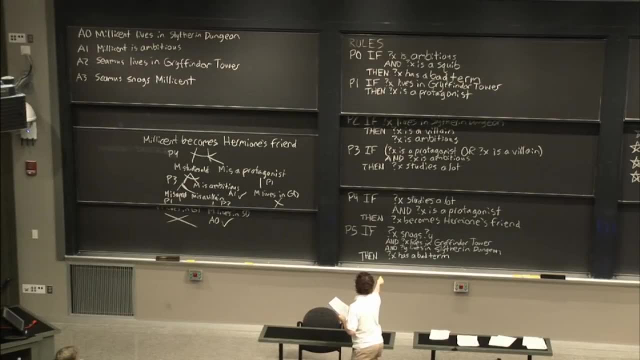 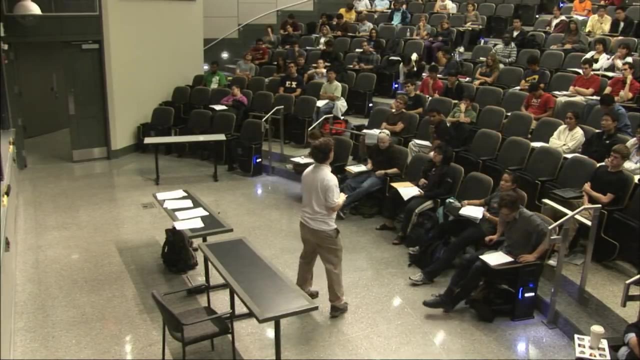 add an assertion. in other words, you can't add an assertion that will prove some other rules. you have to add an assertion that directly. that's basically the rule here, because there's a lot of choices, but he wanted one particular answer, so can anyone think of an? 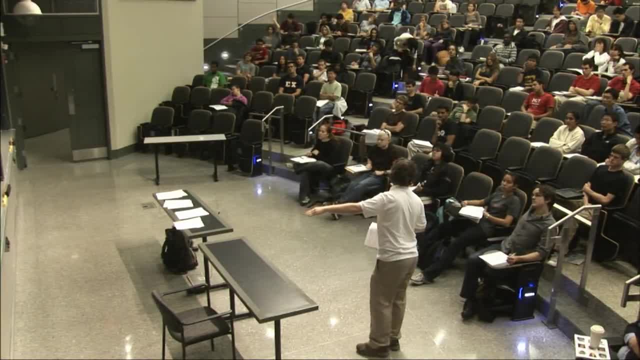 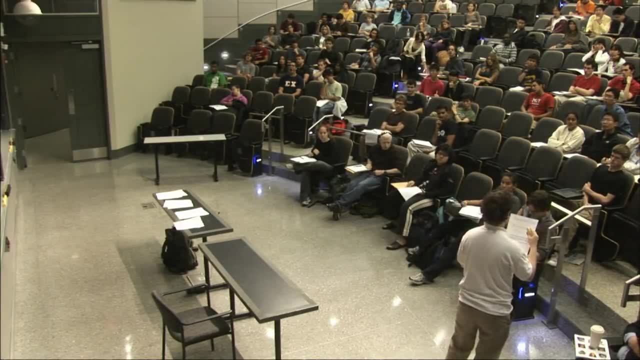 assertion that doesn't match any consequence of any rule that will make her be Hermione's friend. a lot of people say Millicent lives in Gryffindor. that's correct. so part three: your solution to part two- causes an uncommon situation. what is the uncommon? 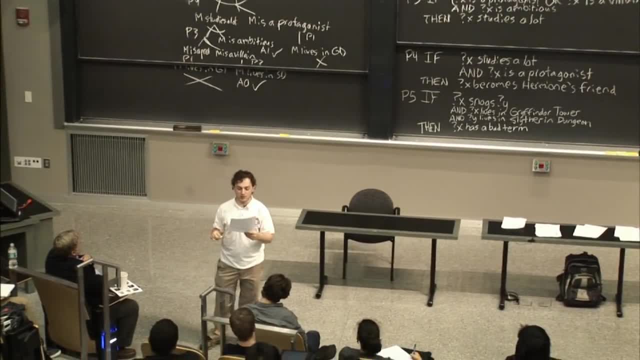 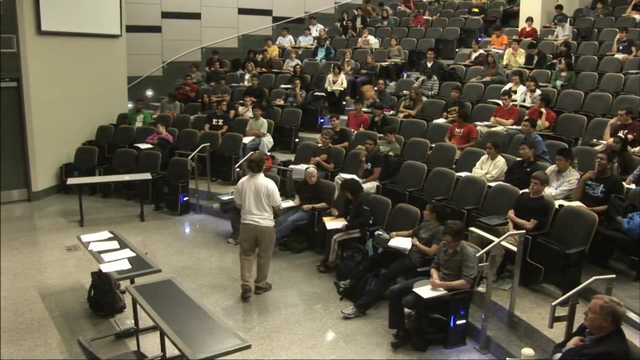 situation and what should you do to the list of assertions to solve this problem? does anyone know what the uncommon situation would be if we added that she lives in Gryffindor? hand is raised up here. what is your answer? that's true, she lives in Gryffindor. 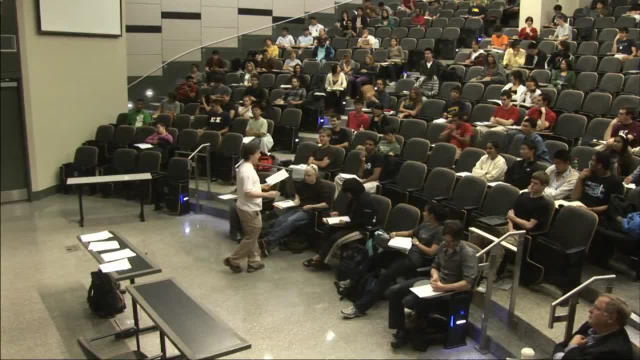 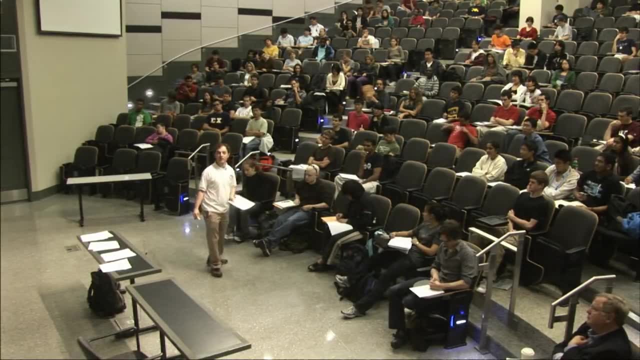 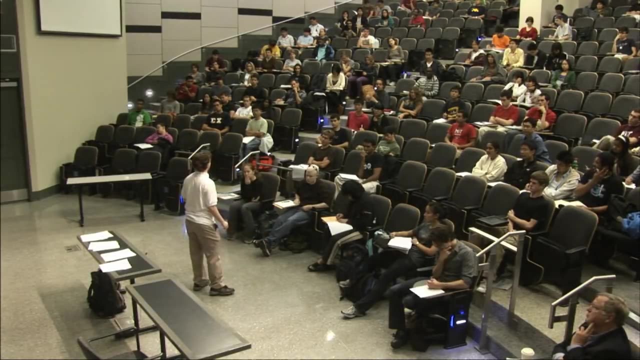 and Slytherin. so how would you fix that? yes, you can pick out. take out Slytherin from the assertions and say that she only lived in Gryffindor. a lot of people gave the answer to this question, which is a perfectly reasonable thing to. 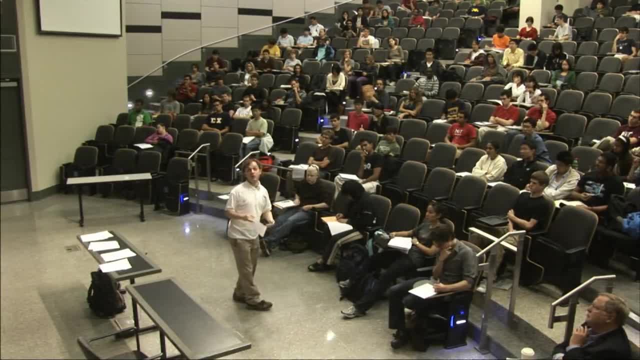 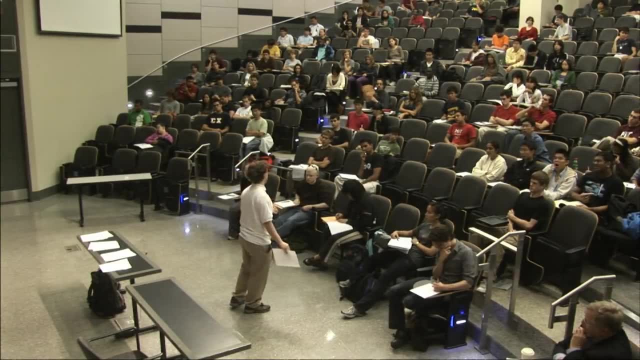 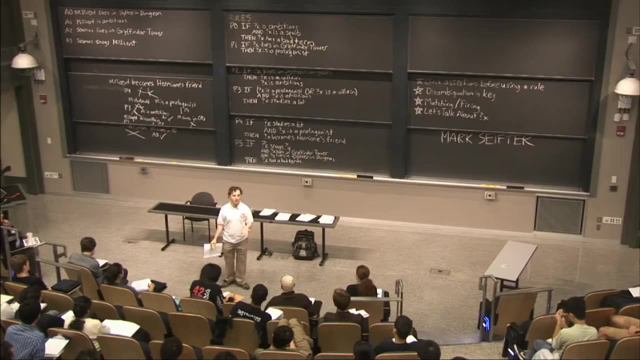 do in a rules based system. they said: well, we can add a rule that says that if you live in X and Y is different than X, then you can't with that. among other things is that we asked for a way to change the assertions and not the. 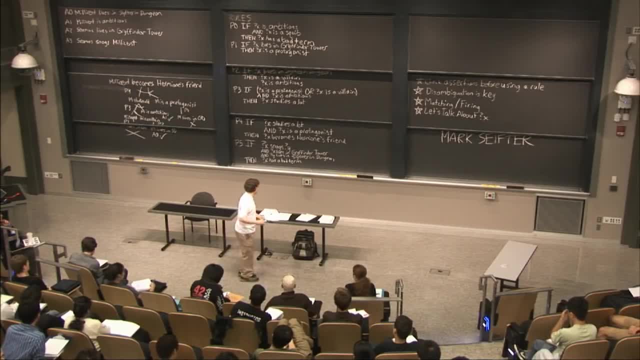 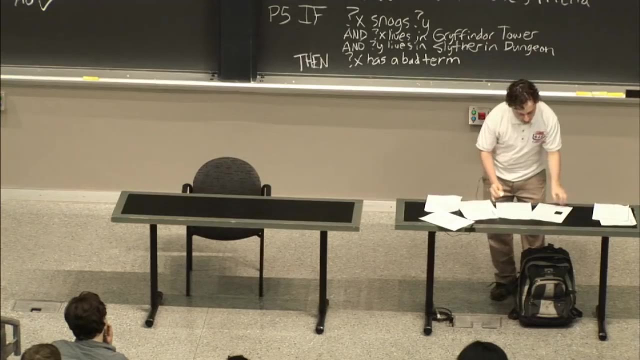 rules and you gave us a way to change the assertions. that's the right answer, great. so there was another backward chaining problem. this is 2009 quiz one, and I will leave it off for the moment. you guys should take a look at it, in particular, with: 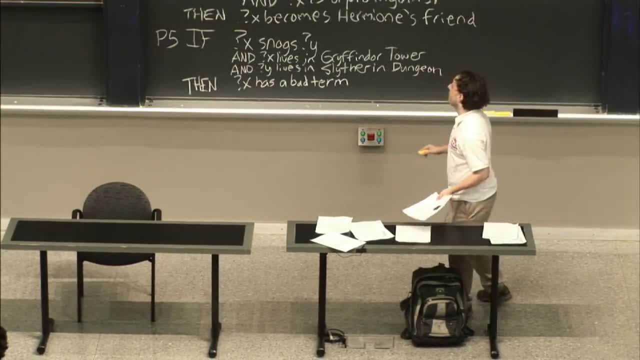 variable binding, because remember that you always have to bind the variable that's relevant to you, but that doesn't mean that you always have to bind all of the variables. for instance, let's say that we wanted to prove that Millicent has a bad term, which. 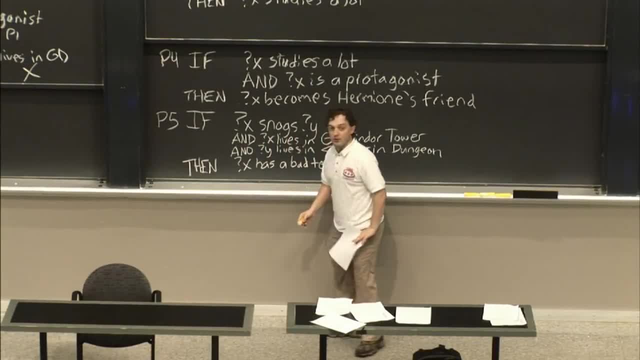 as it turns out, is what we want to prove in the other backward chaining. very quickly and without doing the problem, can anyone who thinks they're very clever at backward chaining tell me exactly what things would be added to the goal tree to prove that, Millicent? 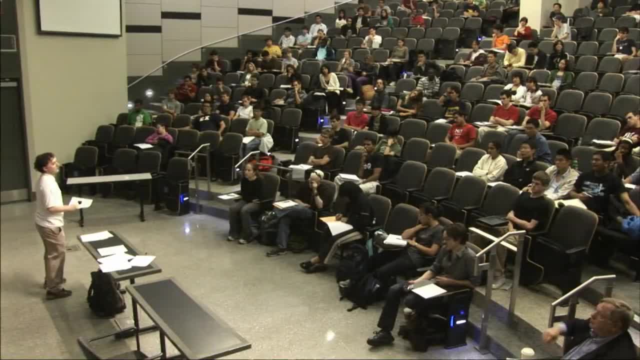 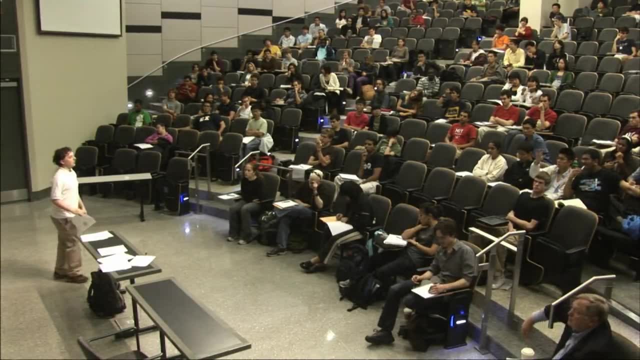 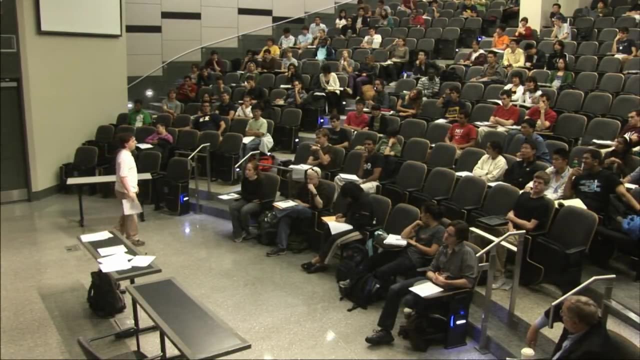 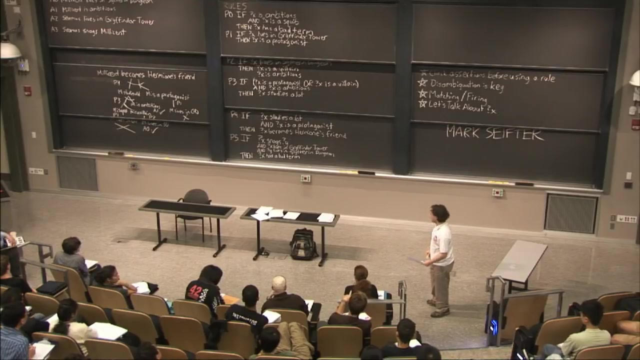 has a bad term. raise your hand. I won't pick out a victim because I'm asking this to happen pretty quickly. no one? all right, you would add the three to rule five specifically, so for anyone for variable y. so you just have to show that there's. 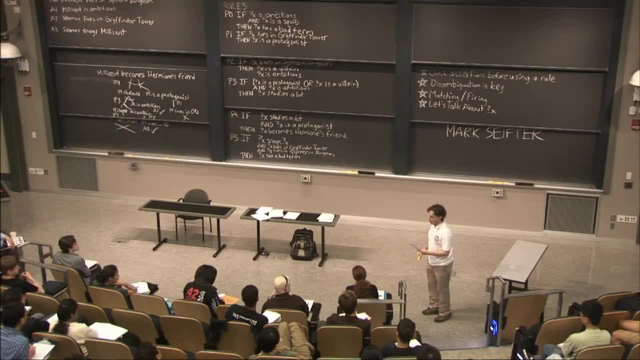 at least one person who matches. so can you just sort of read out: what would the first thing say with the snogs x, snogs anyone- yeah, Millicent. snogs y. that's crucial. some people did a lot of different things. some people put Seamus. 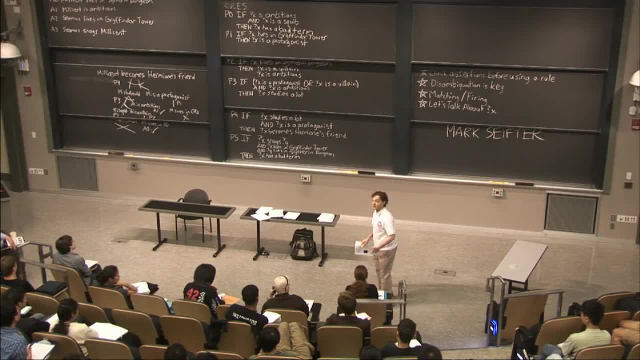 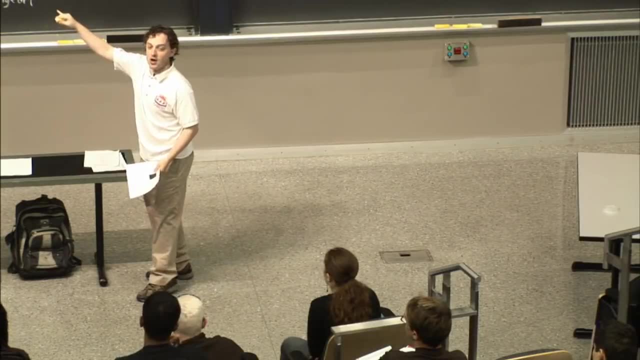 in already. you can't do that. the system is stupid. it doesn't know the person is Seamus. also, some people said it worked because, look, they're snogging each other. but it's the wrong snog old direction up there because we have Seamus. 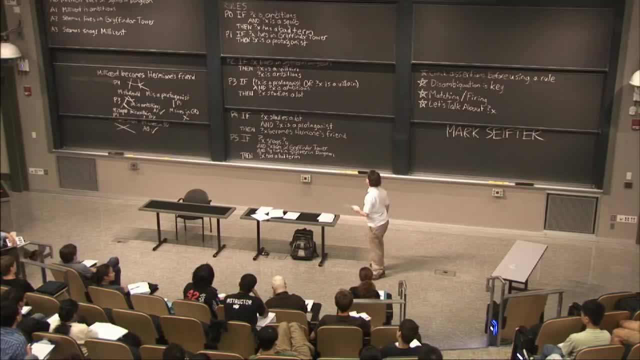 snogging Millicent, not Millicent snogging Seamus. but yes, exactly, it would be Millicent snogs y. Millicent lives in Gryffindor tower y lives in Slytherin dungeon. so let's give forward chaining all. 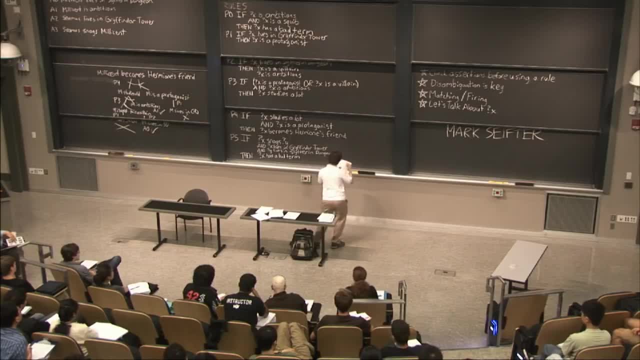 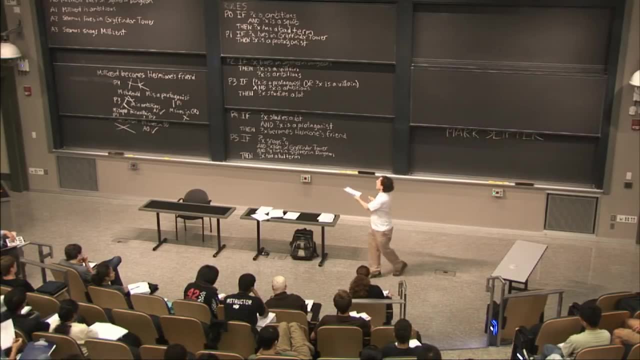 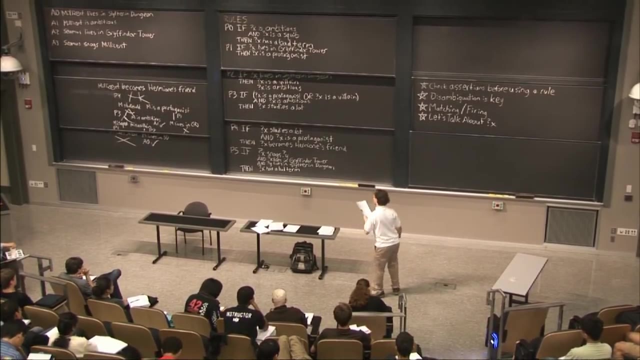 the attention it deserves: about eight minutes, which will be more than enough. okay, we still got all these rules, we still got all these assertions. instead of doing that horrible backward chaining- it's not that horrible, but we'll do forward chaining. it'll be really easy. we'll. 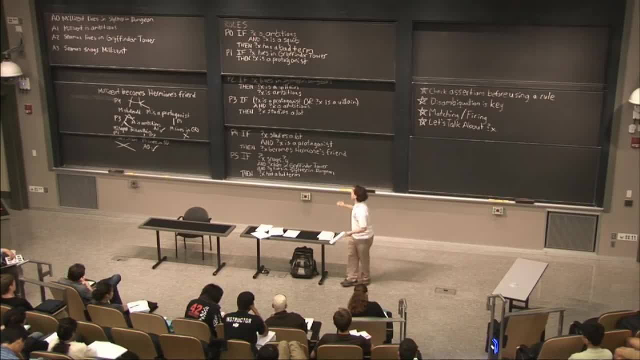 just add new assertions as they go. remember the tie break order rules in order from zero to five, and if the same rule could fire off with multiple different assertions, we'll use the assertions in order from zero to three. so let's see we don't have much. 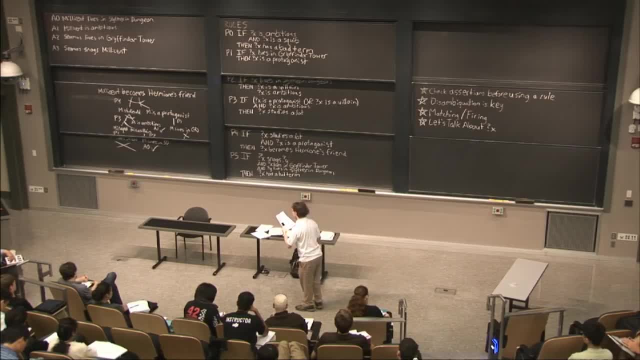 time, but with our four assertions. let's see what rules possibly could match with our four assertions. well, I'll figure out for you. do we have an assertion about an ambitious person? yes, but they're not a squib, so not rule zero. do we have someone who 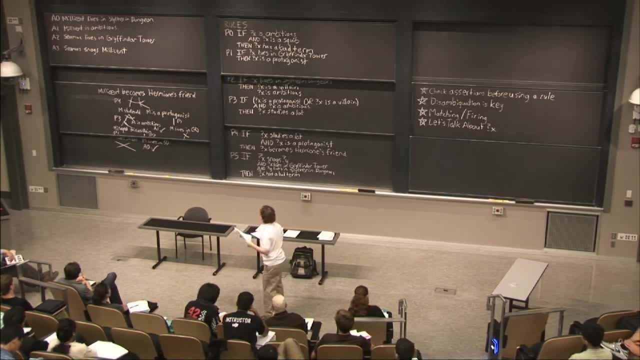 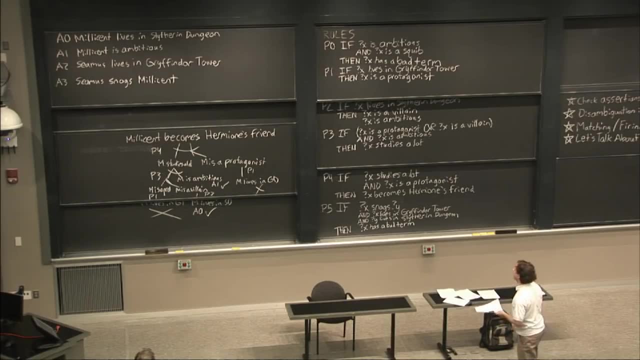 lives in Slytherin. we do rule two matches. do we have a protagonist or a villain? we don't have any protagonist or villain. rule three is not going to match because it's in an end. do we have someone who studies a lot? we do not have. 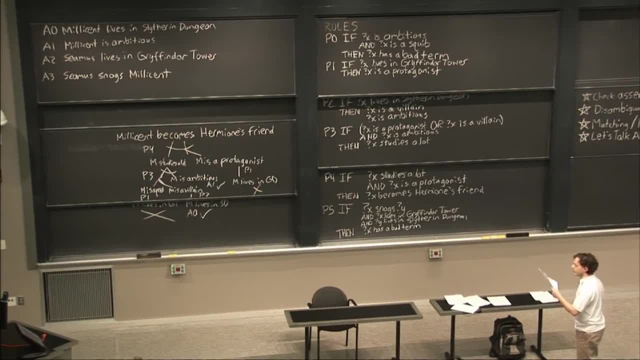 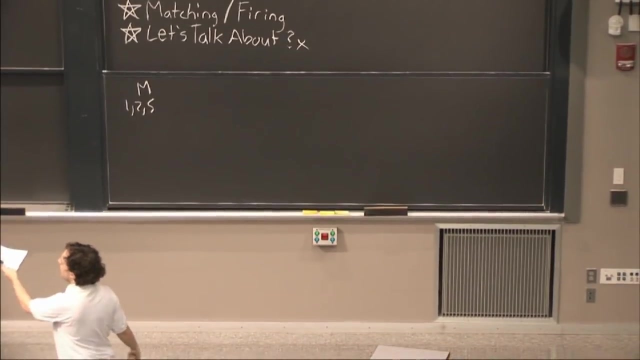 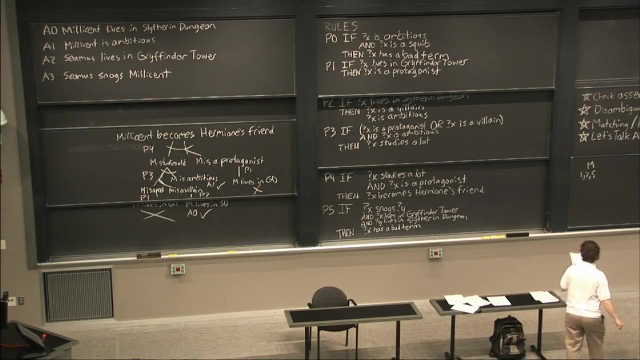 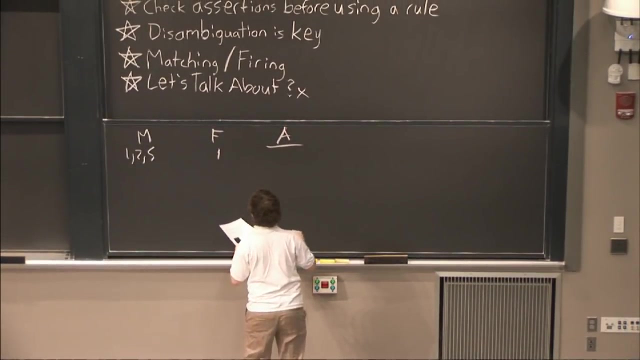 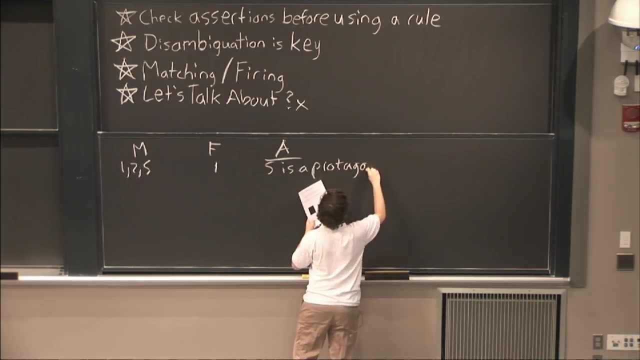 someone who studies a lot, rule four is not going to match. do we have some snogging? we do have some snogging, so rule one, two: which one is rule one? if x lives in Gryffindor Tower, the only binding for x is Seamus. Seamus lives in Gryffindor Tower. we're firing off rule one. so new assertions? the first assertion that we'll add is: Seamus is a protagonist. great. now there's one other thing, and it's the main thing I wanted to tell you about in forward chaining. 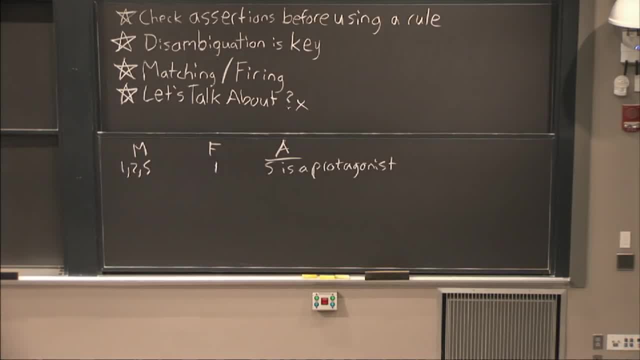 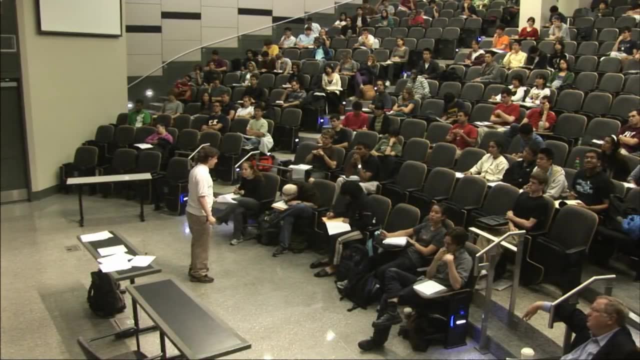 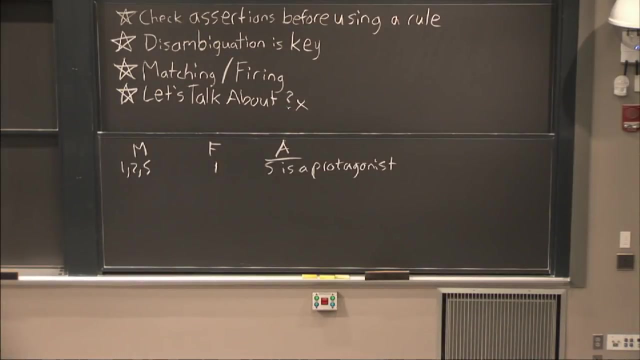 about our old friend, rule one. now that we've done this, does rule one still match an assertion in the database? yes, it does, but what's going to stop us from constantly doing rule one every time, because it comes numerically before the other rules? what stops us there is part of our implementation, and it's a very important part that people sometimes forget. 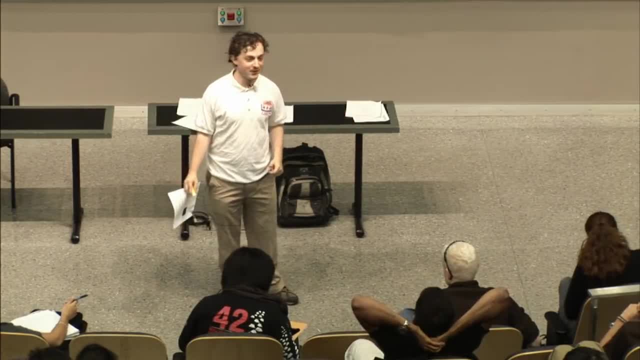 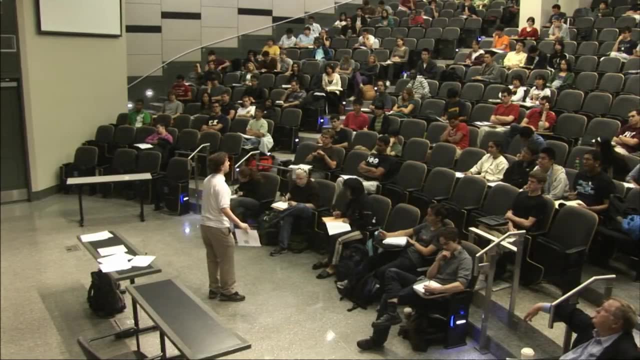 so what I like to call the no impotent rules implementation detail, that is, if a rule is completely, 100% impotent, it would do absolutely nothing, then you do not fire it, you go to the next one. that's pretty important. let's say that you. 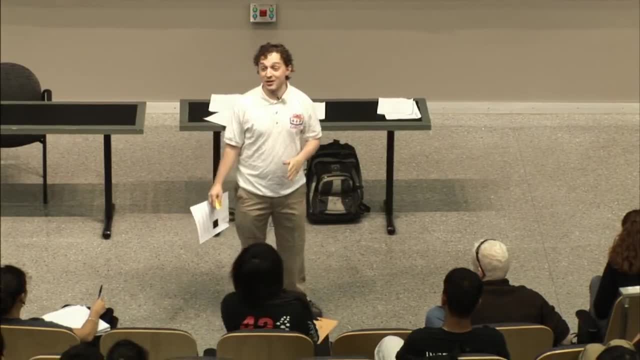 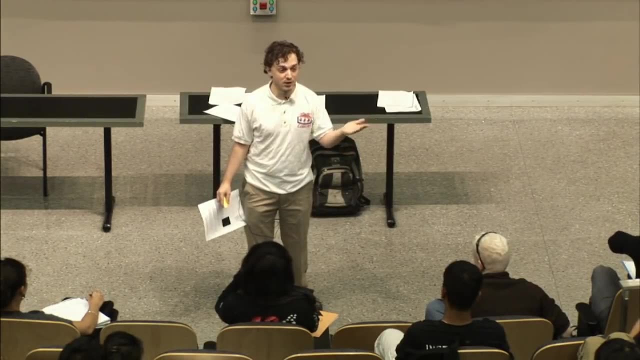 possibly had a delete which you won't have on the quiz. that means that if the thing to delete is missing, it's impotent. if the thing to delete is there, it's not impotent because you can delete. let's say, you have five hundred thousand things that you're going to add to your assertions. 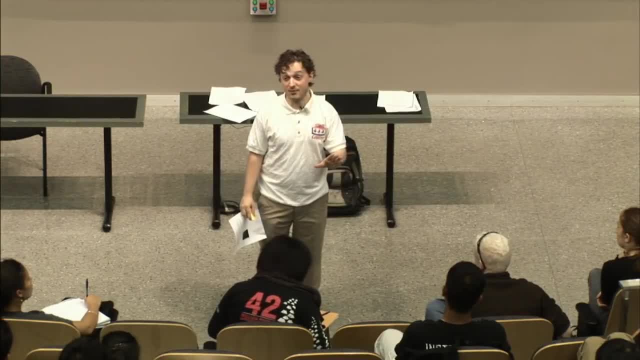 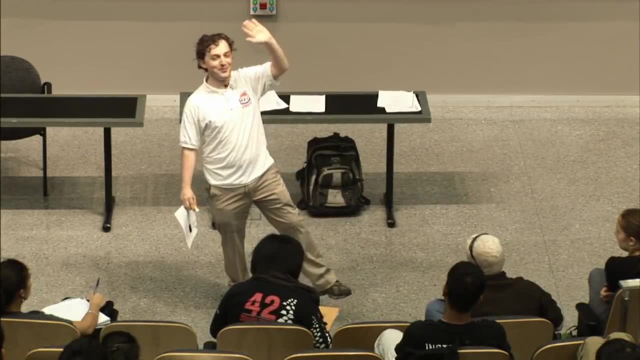 four hundred ninety-nine thousand nine hundred ninety-nine are already in your database. one of them is missing. Is it an impotent rule? No, it's not. You have to fire it anyway. You can't be like: oh, it's mostly an impotent rule. 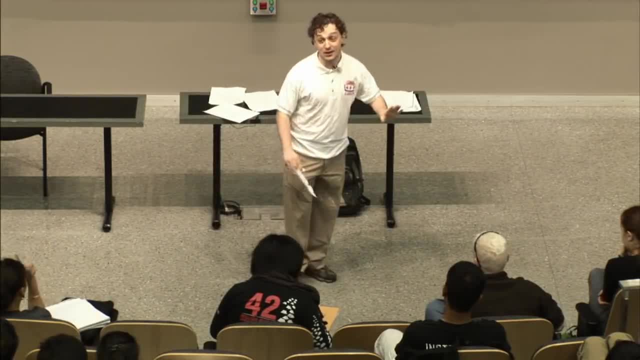 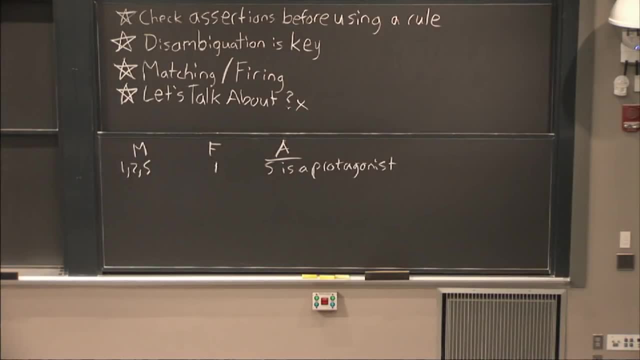 No, you have to fire off the rule if it will do anything. But right now, rule one won't do anything because we've already added Seamus as the protagonist. So what rules match now? Well, Seamus becoming a protagonist is nice and all. 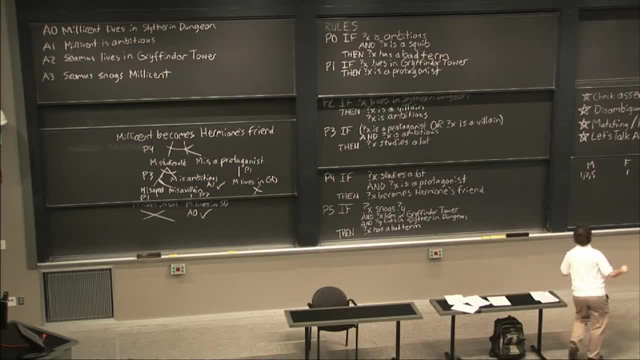 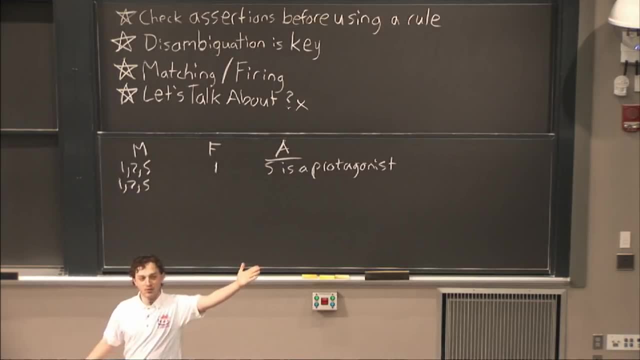 but he's not ambitious. so we still don't match rule three. We still match rules one, two and five. As I basically just got finished telling you, the one that we're going to fire off now is two, That's right. 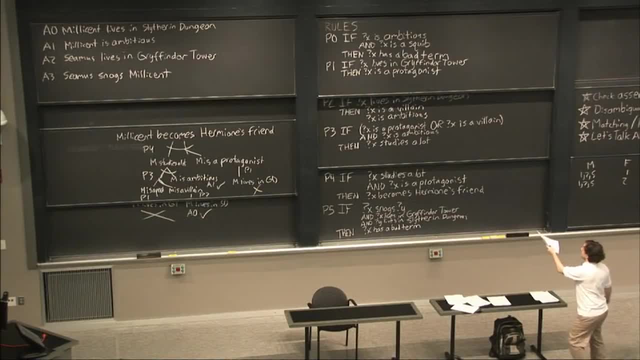 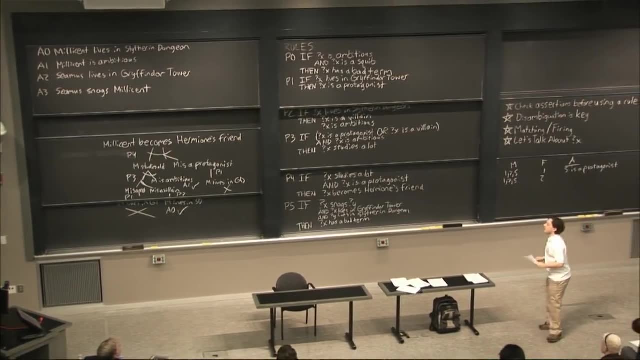 So rule two is: if Exil is in Slytherin dungeon, our only binding for that is Millicent, and that will show that she's a villain and she's ambitious. So what assertions will we add? Millicent is a villain and people stopped. 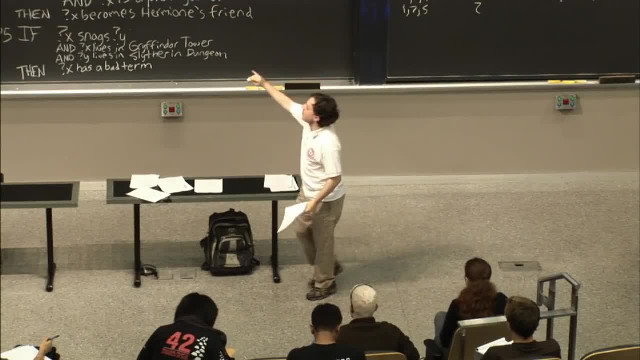 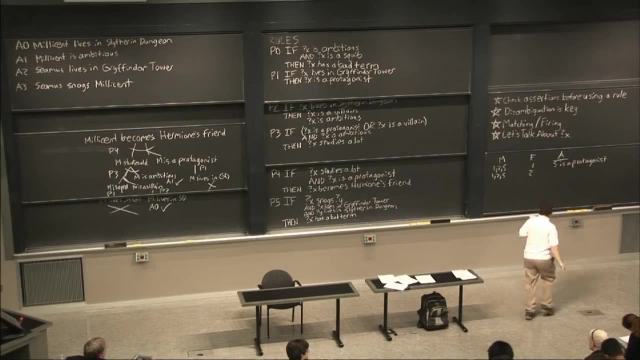 That's right. Good job everyone. You remember that Millicent is already ambitious from assertion one, so we don't have to add them both. A lot of people did. They were wrong, So Millicent is a villain. The other part of that rule doesn't do anything. 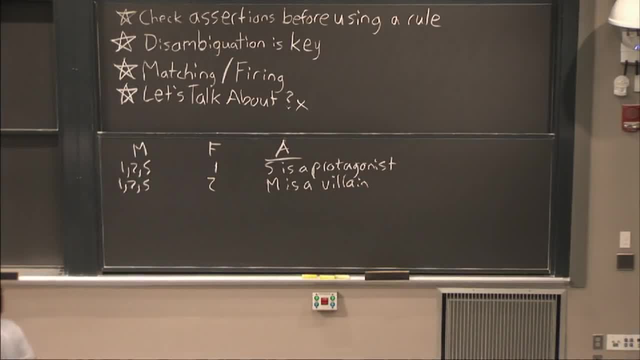 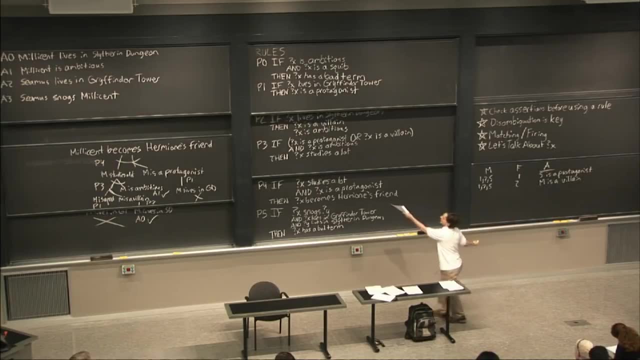 but it's not an impotent rule, because one of the things is not on there, Great. So what rules match now? Well, as it turns out, now that Millicent is a villain and ambitious, we've matched rule three as well. 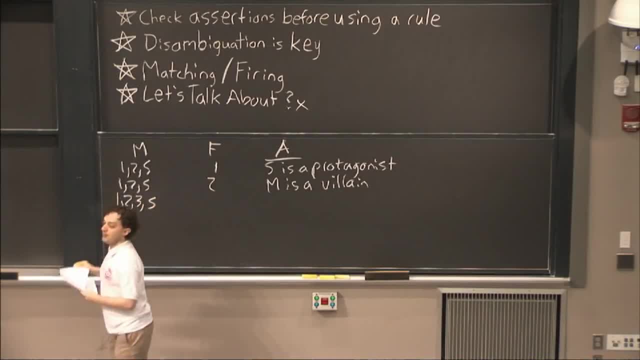 So we match one, two, three and five. What rule are we going to fire everyone? Three, Three, Three. because one and two are impotent rules, We'll fire rule three. Well, Millicent is a villain. 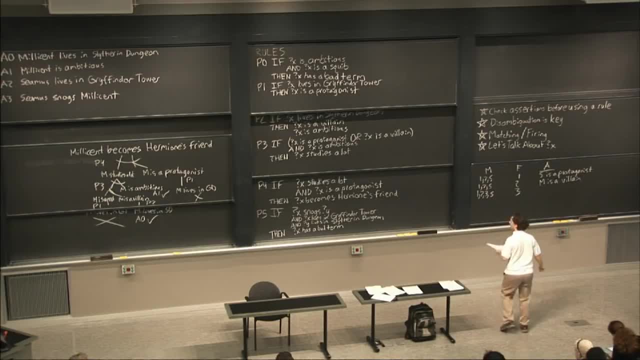 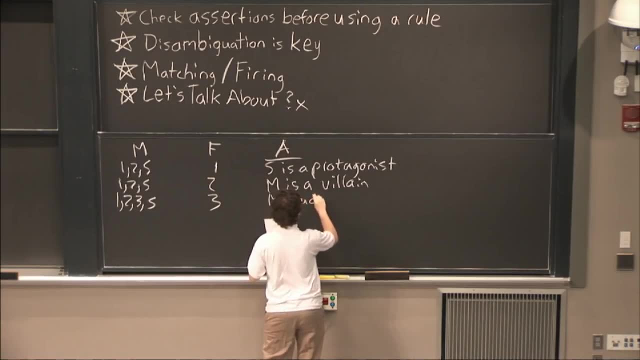 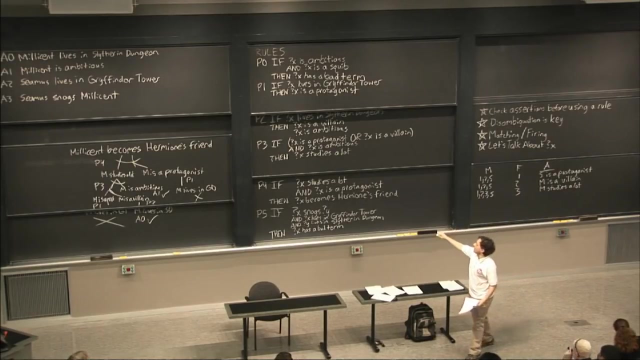 She's also ambitious. She's our only match for three. Therefore, what assertion do we add? Millicent studies a lot, That's right, Great. So Millicent studies a lot. However, she's not a protagonist. We still don't match rule four. 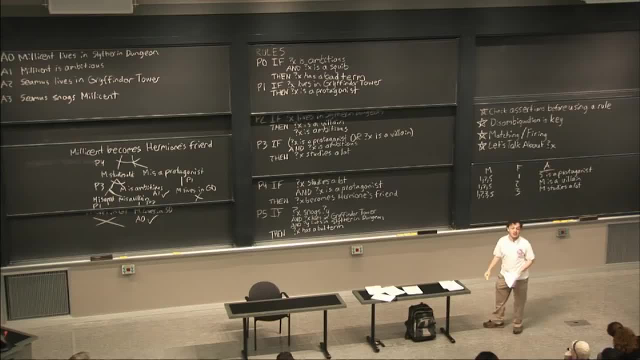 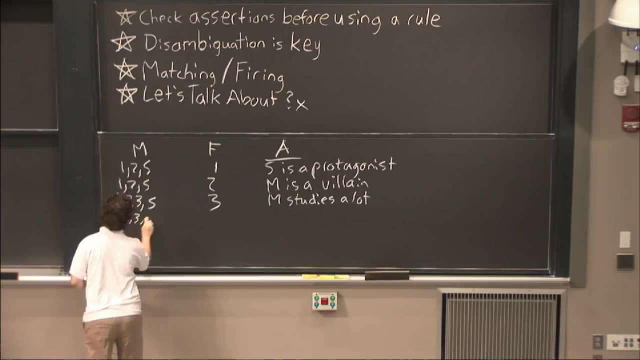 Oh well. Well, we figured that out already. We figured that out ourselves from backward, chaining that we were never going to match that. So what matches? It's still one, two, three and five, Seeing as one, two and three are impotent. 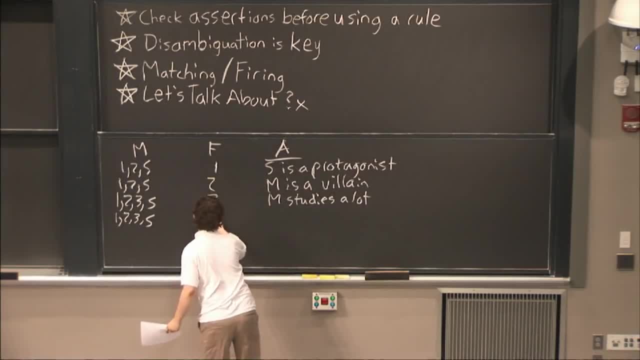 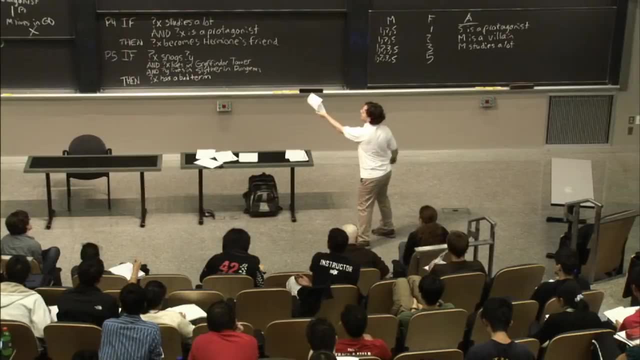 the only match is five, And so the only match we care about, the only one we're going to fire is five. And the result? let's see: X, snogs, Y, that's Seamus. snogs Millicent X lives in Gryffindor, that's Seamus. 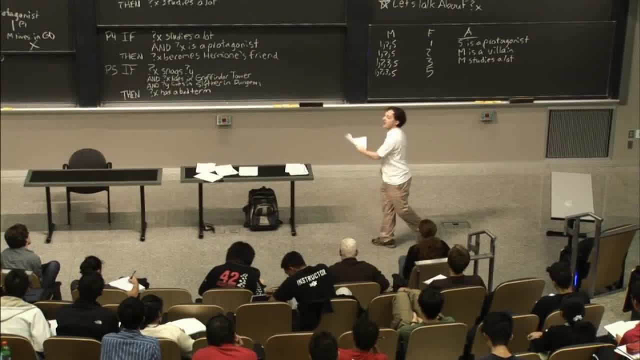 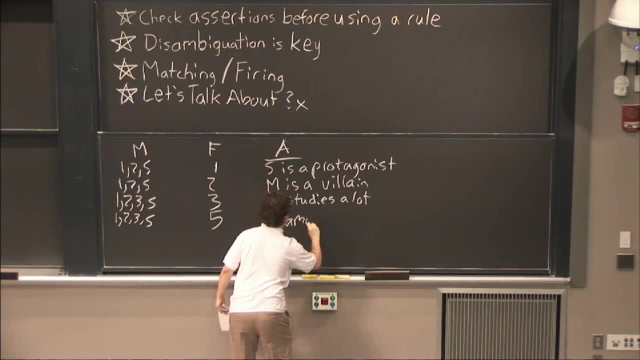 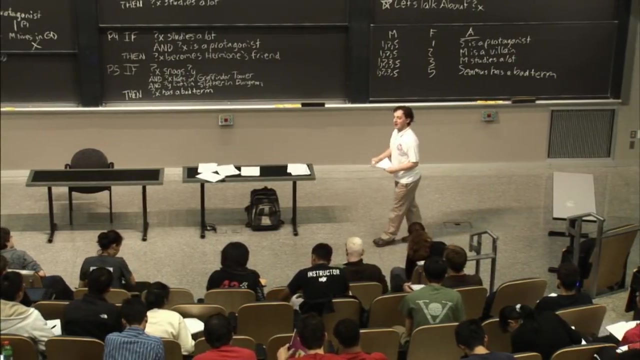 Y lives in Slytherin, that's Millicent. So what do we add? Seamus has a bad term: Simple, painless, It works out. We're done and we got 100 on this quiz. Hopefully you guys will too. 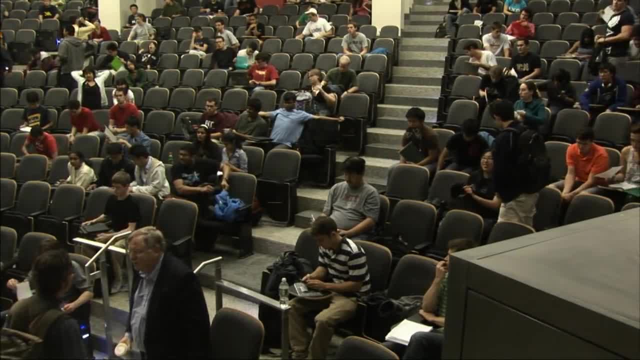 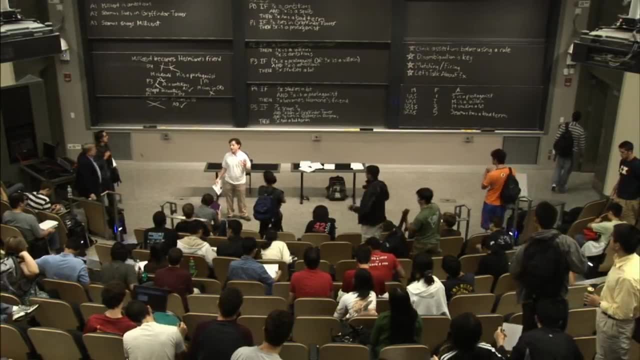 Question. The question is if you have a new assertion which matches a rule, but it's really high number, it's all the way down at the bottom of the rules. but it's new and it has new stuff. Should we do that first, maybe because it's new? 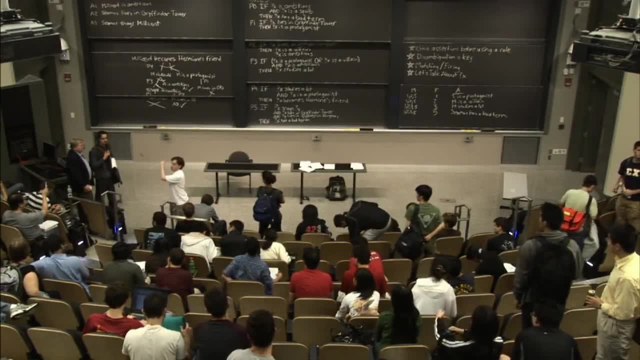 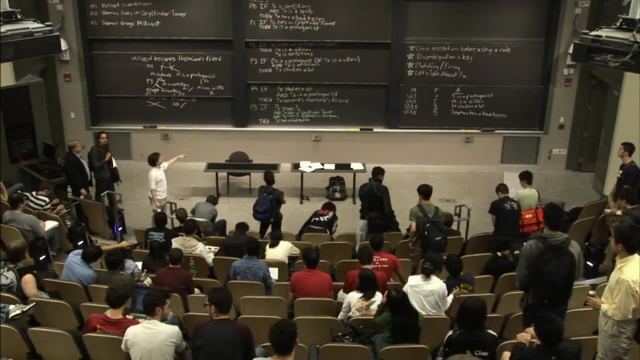 Oh, you mean that it has a lower number, a lower number, Okay. So the question is: if a rule- let's say that rule three- made Millicent be a squib, Then yes, you'd immediately not only match zero with 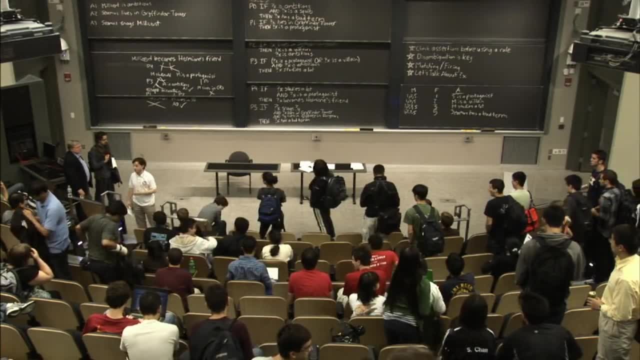 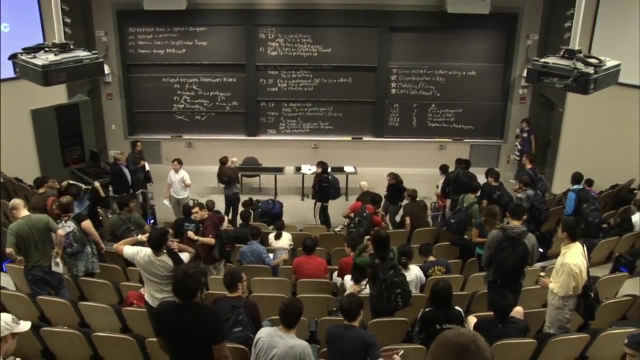 zero would immediately fire because it's numerically it comes first. You'll see that on some of the other old quizzes and you may see that in tutorial. If you guys want to do some more practice problems in tutorials, your TAs will have that available as one opportunity in tutorial.